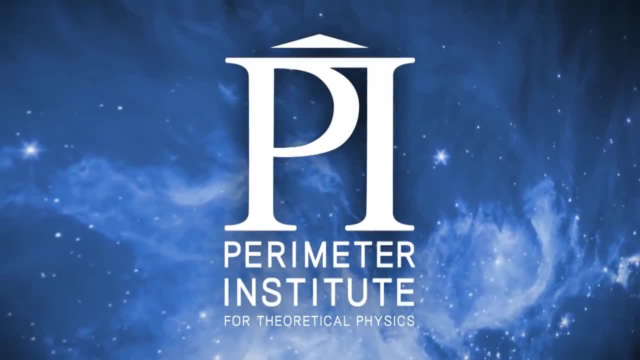 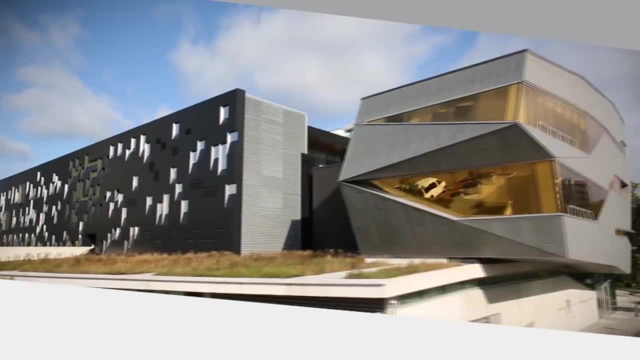 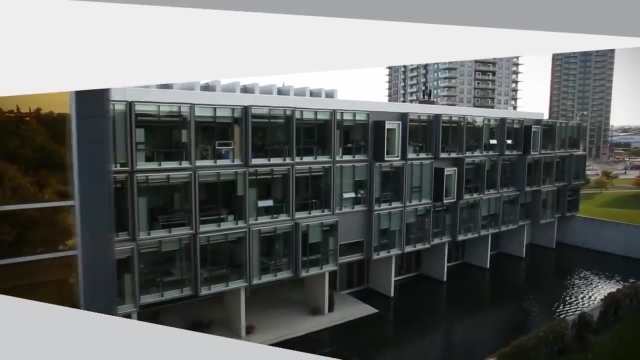 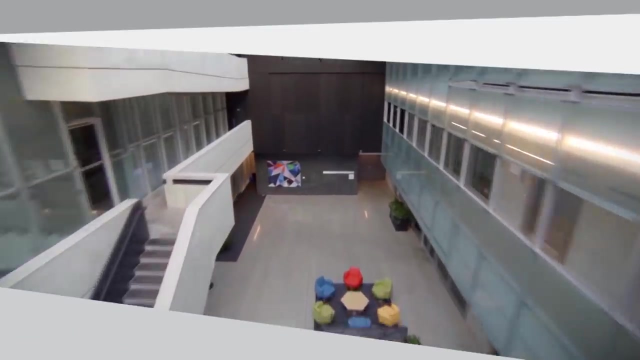 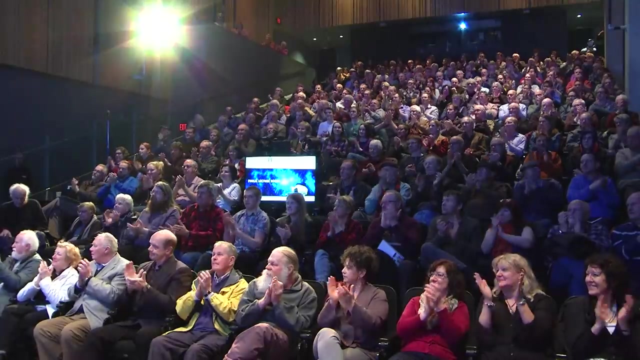 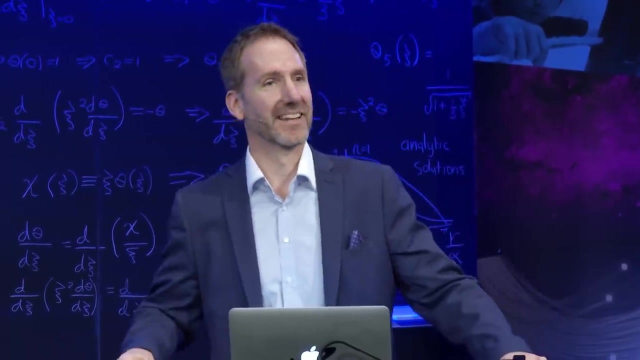 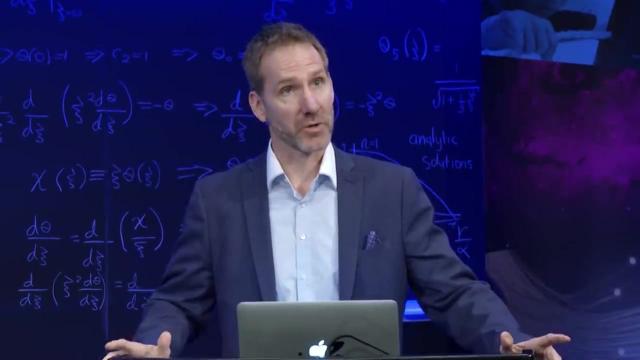 Thank you very much. Hello, Thank you, Welcome, Welcome. Welcome to Perimeter Institute and welcome to Perimeter Institute's public lecture series. For those of you that don't know, Perimeter is located in Waterloo, Ontario, Canada. My name is Greg Dick. I'm the Director of Educational Outreach. 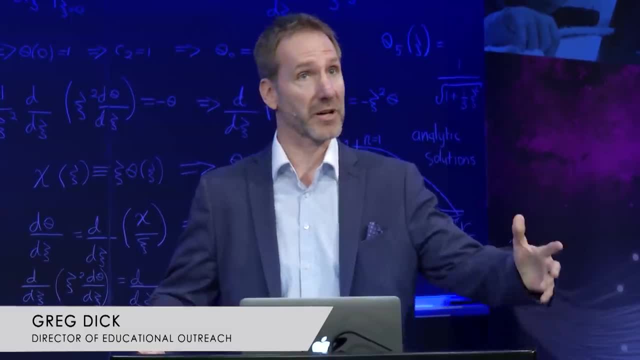 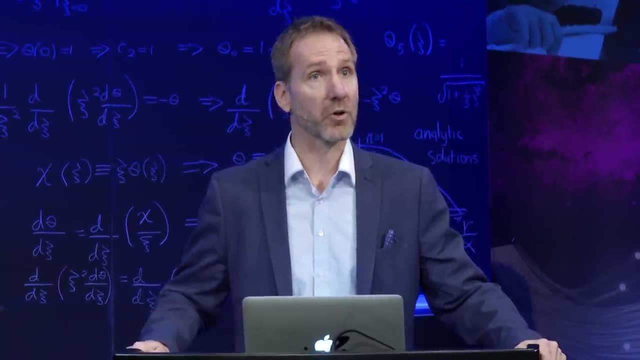 and it is a pleasure to welcome everyone here this evening, both those of you here in the live studio audience and those of you watching online. The lecture itself will last approximately one hour and will be followed by a question and answer session. For those of you that. 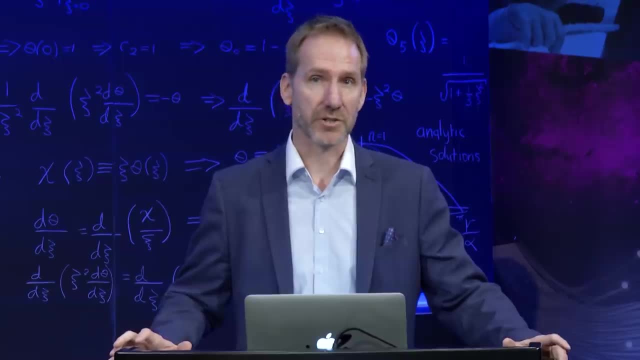 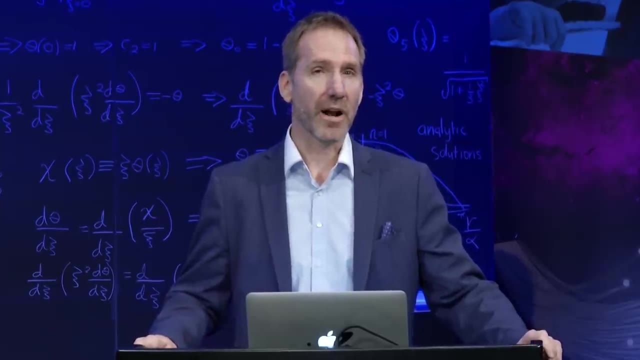 are watching online. Dr Kelly Foyle and a team of PI researchers are behind their keyboard, ready to engage in conversation and answer questions throughout the lecture And, if you want to ask a question both during the lecture that way, or ask a question to our guest speaker. 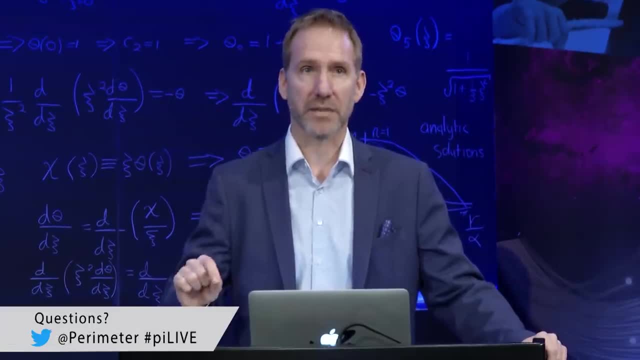 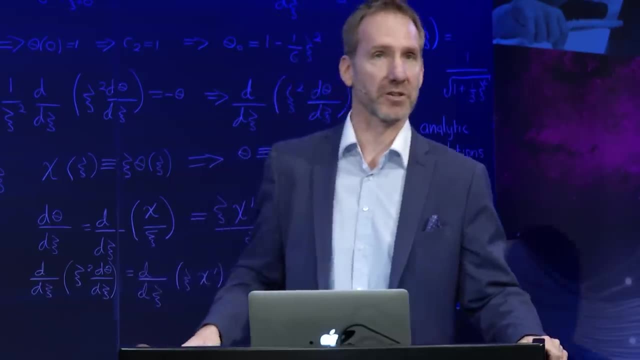 use hashtag PILive And if you have a question for the guest speaker, get it in. All right, And now it's time to introduce tonight's very special guest speaker, Dr Emily Levesque. Dr Levesque is an Assistant Professor of Astronomy at the University of 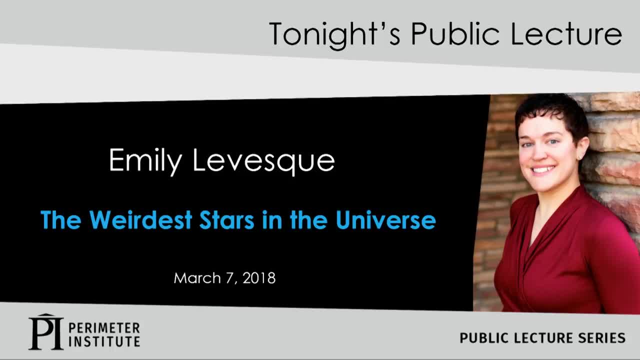 Washington. in Seattle, She received her Bachelor's Degree in Physics from MIT and completed her PhD in Astronomy at the University of Hawaii and was both an Einstein and a Hubble Postdoctoral Fellow at the University of Colorado. Emily is a rising star in astronomy and a professor. 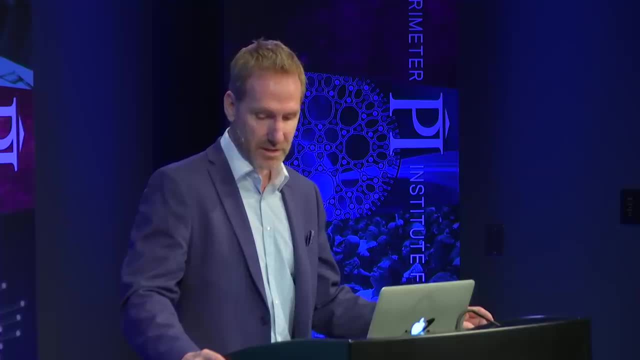 at MIT. Her accolades include a 2017 Alfred P Sloan Fellowship and a 2014 Ann Jump Cannon Research Prize from the American Astronomical Society. Dr Levesque's research focus is on massive stellar astrophysics and the use of massive stars as cosmological tools. Tonight. 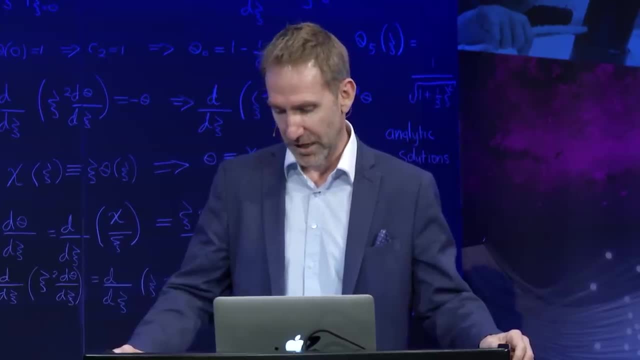 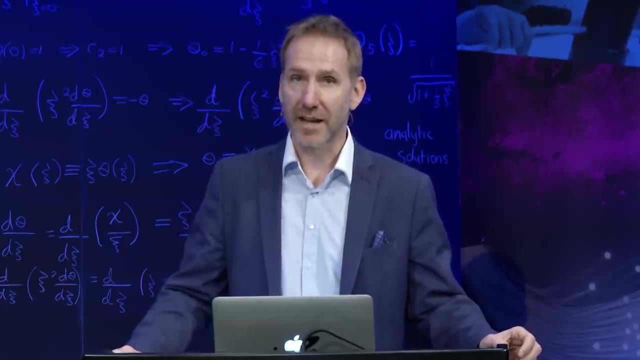 she will discuss some of the strangest stellar phenomena in our universe and how these weird stars serve as a common thread for exploring the universe. We're exploring our universe's history, evolution and extremes. Ladies and gentlemen, please welcome Dr Emily Levesque. 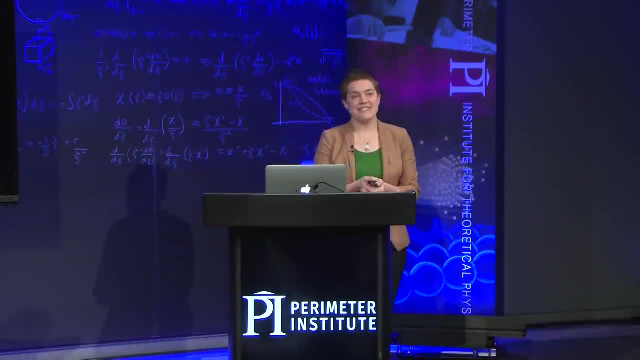 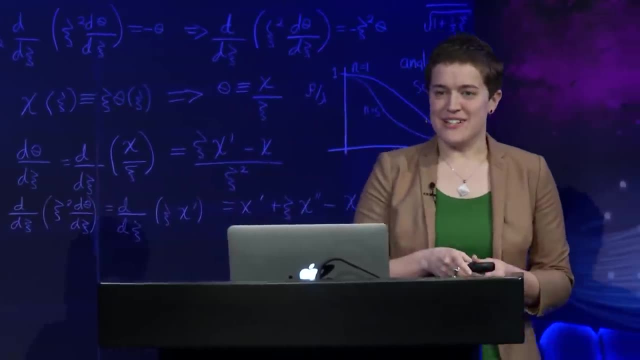 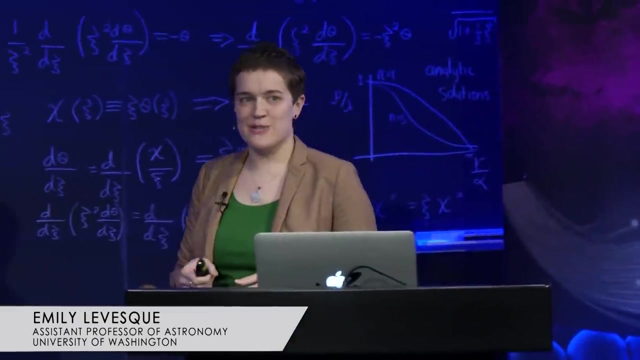 Well, hello and welcome to tonight's lecture. I'm extremely excited to be here and so happy to be sharing these very weird stars with all of you. I always like to start by putting up some pictures of some of the weirdest stars in the universe, So every object that you see on the screen right now represents some sort 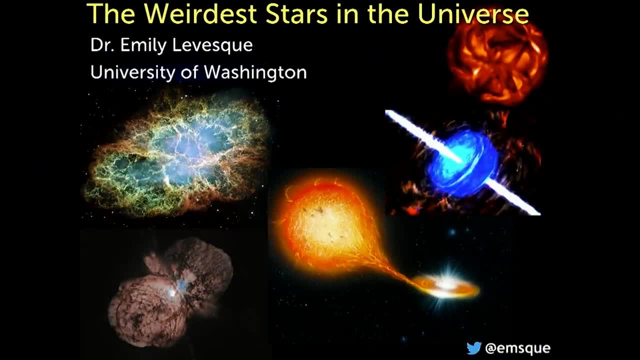 of bizarre or unexplained or particularly puzzling type of star, something that has surprised or confused, at times, astronomers. As I go through the talk and I look at things that are particularly weird or surprising, I'll be marking them with these little exclamation. 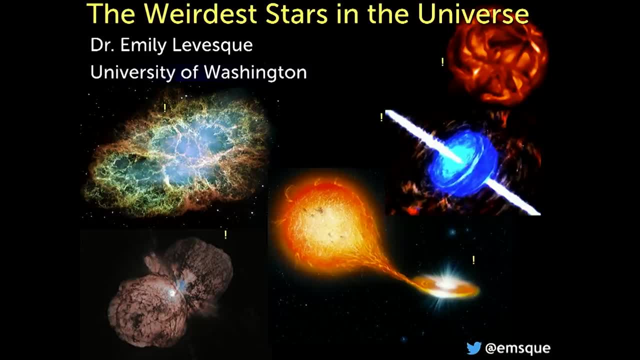 points. I can also promise you that by the time we get to the end of this talk, you'll be able to name every single thing on this screen. You'll be able to explain what it is, at least as well as astronomers can explain them, and you'll recognize all of them, if you ever happen. 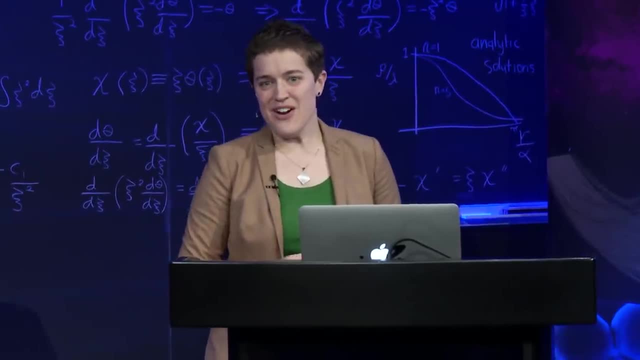 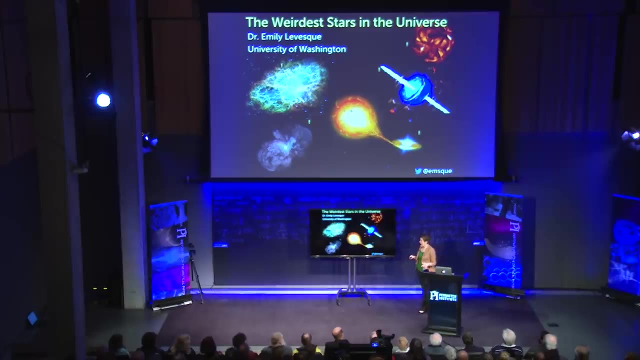 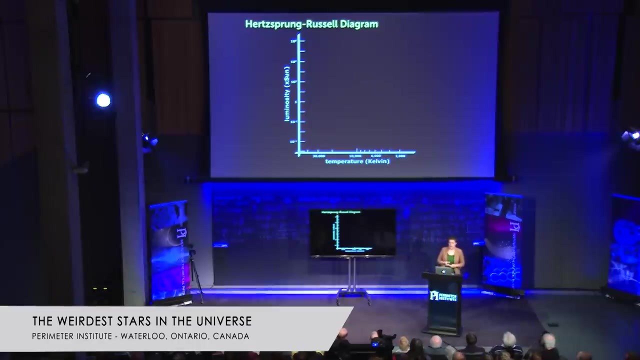 to come across them again. So to start off talking about weird stars, we need to establish what is considered normal for an object like a star, And to do that I actually need to start with a diagram. So this is a very common diagram used in astronomy. It's called the Hertzsprung-Russell diagram. What we're 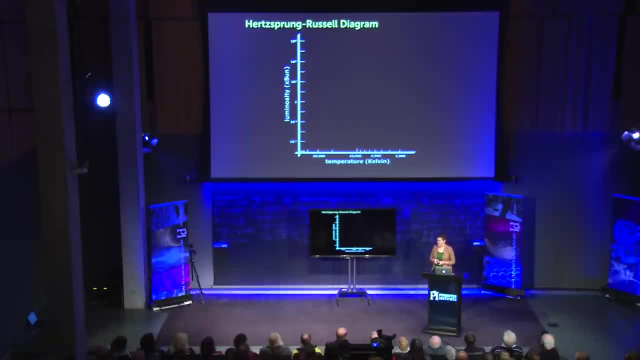 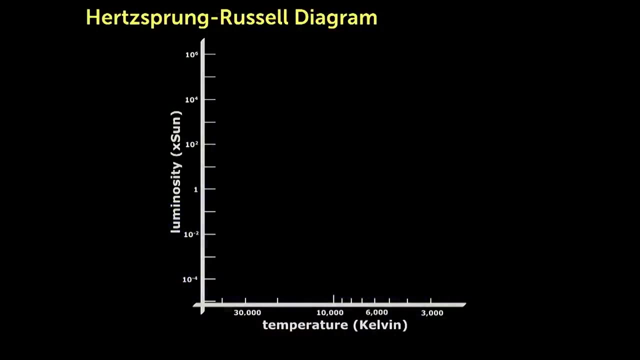 doing here is plotting temperature on the x-axis going from very hot on the left to very cold on the right, and plotting brightness on the y-axis going from dim at the bottom to very bright at the top. What we can do with this is drop the collection of normal. 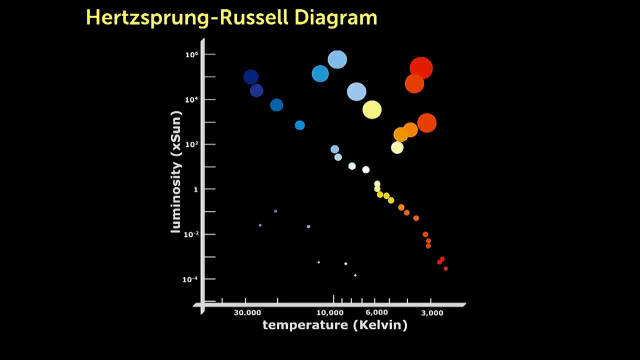 stars that we know about onto the diagram and see where they land. You can kind of see that there are clear spots where normal stars tend to hang out. I'll fill this in with a slightly more detailed version of the illustration and you may recognize the names of some of. 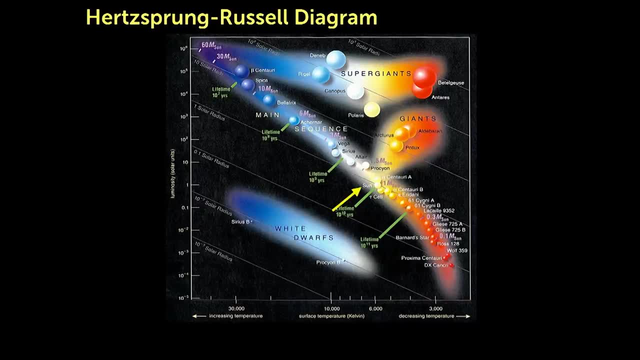 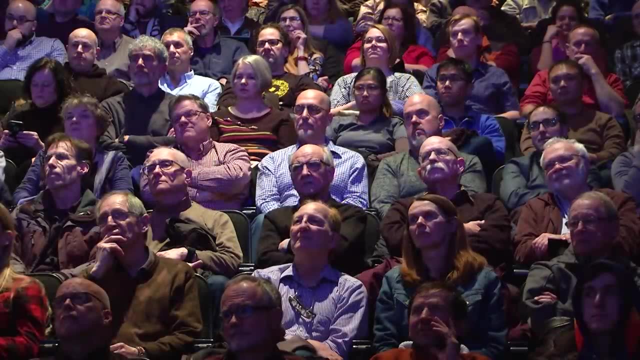 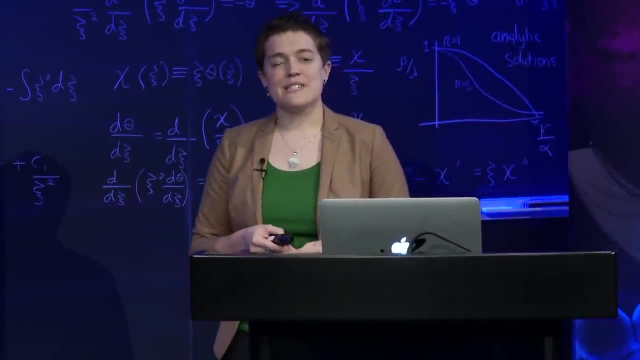 the stars on the plot, I always like to point out where our sun is. Our sun is right in the thick of things, and our sun is really a kind of depressingly normal and unremarkable type of star. The main thing that we use this diagram for in astronomy is explaining how stars evolve. This is something a lot of people don't necessarily realize stars do. They are born, they age and evolve with time and change, and then eventually they die. You can plot out how a star is going to live and die by following its path on the Hertzsprung-Russell diagram. 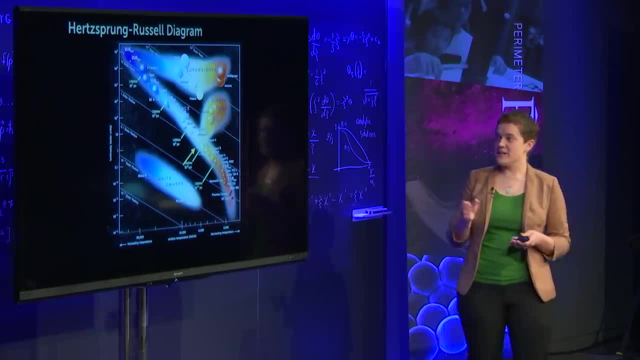 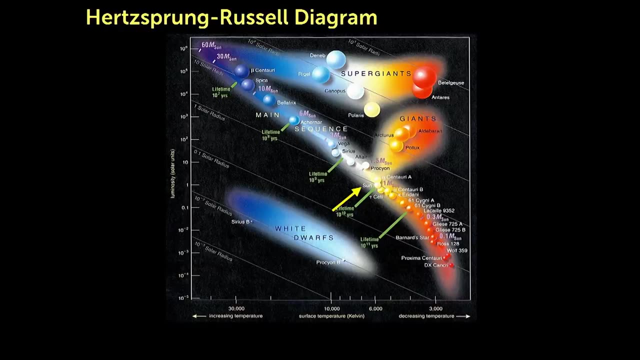 over the course of its life. You can see the sun. You can see that sort of diagonal of very normal looking stars. The stars that I'm interested in and the weird stars that we'll be focusing on tonight are at the very top of this diagram. 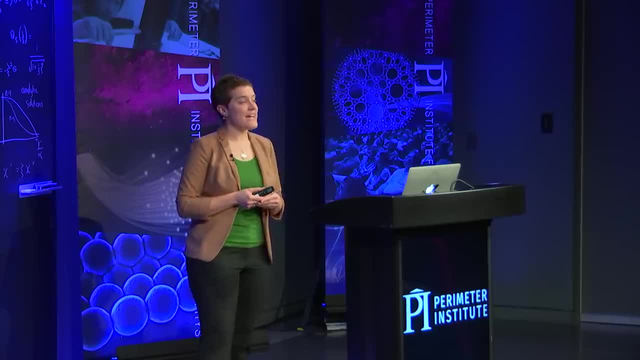 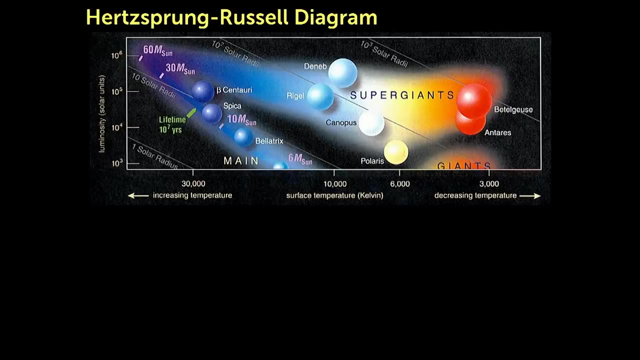 diagram. So these are the supergiants. These are massive stars. They're stars that are at least eight times the mass of our sun or more, And I want to start by taking a short tour through these stars on the Hertzsprung-Russell diagram and looking at how they evolve. I 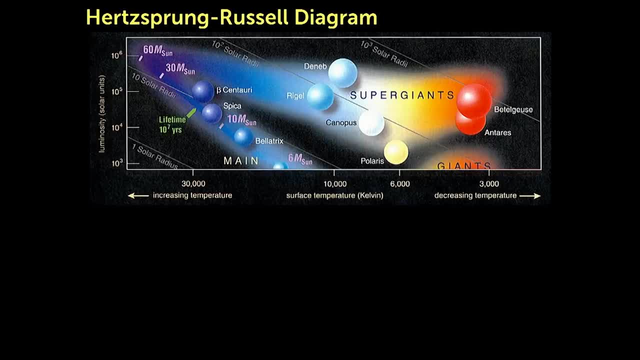 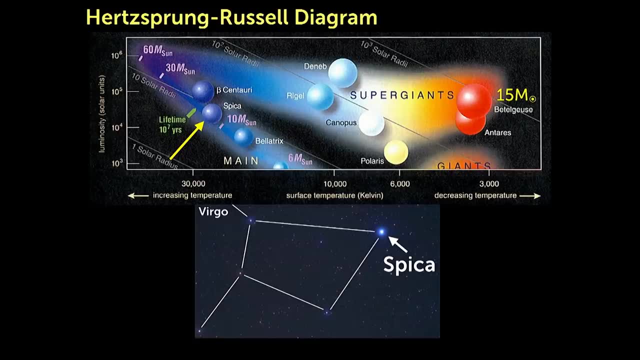 like to use examples of stars that you can find in your own night sky. So to begin with, I want to look at Spica. Spica is a star in the constellation Virgo. It's an amazing example of a blue supergiant. So this is a massive star in the first phase of its life. It's. 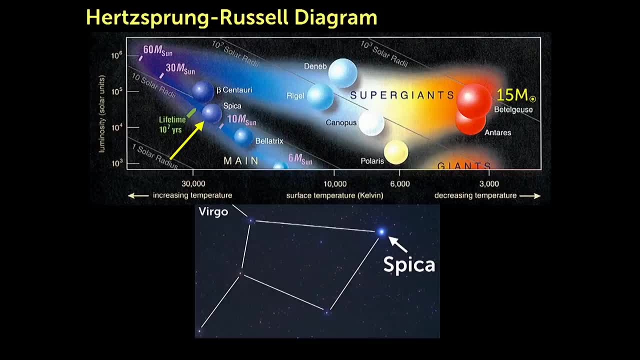 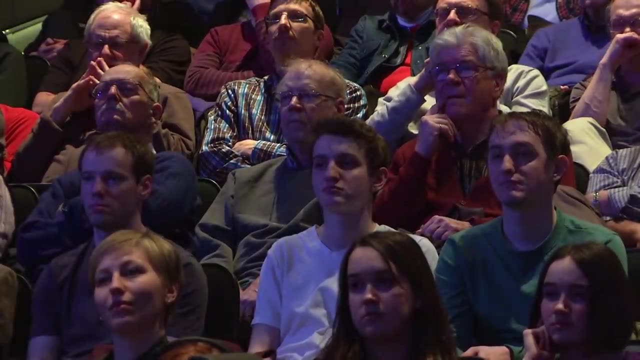 fusing hydrogen into helium in its core. It's very hot. It's about 22,000 degrees Celsius. That's much hotter than our sun. Our sun is 5,500 degrees Celsius. It's about seven times the mass of our sun. and it's about 10 times the mass of our sun and about seven times 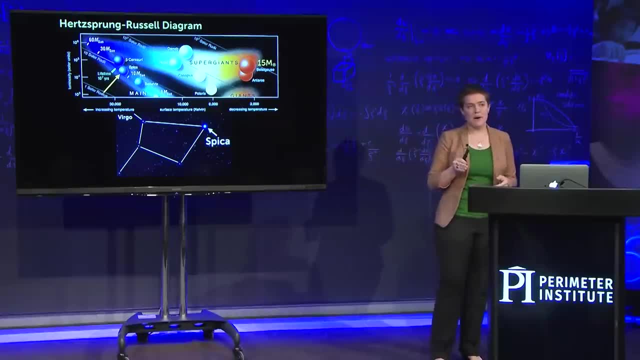 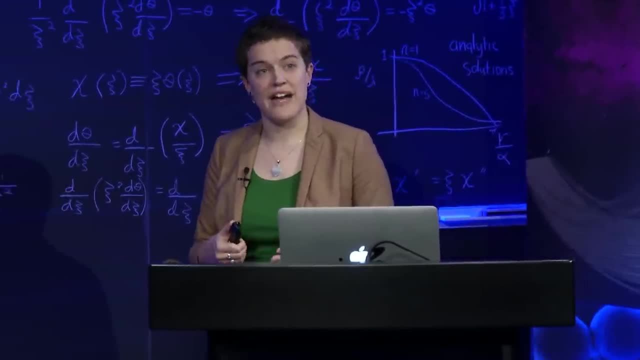 the size A star like Spica will stay in this part of the HR diagram for maybe 10 million years. So it's fusing hydrogen into helium. Eventually the star will run out of hydrogen and it needs to try fusing something else, So it switches from fusing hydrogen to helium. When that 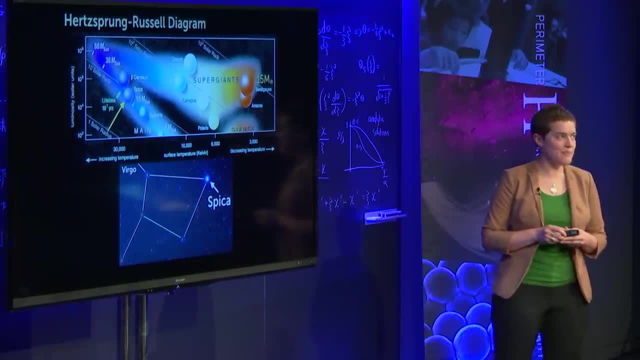 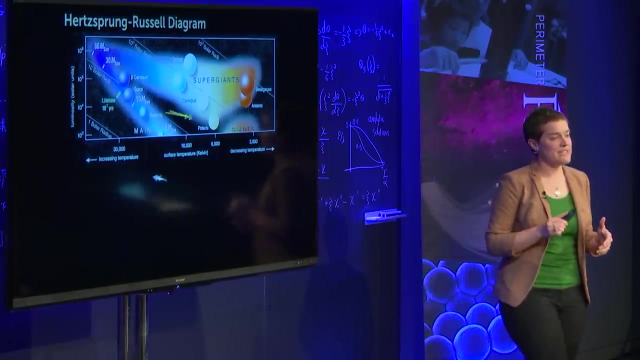 happens, the stars actually go streaking across the top of this diagram from left to right very quickly. After 10 million years fusing hydrogen, they cross from the hot to the cool side of the plot in about 100,000 years. Along the way, though, they make a brief pit stop. 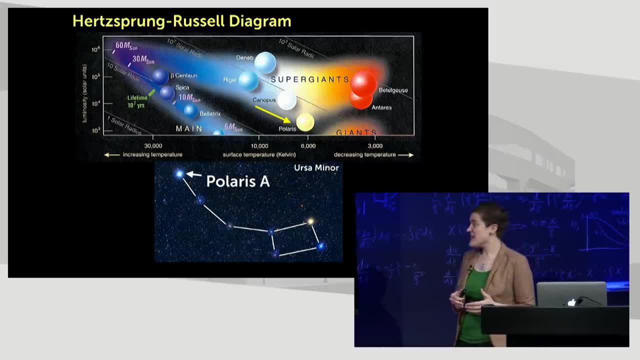 when we would consider them yellow. We actually have an amazing example of a yellow supergiant that we all know really well. Our north star, Polaris, is a yellow supergiant. This is actually pretty surprising, because stars like this are rare since their lifetimes are so short, So it's pretty cool that our 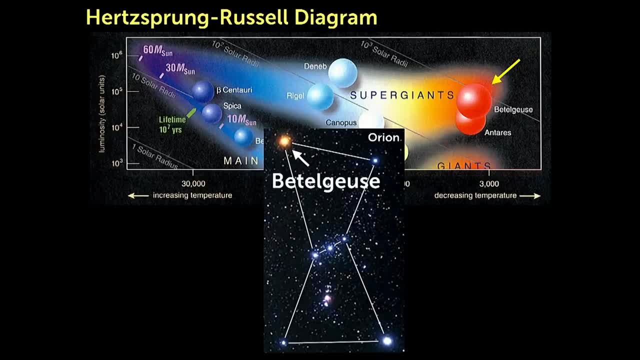 It's very easy to find in the night sky if you look for those three stars that make up his belt And you can see Betelgeuse as his left shoulder. It's a very bright star that is very obviously red. Betelgeuse is an excellent example of a red supergiant, which are one. 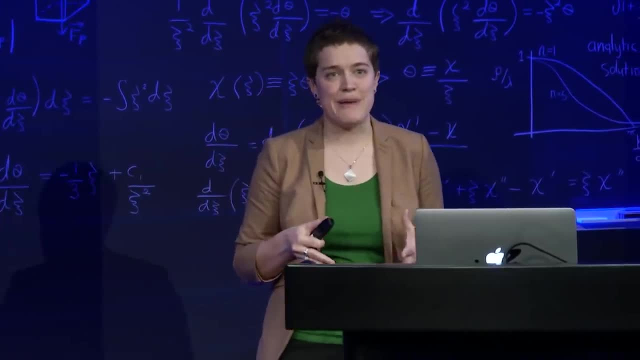 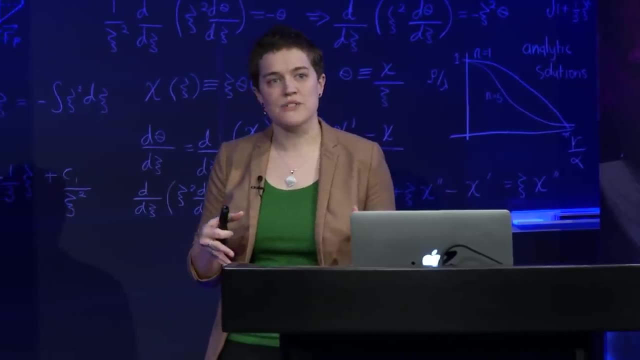 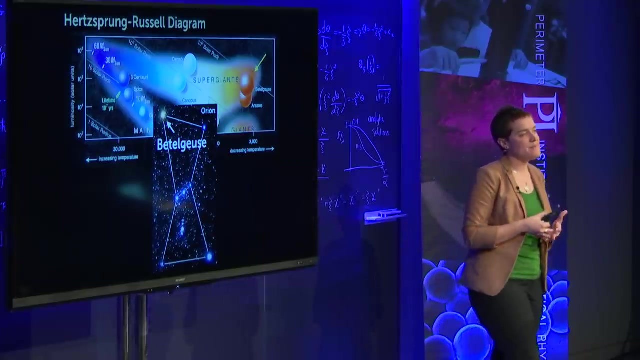 of my research specialties and a particularly fascinating type of massive star. What's interesting about a star like Betelgeuse is that, as it has cooled off and moved across the Hertzsprung-Russell diagram, it's also gotten enormously big. This star was born with maybe 15 or 20 times. 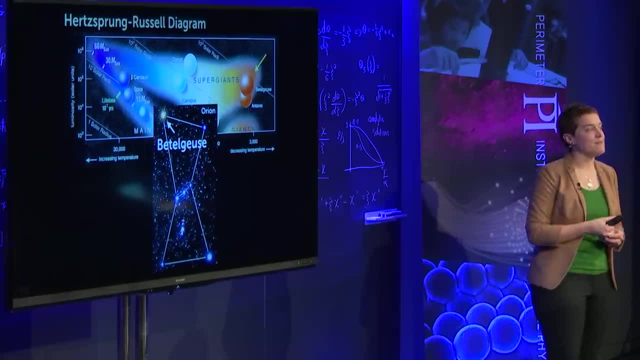 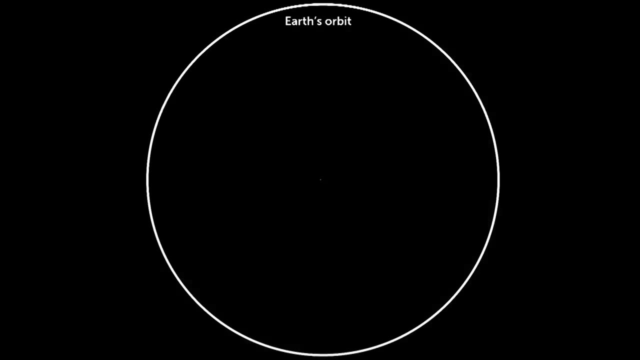 as much mass as the sun, But it's 900 times the sun's size. So I want to try and put that into context. This is the orbit of the earth. That one dot in the center- it shows up as a couple of pixels on the projector- is our sun. If we back up a little bit, we lose sight. 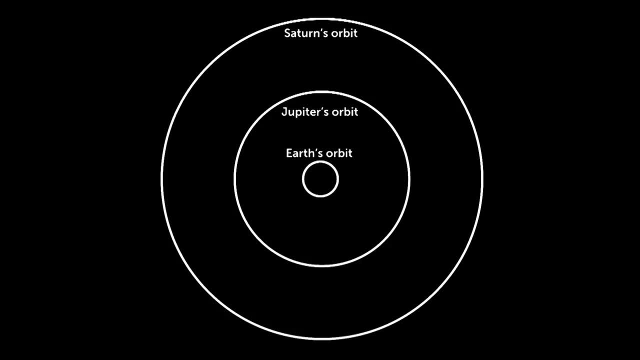 of the sun, the size of Earth's orbit relative to things like Jupiter's orbit and Saturn's orbit. If we were to put Betelgeuse where our sun is, it would stretch out to well past the orbit of Mars. It would begin. 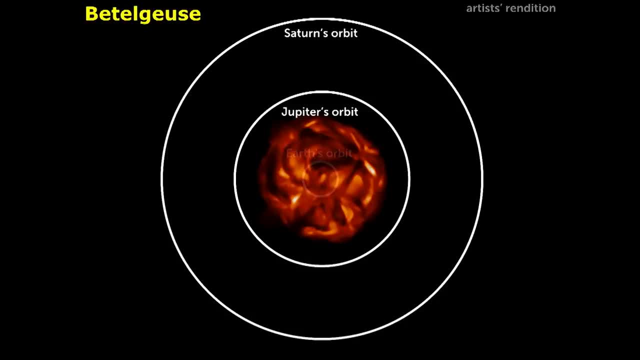 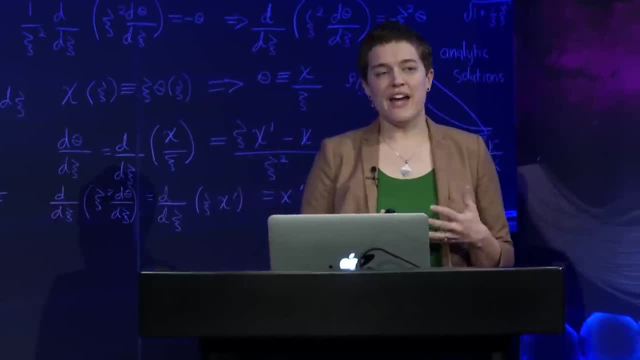 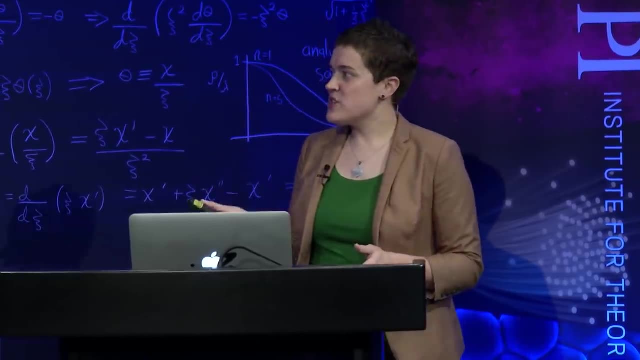 approaching the size of Jupiter's orbit. So this is incredibly big and in its own right, makes the star a bit weird. There's a couple funny consequences of a star being this big and this cool, And I want to again try and compare it to the sun. So this is an image of our sun And if 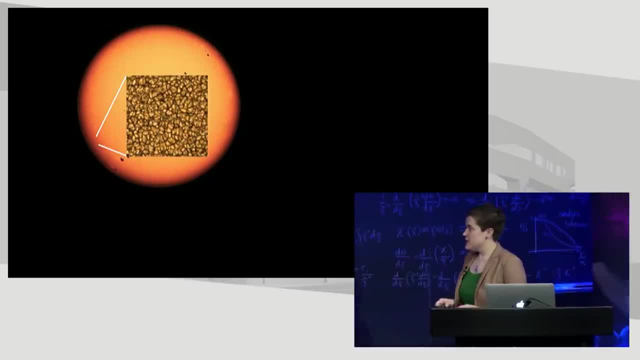 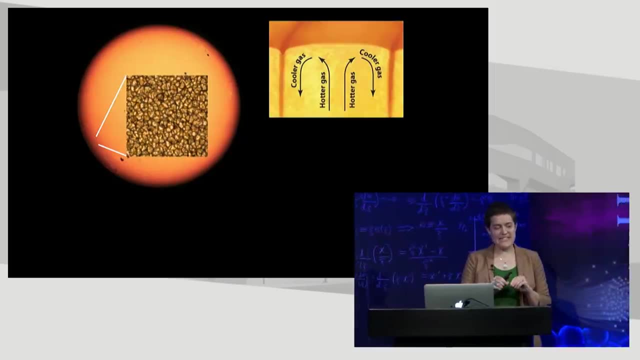 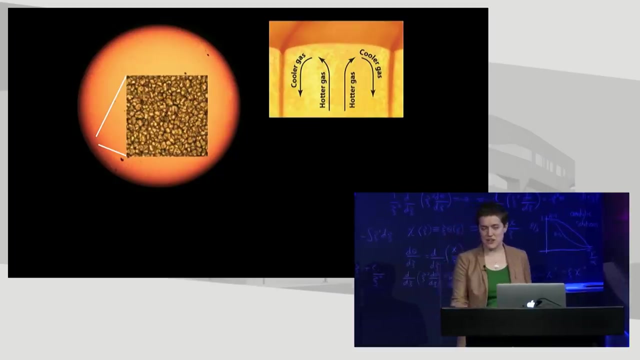 you were to zoom in on it very close, you would see things like this happening on the surface of the sun. These are called granules. What we're seeing are the very tips of a convective layer in the top, near the surface of the sun. What we're seeing is gas that starts out hot rises to near. the surface of the sun cools off and then falls back. It's not unlike watching bubbles boil in a pot of water. So on the scale of the sun, these are tiny, But stars like red supergiants do this too, and the effect is a good deal more dramatic. So if I put the sun away, it is now a. 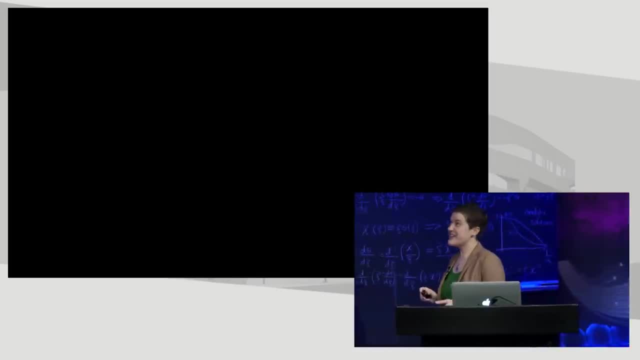 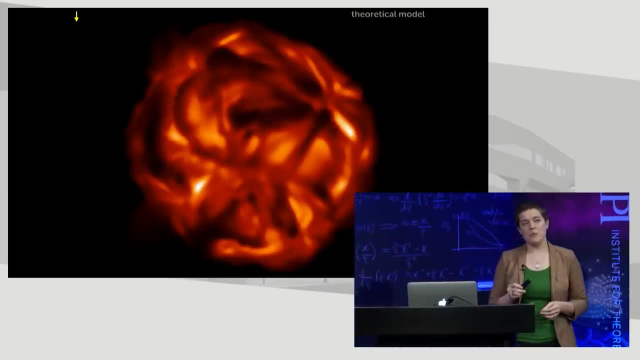 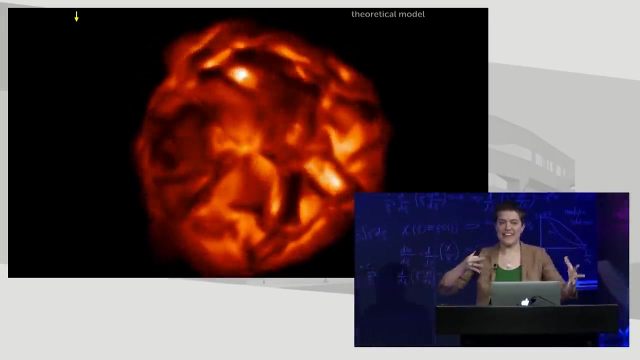 single pixel on the screen, but I promise you it's still there. We can, to scale, compare the sun, there it is, to Betelgeuse. This is what those same little cells look like on the surface of Betelgeuse. The whole star is boiling and roiling. 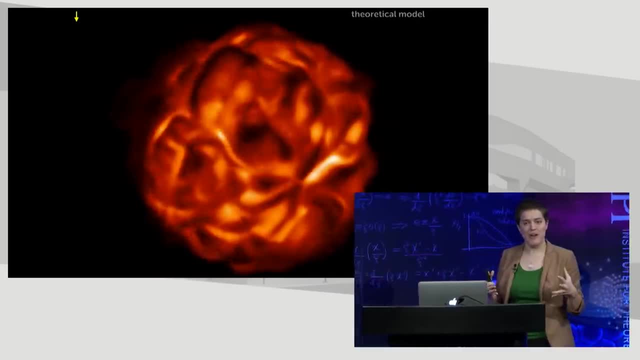 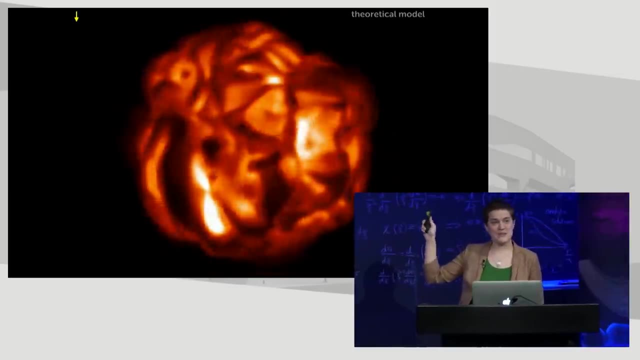 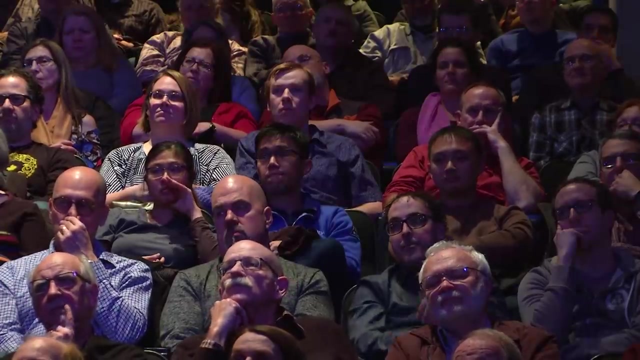 And changing very dramatically when you look at how bright it is. This is a consequence of how large and how cold it is, And this is a normal red supergiant. This is very typical for stars like this, So it starts to establish why these stars are as interesting as they are. We went through 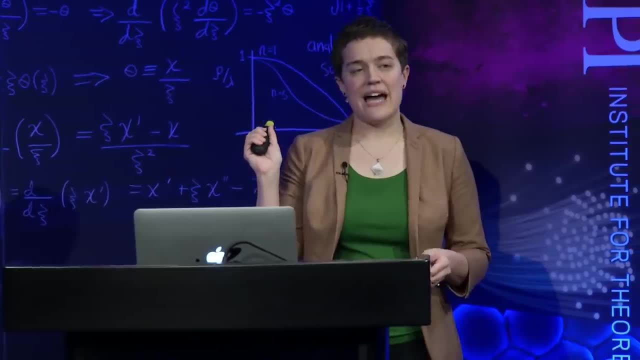 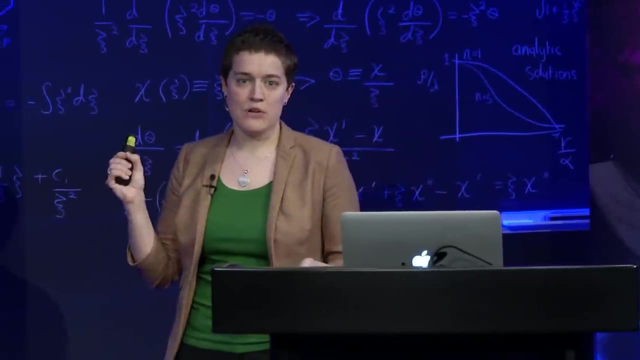 the Hertzsprung-Russell diagram and we followed stars starting as hydrogen-fusing blue supergiants, crossing the diagram to briefly become yellow supergiants and ending up as helium-fusing red supergiants. We can actually draw a line to represent the journey that. 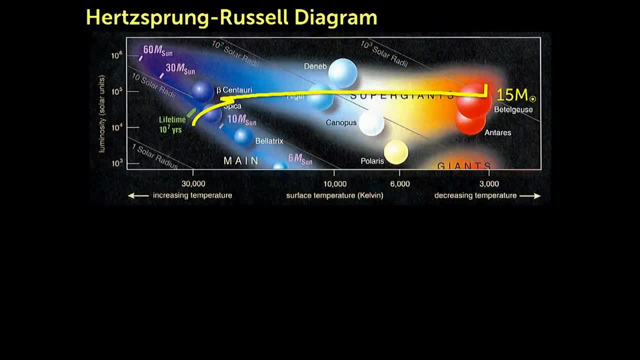 we just followed. This is how a 15 times the mass of the sun star would move during the course of its lifetime on the Hertzsprung-Russell diagram. We call something like this an evolutionary track, and it's a great way to quickly and at a glance look at how a star is going to. 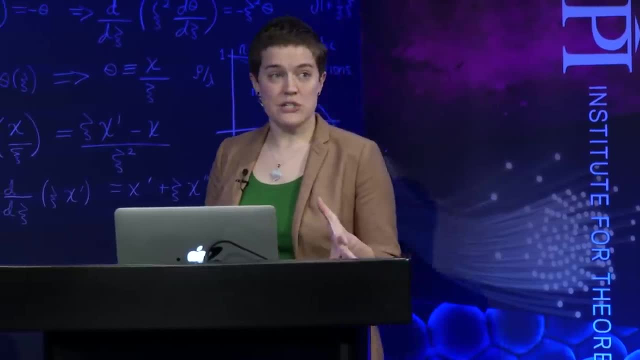 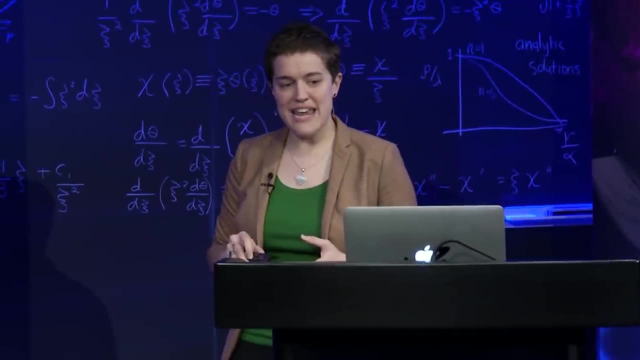 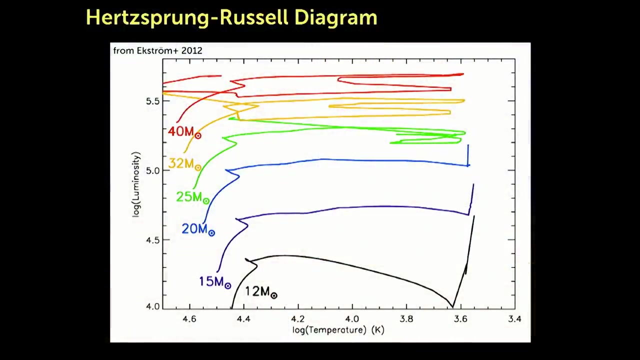 behave during its lifetime. This is actually a really great tool for studying theories of how stars evolve. This is an evolutionary track for a 15 solar mass star, but we can take a bunch of evolutionary tracks like that and draw them on a Hertzsprung-Russell diagram We can look at what a 12 solar mass 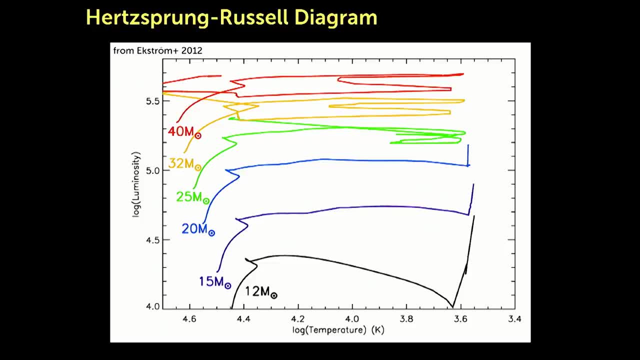 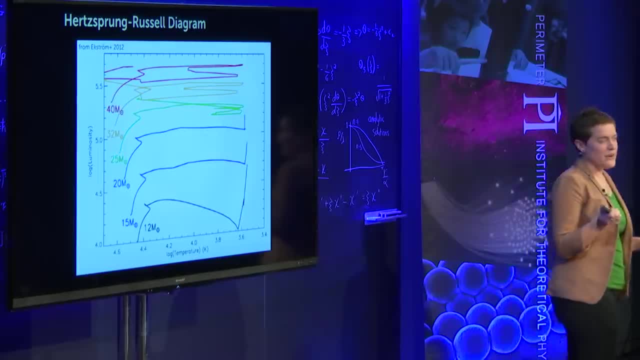 star will do, what a 20 solar mass, what a 40 solar mass star will do, and get a good sense of what normal mass of star evolution looks like. So there's something you might notice on this diagram and it has to do with how cold the stars get Every one of these. 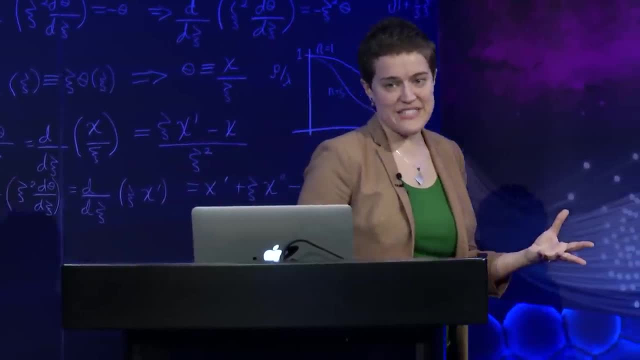 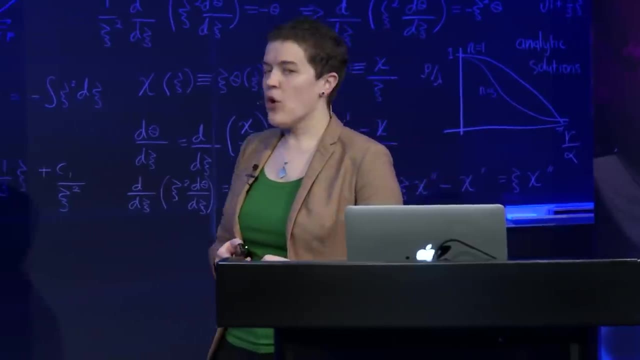 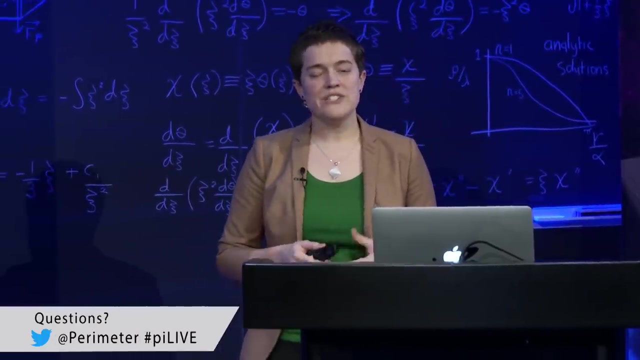 evolutionary tracks was computed using our understanding of stellar physics, and every single one seems to stop at about the same temperature. Every one is not really getting any colder than about 3,000 degrees Celsius or so. To the right is this region where we don't think stars. 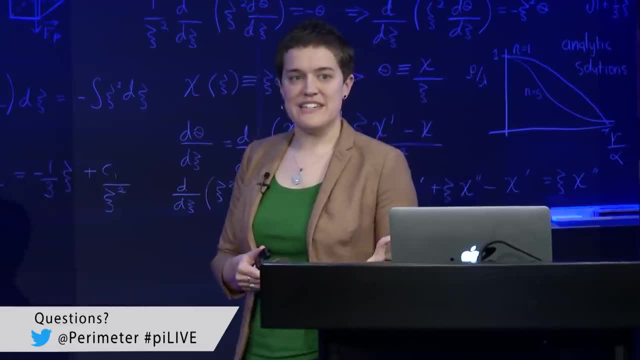 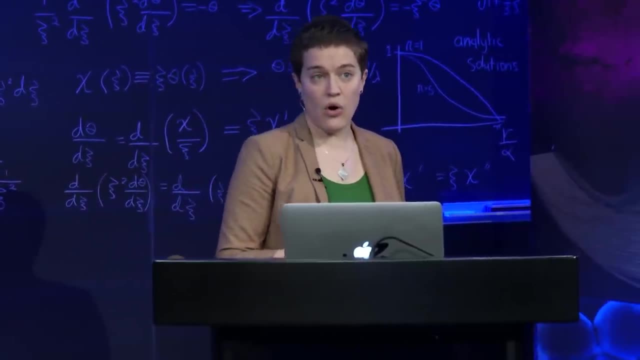 should be able to stably exist. Everything we know about stellar physics suggests that stars should not sit in this part of the diagram. Now I mentioned red supergiants and I mentioned that they're incredibly cold, So we think that those stars should sit right at the edge of these evolutionary tracks. 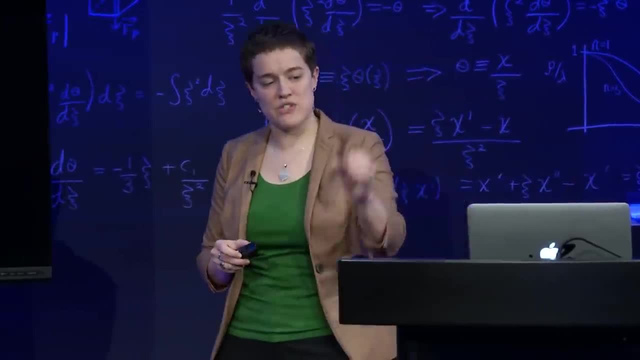 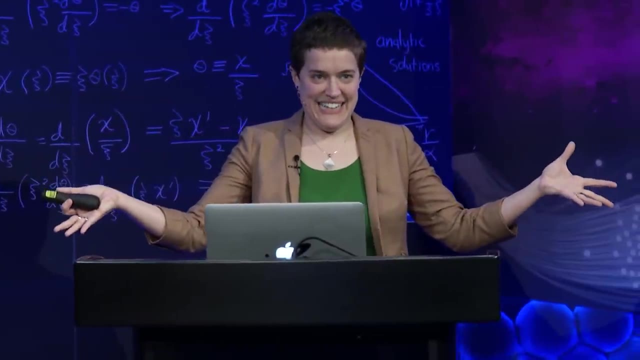 but for a long time. if we observed red supergiants, if we measured their temperature and we measured their brightness and we tried to put them on this diagram, those stars would land here in exactly the place that they don't belong. This bothered us for a very long time. We 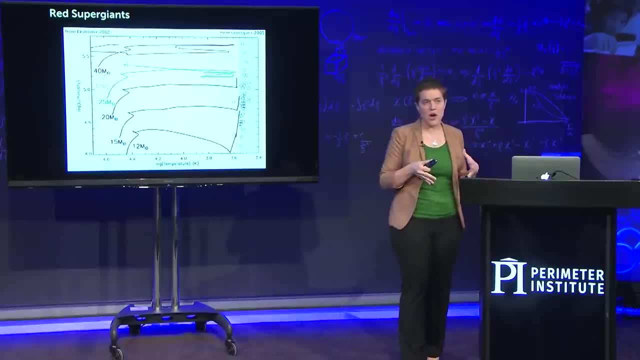 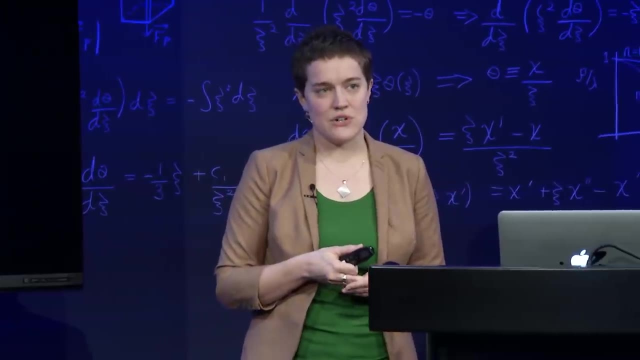 were trying to understand what was wrong with our stellar physics, what was wrong with our theory of how these stars evolved that could explain this really bad mass. So we've got match between red supergiants and the predictions of evolutionary tracks. What finally clued us in was when we started looking at where the temperatures of those 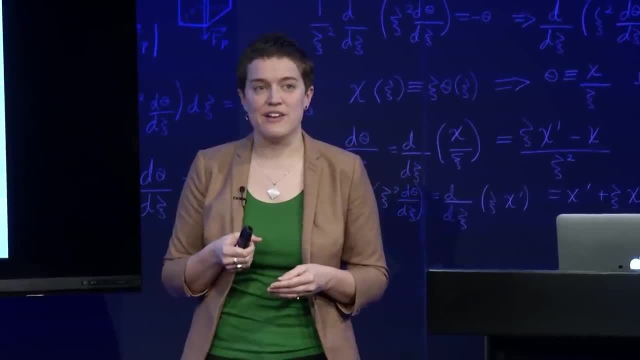 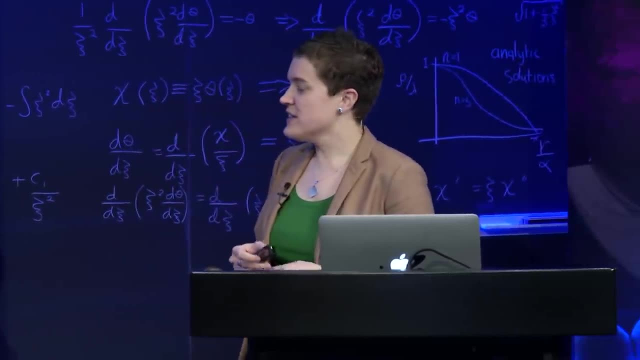 stars were coming from and when we developed a very good way to measure those temperatures more accurately than we had before. The way that we'll do this is to take light from a red supergiant and sort it out into something called a spectrum. 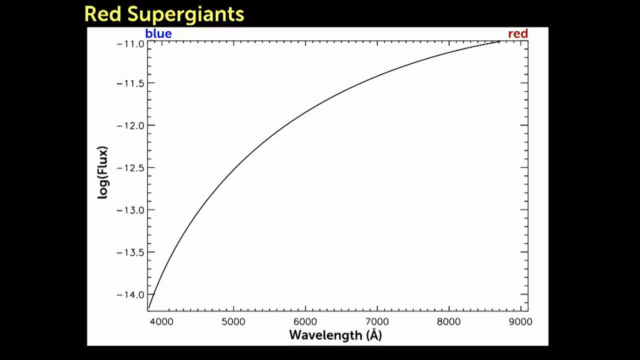 So in a spectrum you observe light from an object and you sort it out according to its wavelength. So the very bluest light will be on the left side of the diagram and the very reddest light will be on the right. The brightness is still represented on the y-axis, so you can tell at a glance that this. 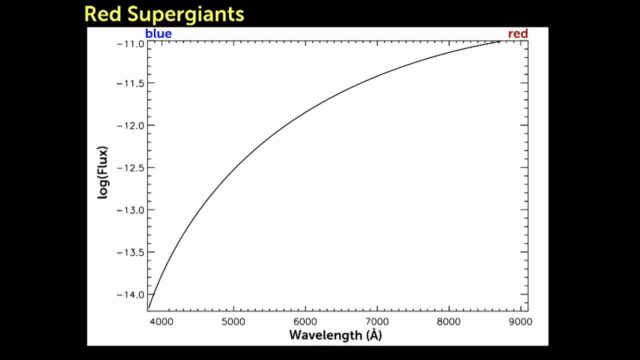 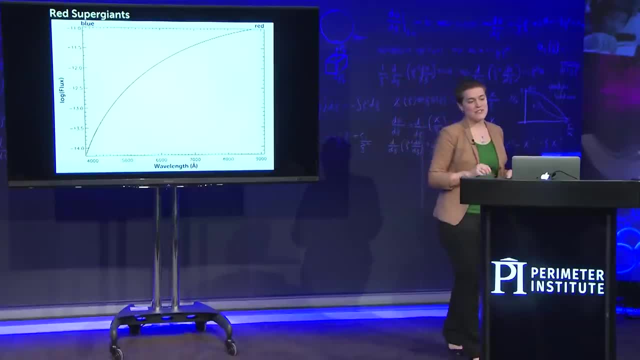 is sort of a spectrum of a reddish star, because we're seeing more red light than blue. This is a cartoon version of what a red supergiant spectrum would look like. An actual red supergiant spectrum looks like this. It's a lot messier, and something you notice right away is that there are these strange. 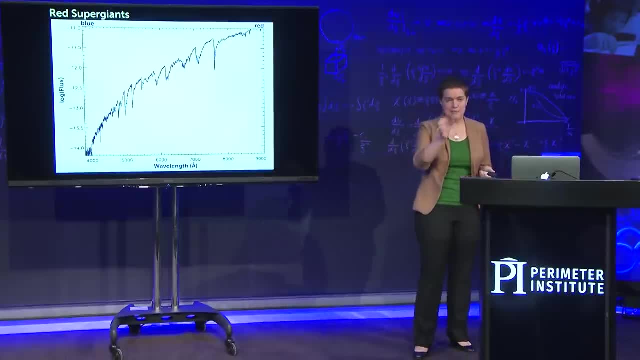 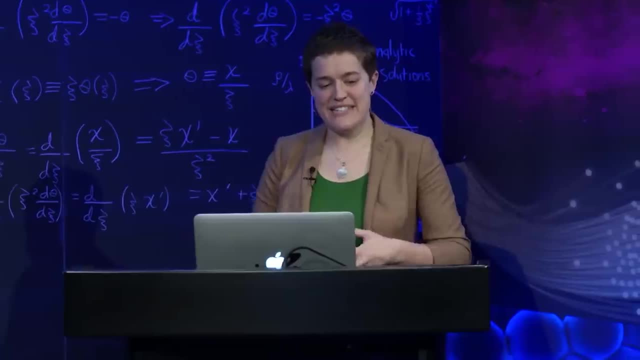 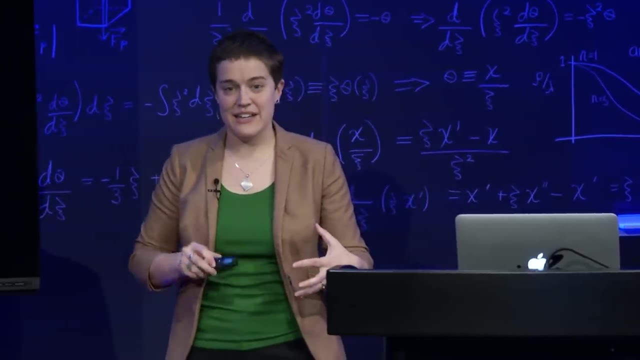 sort of bites taken out of the spectrum. There's these little dips that show up periodically as we go from blue to red. All of those dips represent light that has been taken out of the spectrum on its way to us. That's light that's been absorbed by something in the atmosphere of the red supergiant. 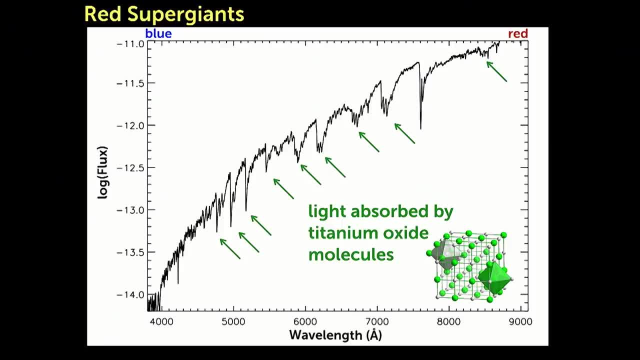 In this case, that is, light being absorbed by titanium oxide molecules. These stars are so cold that molecules are able to form. those molecules- That's, a light that's being absorbed by a blue supergiant- are able to form in their atmospheres. 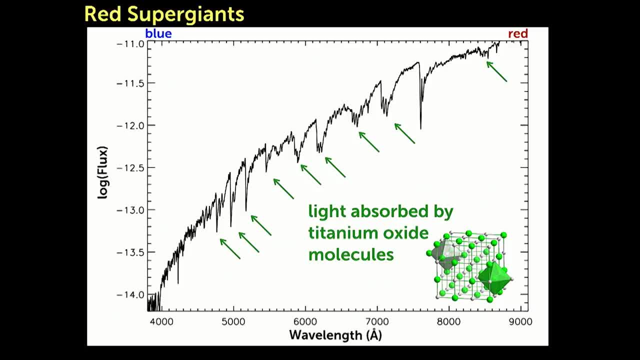 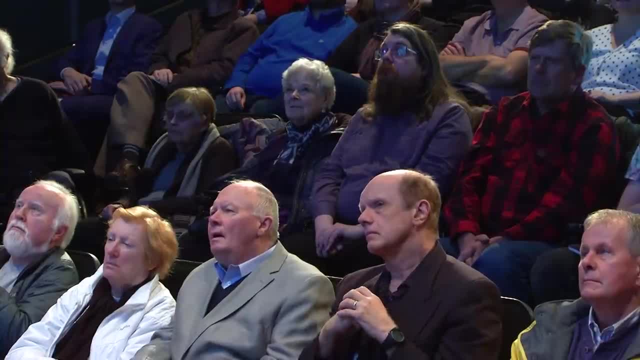 It makes the spectrum look interesting and, as it turns out, it's also a really good tool for measuring temperatures. If you look at a simulated spectrum of a red supergiant and you cool the star off at 4,000 Kelvin. 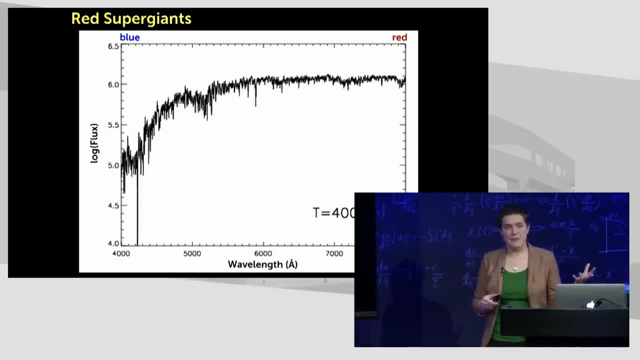 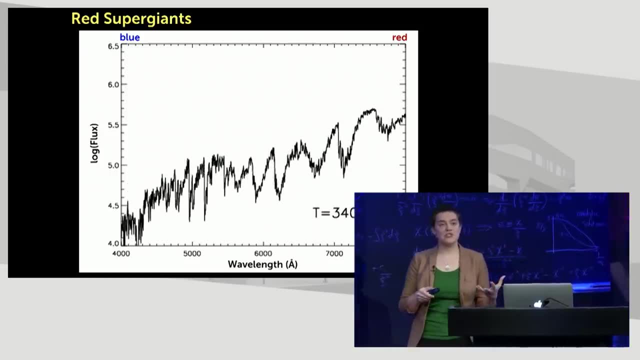 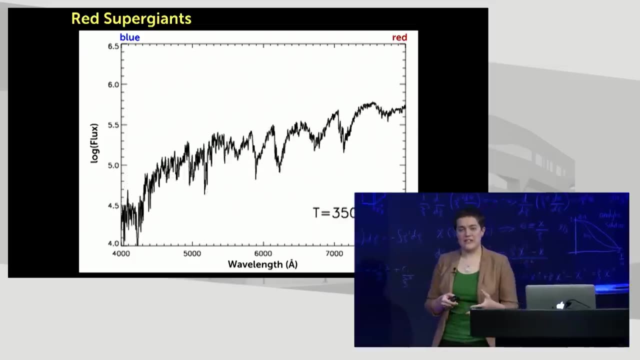 you really don't see that many titanium oxide absorption signs at all. As you cool the star off, they suddenly appear and they get stronger very quickly. What it means is that we can use those dips in the spectrum as tools for measuring temperature. 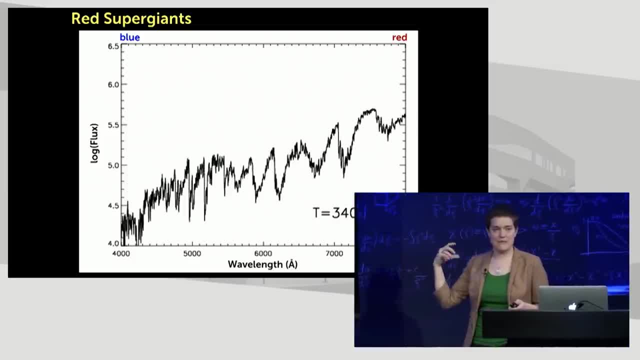 If we observe a star and we see very strong dips, that means the star is very cold. If we see very small ones, it means it's relatively warm. We decided to check this out as a means of maybe improving our temperatures for red supergiants. 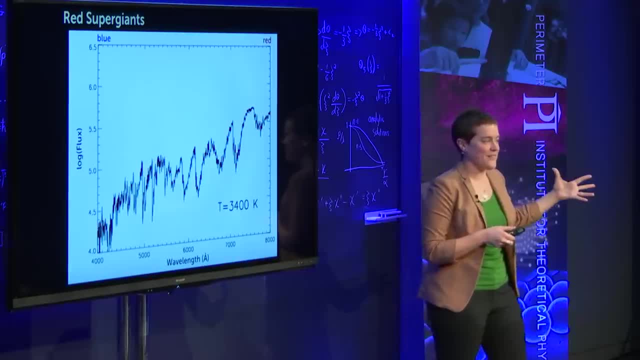 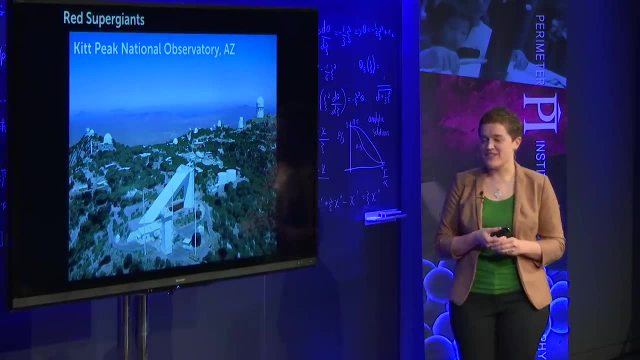 and maybe fixing that problem that we'd come across on the Hertzsprung-Russell diagram. This was actually my very first research project as an astronomy student. I worked on this after my sophomore year at MIT. I got to go to Kitt Peak National Observatory. 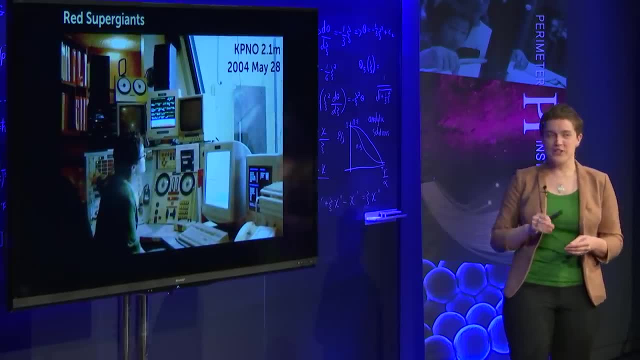 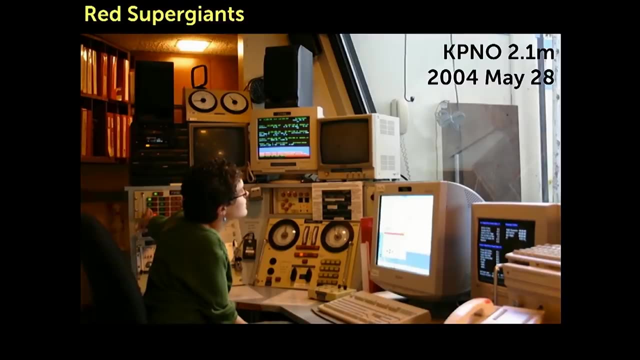 in southern Arizona, I had my very first observing run. You can't tell from this image, but I'm unbelievably excited because they're letting me open the dome of the 2.1-meter telescope and I'm gazing up going ha ha. 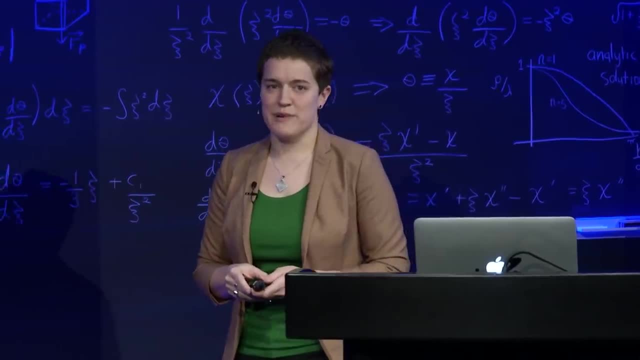 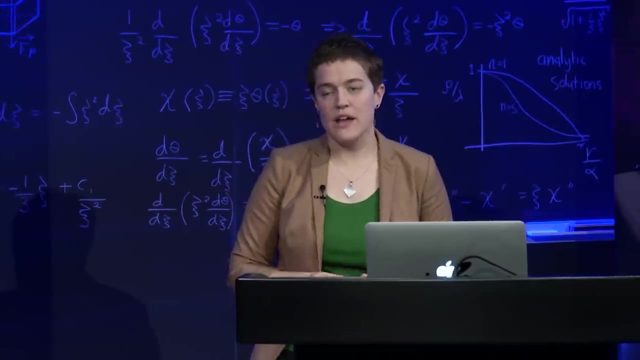 We had five perfectly clear nights. This was wonderful observers, beginners-like, and this has never happened to me again- And we got spectra of 75 red supergiants in the Milky Way. We used that technique, looking at them, and we got spectra of 75 red supergiants in the Milky Way. 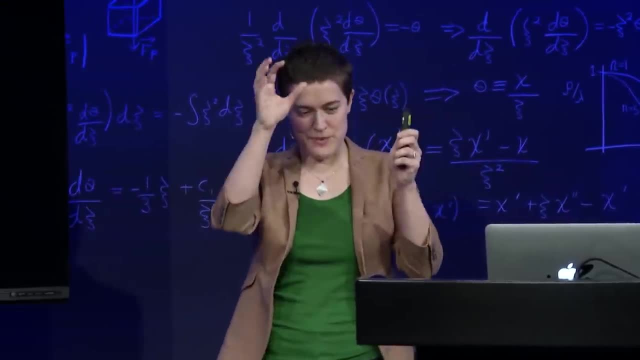 We used that technique looking at them and we got spectra of 75 red supergiants in the Milky Way. We used that technique looking at them and we got spectra of 75 red supergiants in the Milky Way. We used that technique looking at those titanium oxide bites. 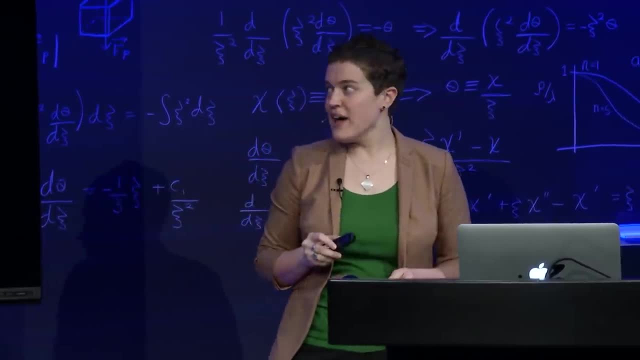 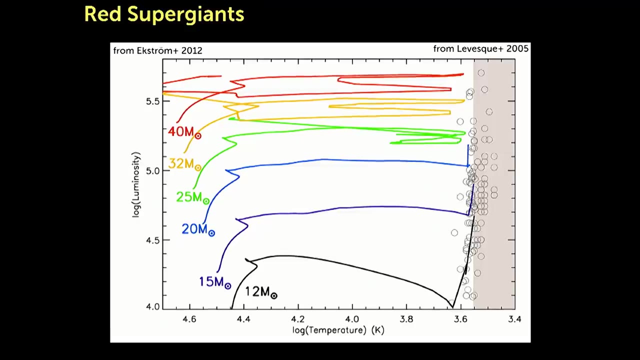 in the spectrum to measure their temperatures, and then we replotted them on this same diagram. So when we remade this with our temperatures, the red supergiants moved from here to here. We had completely fixed the problem. This was enough, that little shift on the diagram. 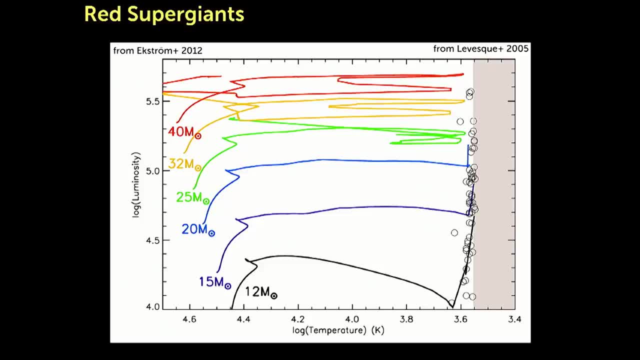 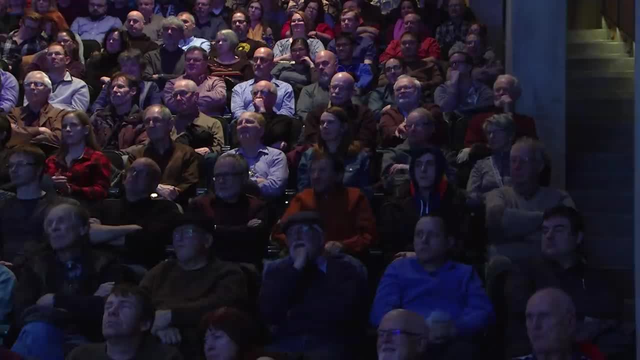 was enough to get us unbelievably excited. Yes, we've done exactly what we set out to do. Physics isn't wrong. These stars work. This is excellent. Let's write the paper, And along the way, we wound up discovering something very cool. 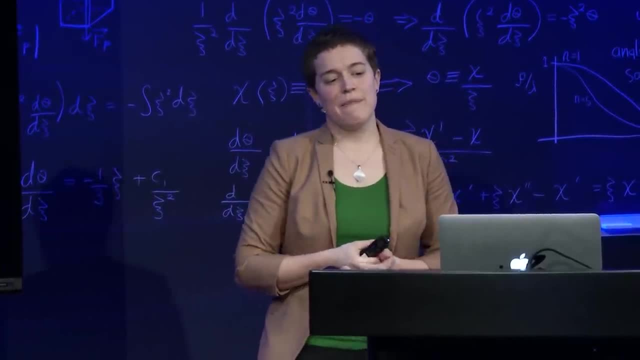 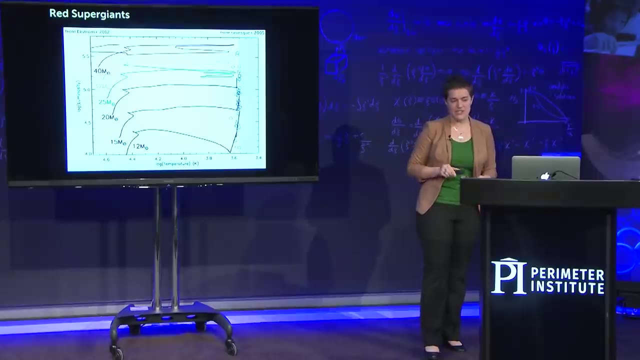 literally and entirely by accident. So on this plot, we've depicted each star's temperature and each star's luminosity, And there's a very handy equation. This is the only equation that I use in the talk, but it's a very important one to have. 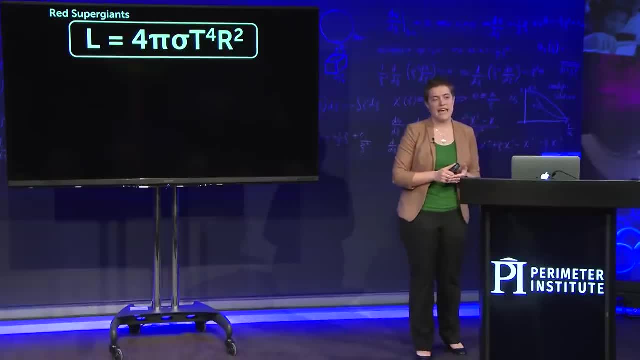 There's an equation in astronomy that relates how luminous a star is and how cold or hot it is to how big it is, And I can walk through whatever you see, And I can walk through whatever you see. And I can walk through whatever you see. 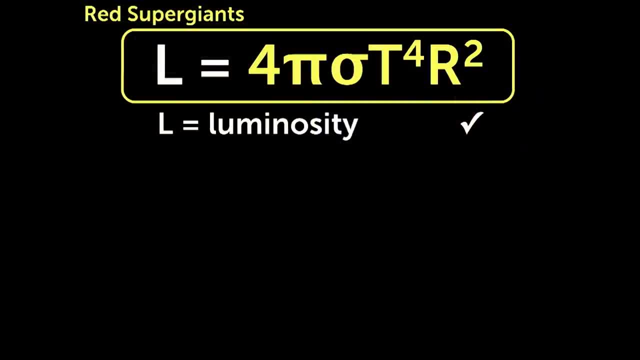 So this is what everything in this equation means. L stands for the luminosity how bright the star is. Well, we already knew that. We know how much 4 is, We know how much pi is, We know how much pi is. 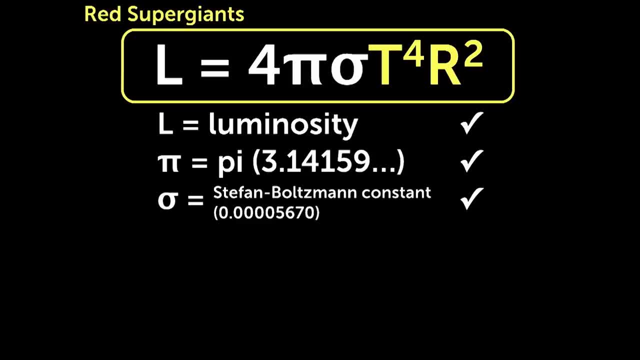 That's just a constant. And we know how much sigma is. That's another constant. We had measured temperatures, So now all that was left was the radius. We had everything at hand, so we figured: why not? This is just an algebra problem. 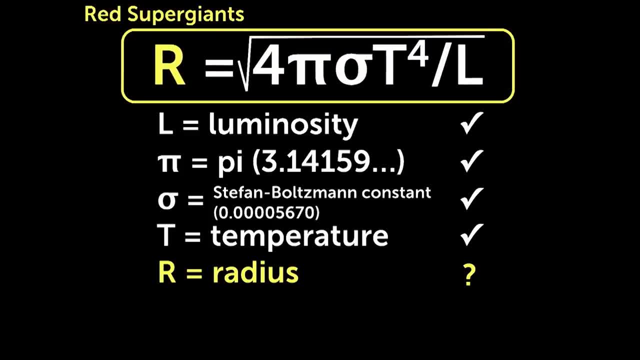 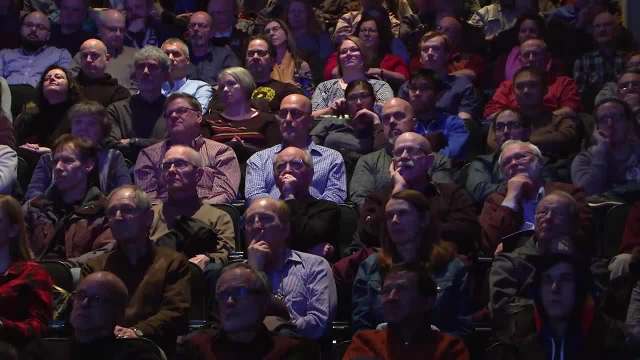 If we move radius to the other side of the equation, take the square root of everything. we've measured radius. So we went ahead and we're starting to see and calculated the size of every star in our list and we put everything in a big table. 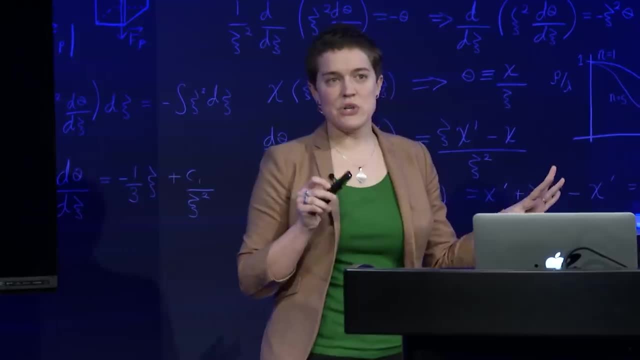 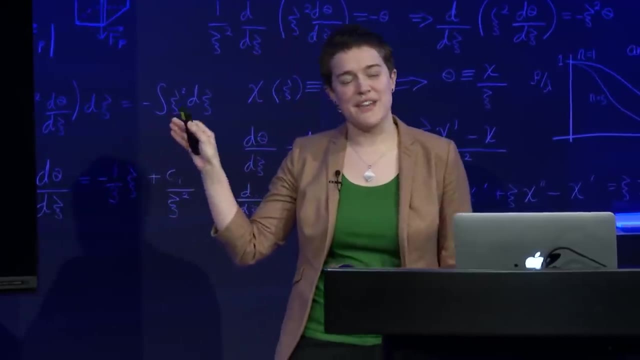 and we started moving on to try and publish the paper. It took one of our research collaborators looking at this table and going hang on. I don't know if you've noticed one of the numbers in this list, but it's astonishing. This is the largest radius I've ever seen measured. 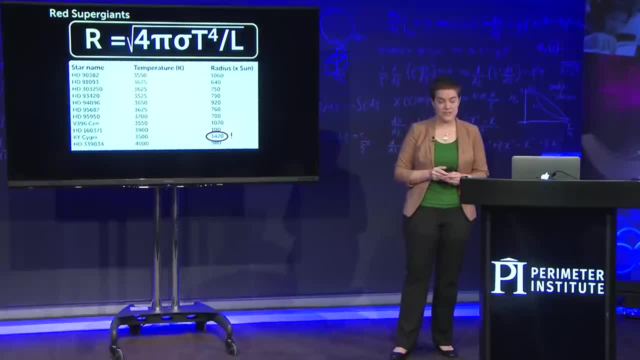 We might have discovered the largest stars in the universe. We went back and did everything again. we checked everything twice, but it turned out it was true. As part of this project, we had by surprise discovered the very largest stars that anyone had ever seen. 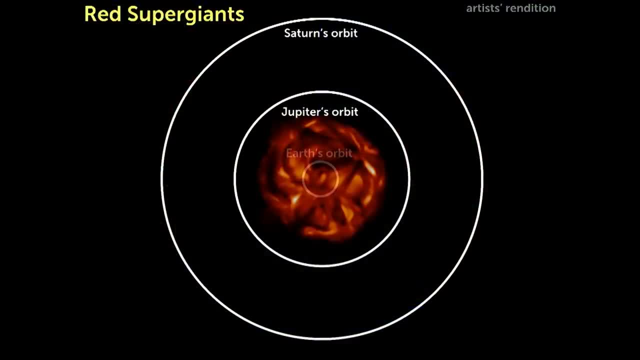 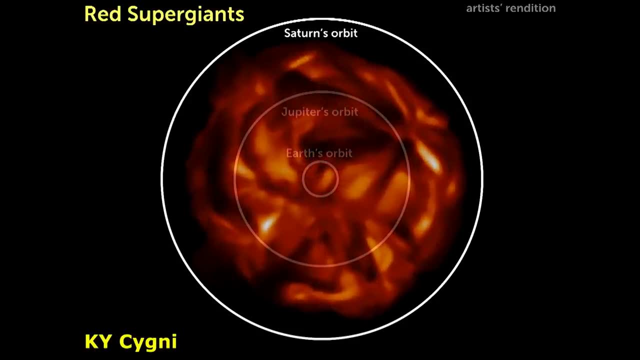 So, for comparison, I showed you where Betelgeuse sat, if we put it where the Sun was and compared it to the orbits of the planets. This is the size of our new record holder, a star named KY Cygni. It reaches out well past Jupiter. 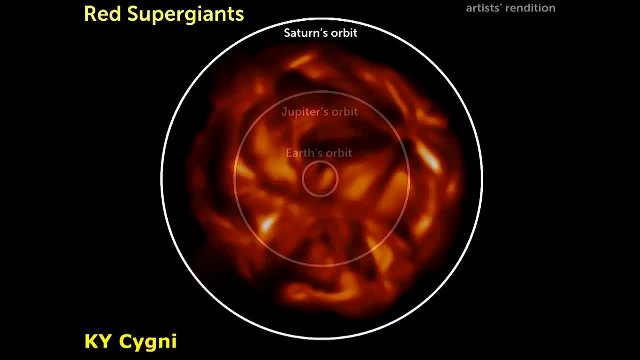 It starts approaching the size of Saturn's orbit. So this on its own, hitting this extreme of stellar evolution, most definitely marks KY Cygni as a weird type of star. So we've gone through how stars move on the Hertzsprung-Russell diagram. 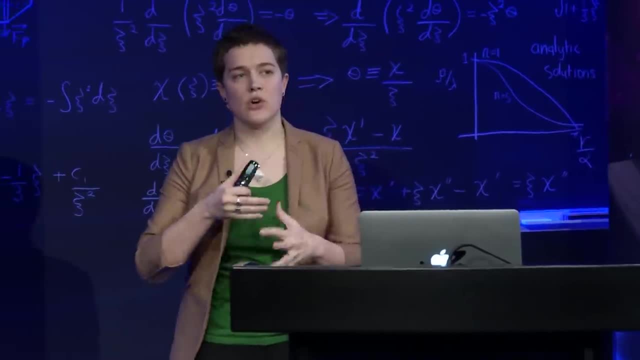 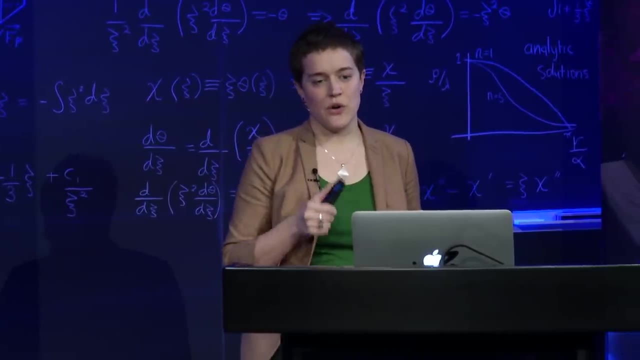 We've talked about these cold red supergiants fusing helium in their cores and how they can get fascinatingly big, But eventually those stars also run out of things to fuse in their cores. Does anybody know what happens when we get to that point? 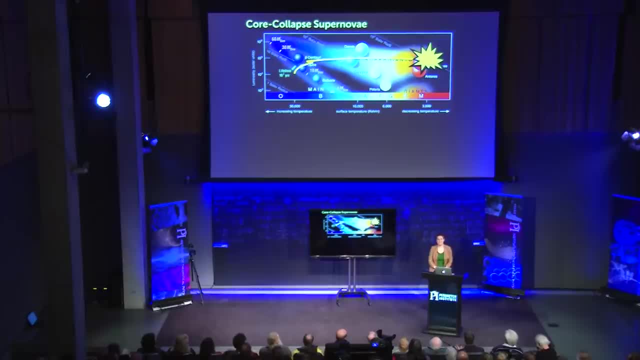 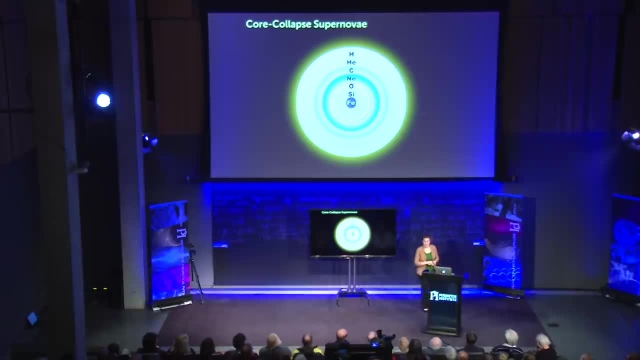 Supernova, Yes. So to understand why a supernova happens, it helps to look at what's going on inside the star. right before the supernova, Massive stars started out their lives fusing hydrogen into helium. then they moved on and fused helium into carbon. 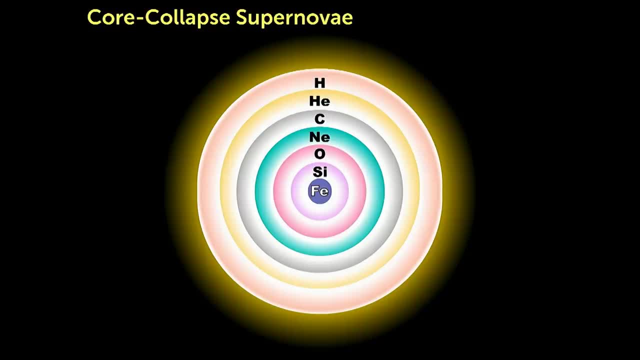 and they progressed, fusing heavier and heavier elements By the time they reached the ends of their lives. if you were to slice one of these stars in half, it would look like the inside of an onion with layers of every single element that it's been using for fusion. 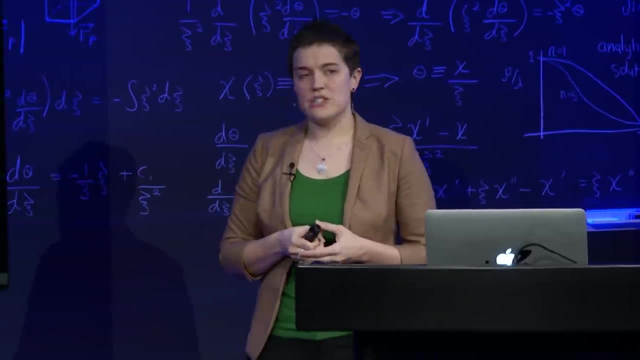 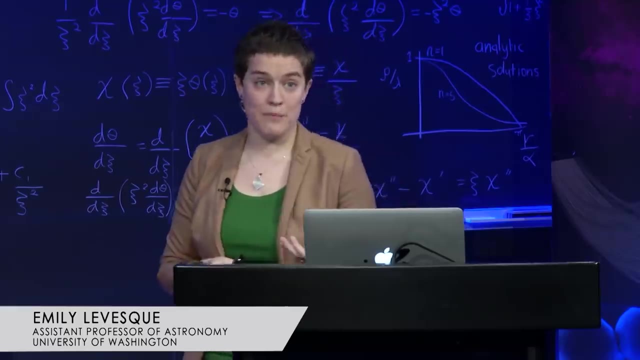 or as the product of fusion inside. This star gets into trouble when it starts to try and fuse iron. This fusion happening in the core of the star serves a very important purpose. It helps the star maintain this very delicate balancing act between the inward press of gravity. and the outward press of that fusion. As long as that balance is maintained, the star is going to be alive and it's going to be just fine. Fusing iron disrupts this process, because fusing something like hydrogen or helium or carbon produces energy. 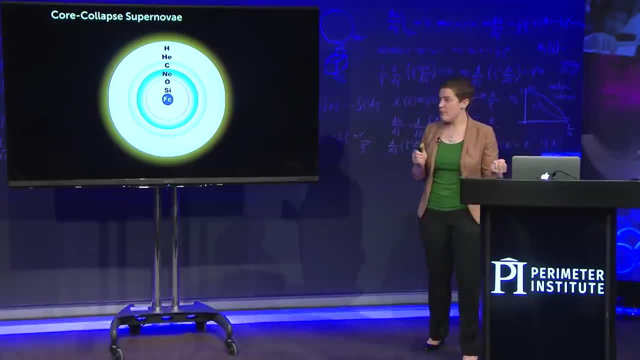 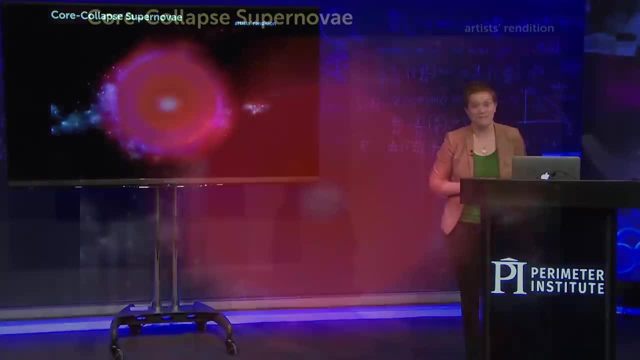 If you try to fuse iron, you need energy. At this point, that delicate balancing act has been disrupted. I have an animation of what happens once we do that. In this animation, we're zooming into the center of a red supergiant. 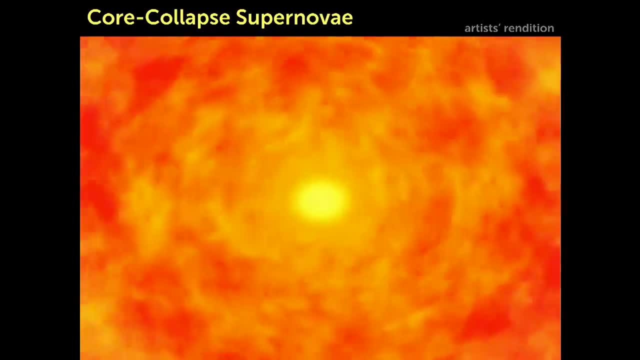 You'll see the colors in the center of the star change to represent different fusion processes that are occurring as we switch from fusing hydrogen to fusing helium, As we switch from fusing helium to fusing something like carbon. you'll see the color change again. 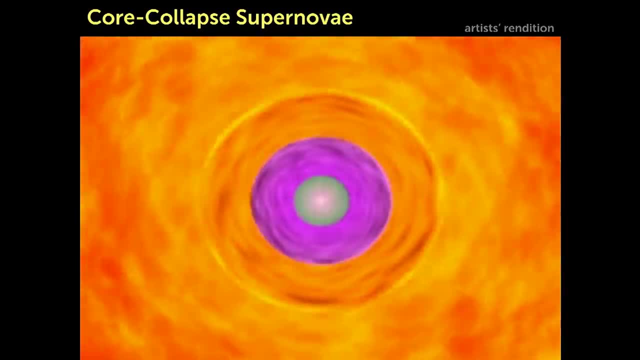 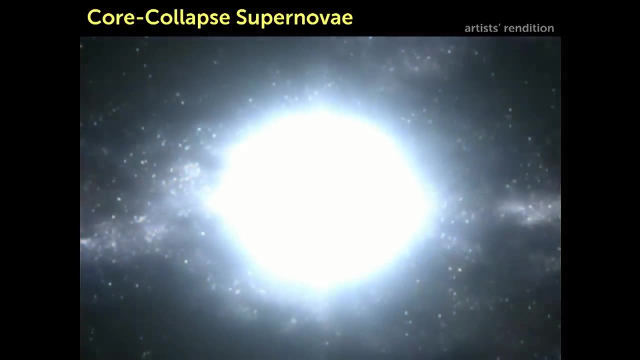 The star will progress through different fusion sources until it attempts to fuse iron. This goes terribly for it. Then in less than a second, that iron core implodes. All of the material in the outer layers of the star tumbles down onto that imploded core and then bounces back out. 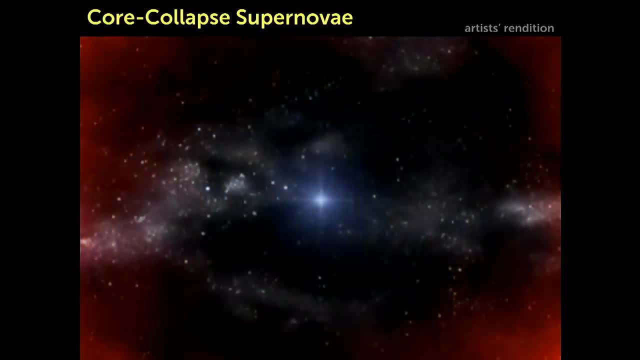 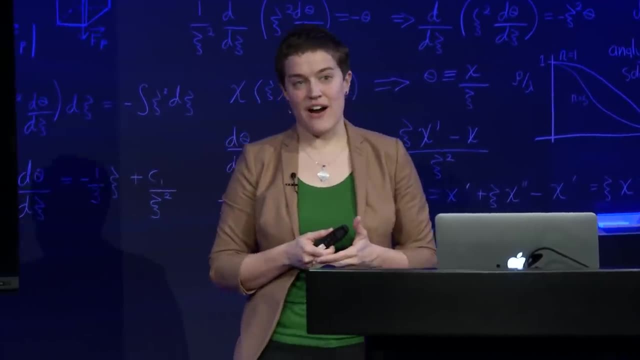 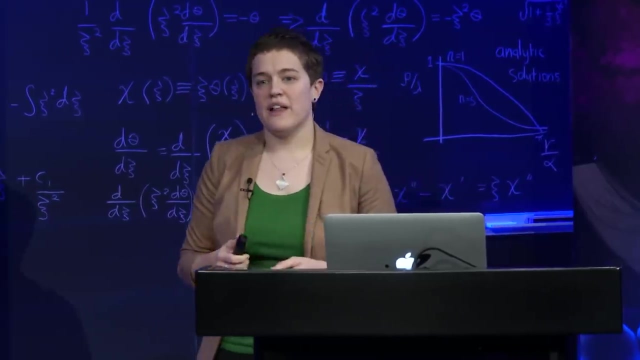 That rebound bounce gives us this unbelievable explosion that we see as a core collapse supernova. This is an incredibly dramatic death for a star. Supernovae are amazingly bright. This picture here is from a cave dwelling in Chaco Canyon, New Mexico. 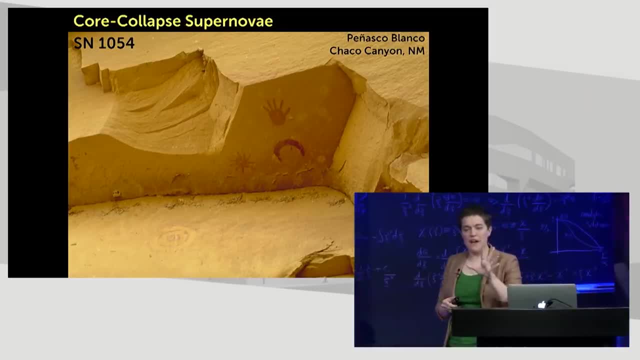 It shows a few illustrations on the rock. You can see what looks to be a daytime moon. You can see a person's hand. Then you see this. This we believe is a depiction of supernova 1054.. This supernova went off on July 4th 1054,. 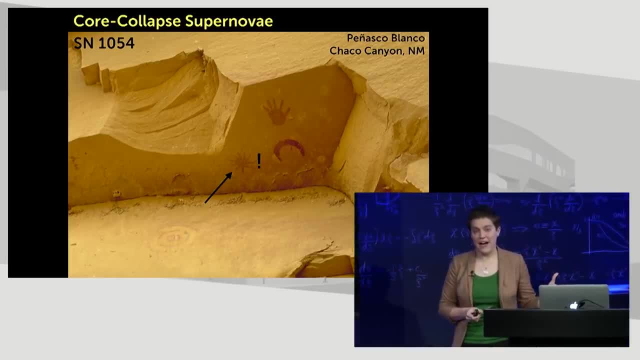 and was in our own galaxy. It was very nearby. It was so bright that you could see it during the daytime sky for two weeks. We have historical records of it from Arabic astronomers, from Chinese astronomers. They called it a guest star because it appeared, stayed for a little while and then left. 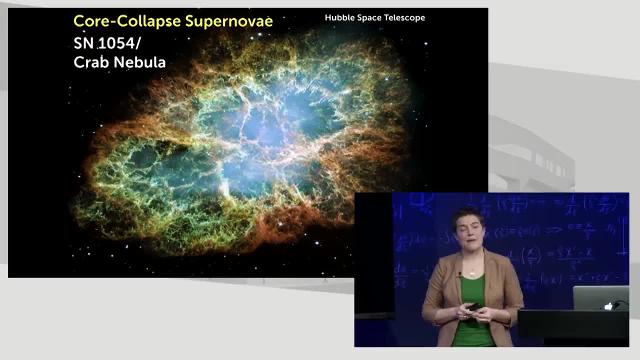 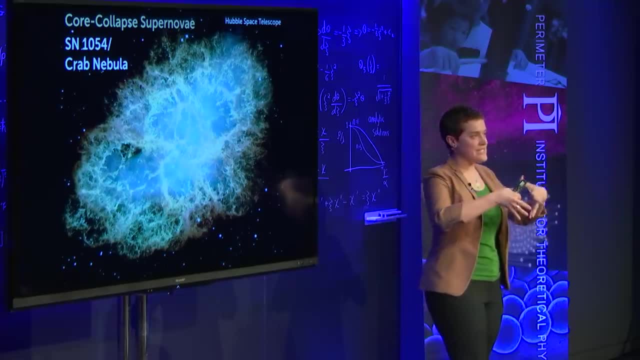 This actually left behind what we now know as the Crab Nebula. The Crab Nebula is the remnant of that 1054 supernova. all of that material that got blasted off of the star, now dissipating into interstellar space and giving us what we call a supernova remnant. 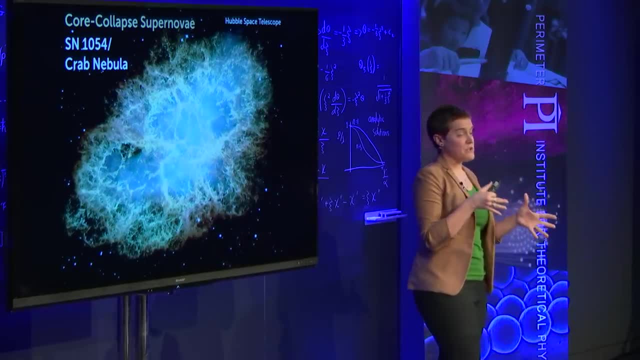 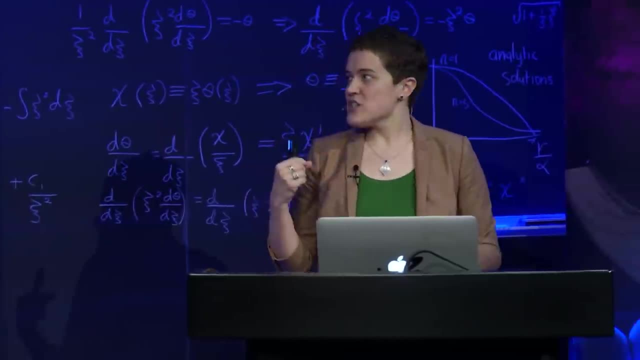 That was an unbelievably dramatic supernova and it was extremely bright, in part because it was so nearby. It was in our own Milky Way. We had a supernova like this in 1054.. There was a supernova in 1572, one in 1604,. 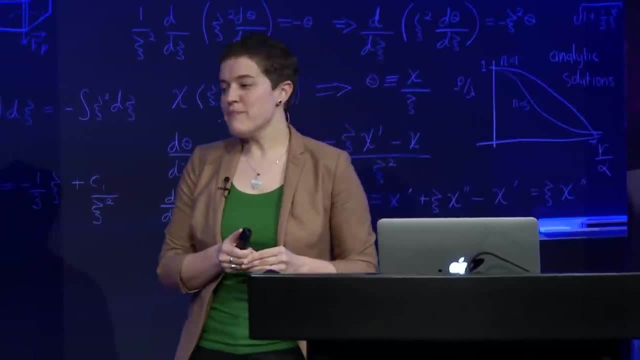 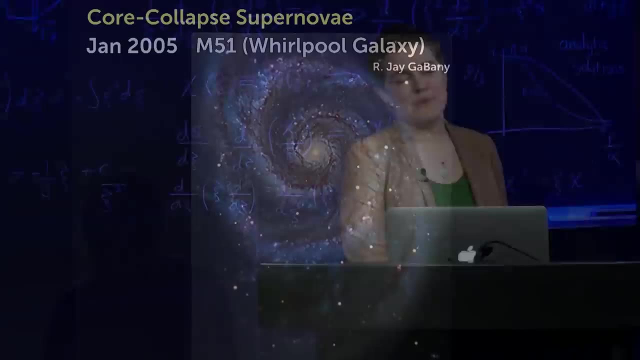 and we haven't had one since Every modern supernova that we've studied has been in another galaxy, and it's a little bit less of a fireworks show. This is an image of M51.. This is the Whirlpool Galaxy. It's an image from January of 2005.. 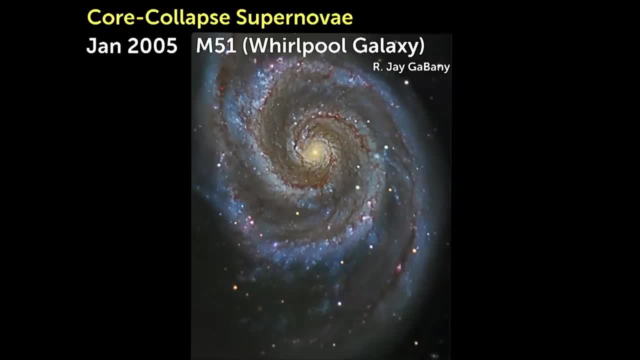 In July of 2005,, a supernova went off in M51.. There's actually a really great image of that supernova happening. Did you see it? Such a dramatic explosion? Let me do it again. Yep, Usually when I turn it off, then I just oh. 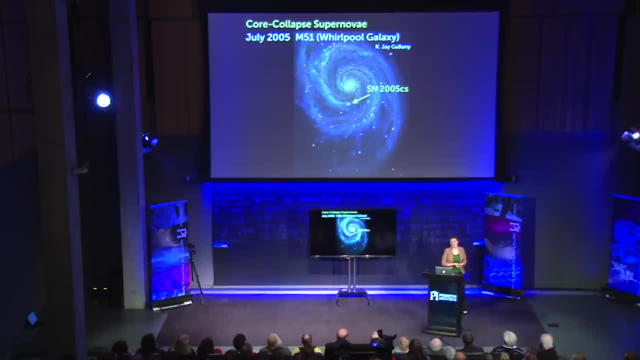 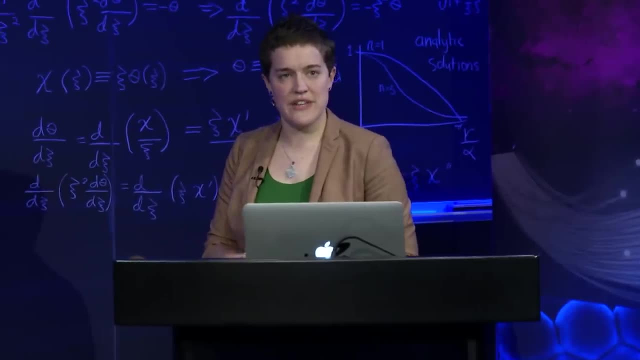 That was the dramatic supernova 2005 CS. It's the same supernovae based on the year that they happen and how many we've seen in that year. This supernova happened in 2005.. We started with supernova A, B, C, D. 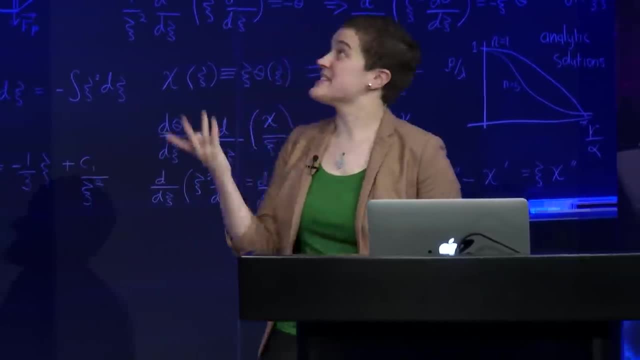 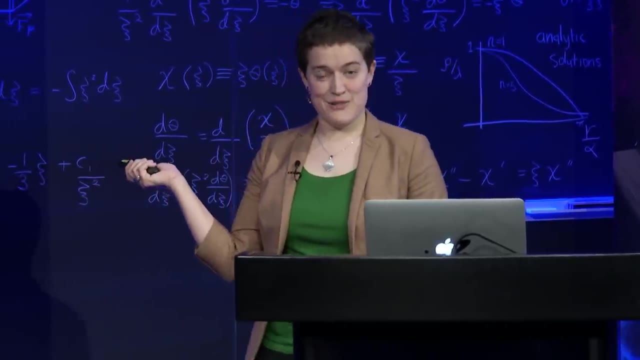 and went through the lettering. These supernovae are fairly common. You can tell if we got all the way down to CS. there's quite a lot of them. This was a pretty bright and still pretty dramatic- by astronomy standards- supernova. 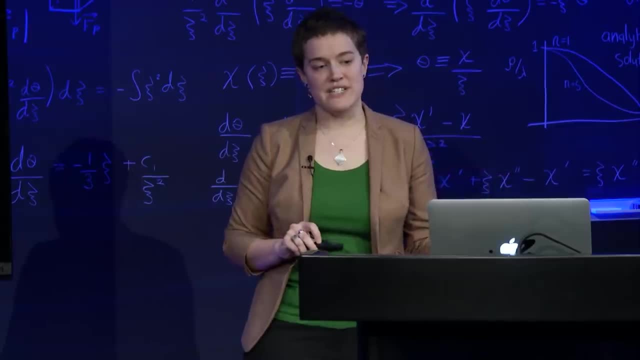 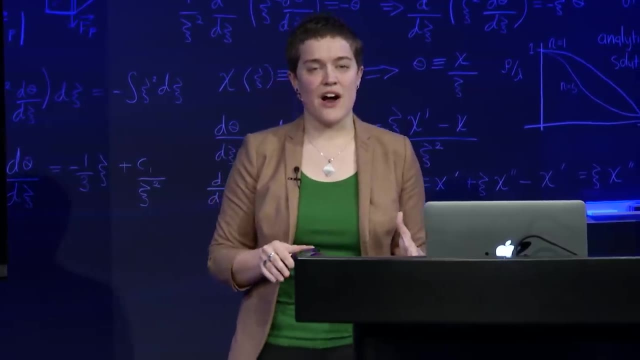 We cataloged it and we watched it do what a normal supernova does: It got incredibly bright and then, over the course of about a year, it faded away. This is what an exploding star should do. Sometimes we see something a little bit different. 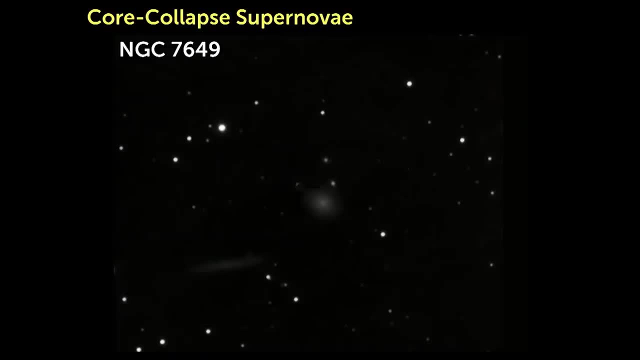 This is the beautiful galaxy NGC 7649.. By galaxy I mean the little fuzzball in the middle of the picture. As we get farther away, the photos get a little bit less dramatic. This galaxy hosted a supernova, we thought in 2009.. 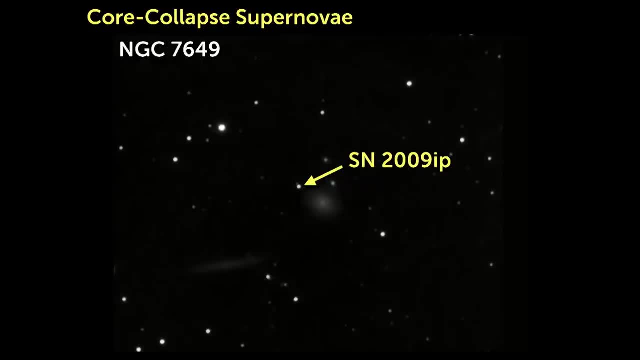 This little bright thing appeared. We identified it and immediately said: hey, we found another supernova. This is supernova 2009 IP- It got that name. We saw this thing get very bright. We watched it fade away and we thought: 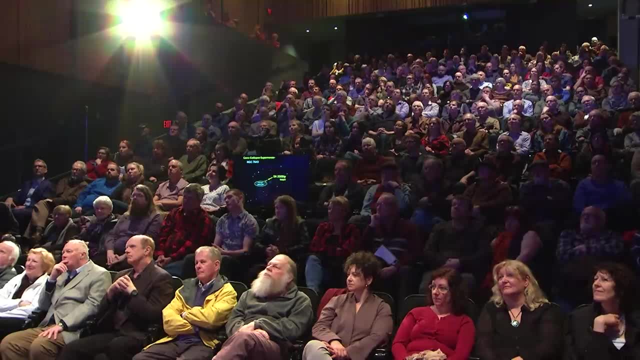 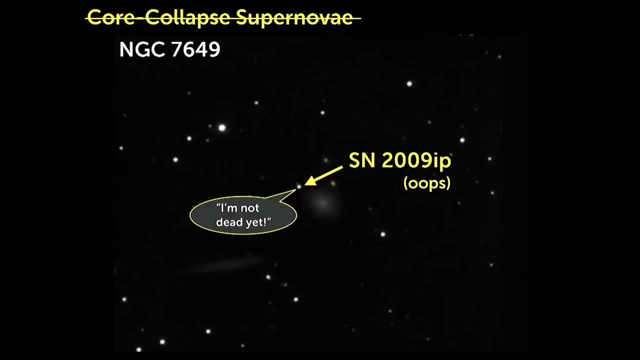 well, perfect, another supernova doing its supernova thing. Then it reappeared in 2010.. It reappeared again in 2011.. In 2012,, we finally saw a very dramatic eruption from this star, and we think that this star might now be dead. 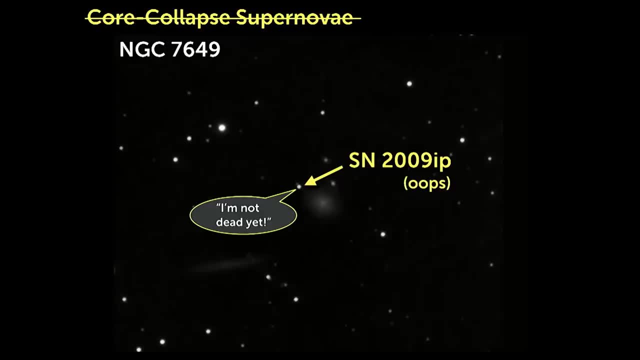 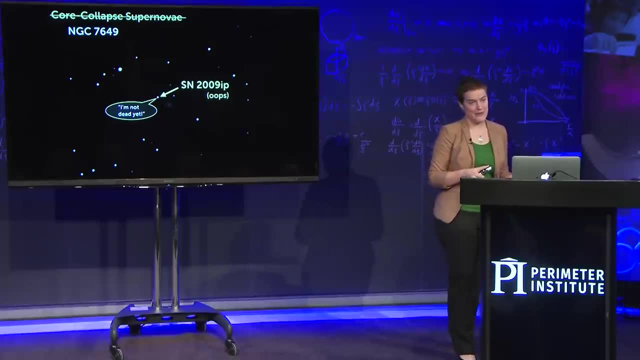 although people are still keeping an eye on it and looking here. just in case, This was an example of a star that, from our perspective, was just pretending to explode. What supernova 2009 IP actually is is an example of something called a luminous blue variable. 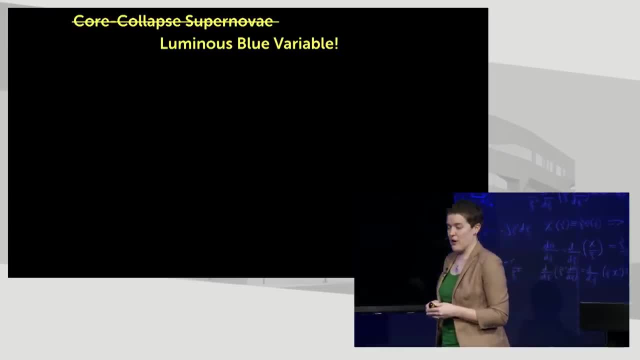 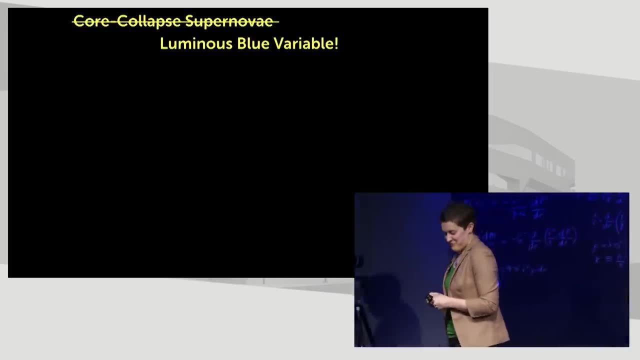 We tend to name things really literally in astronomy. We talk about red supergiants or our telescopes are named fabulous things like the Very Large Telescope. Luminous blue variable is very literally what these stars are. They're luminous, they're incredibly bright. 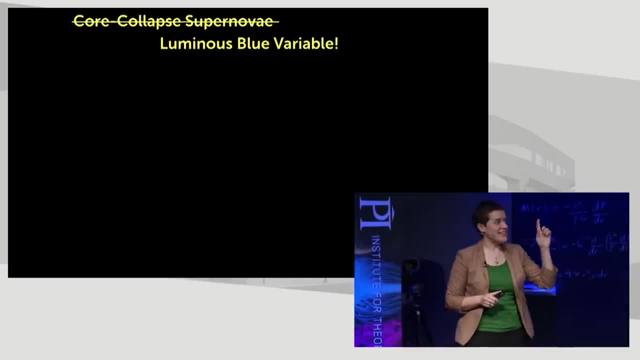 They're blue, which means a lot of the time they're very hot, and the key thing is that they are variable, so they change with time. A star like the one that produced supernova 2009, IP is variable because it's flinging off enormous amounts of mass. 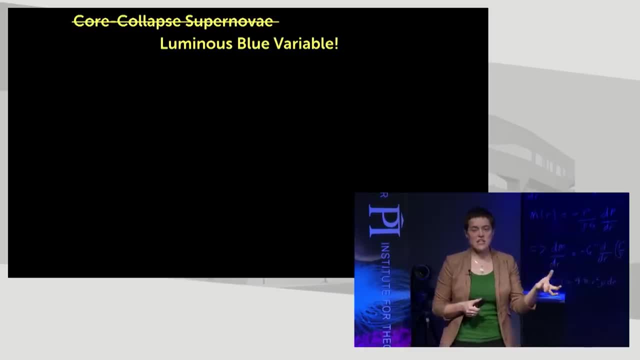 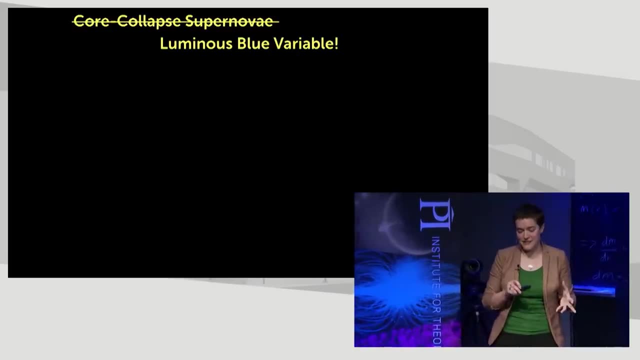 that appear to us as something very akin to a stellar explosion. What we're seeing instead is an eruption, and we still have a very limited understanding of what causes eruptions like that. We have an amazing example of this in our own Milky Way. 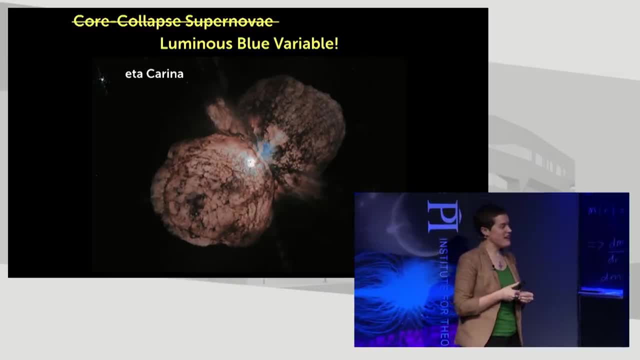 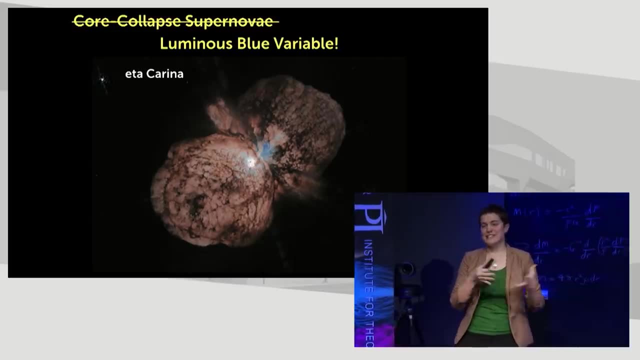 This is a photo of Eta Carina. It's about 7,500 light years away And if you look at that image, it looks like you're looking at something that exploded. It looks like the violent post-death of a star. 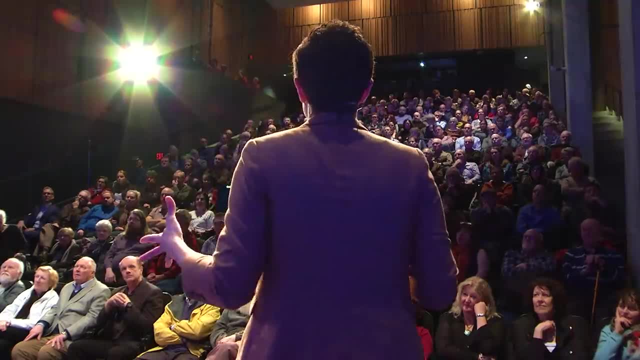 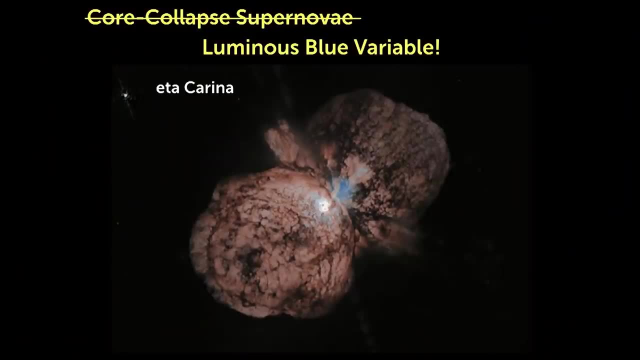 What we're instead seeing is material that got flung off of the star during an eruption in 1843.. When that eruption happened, Eta Carina got so bright that it was actually the second brightest star in the night sky for a few days. 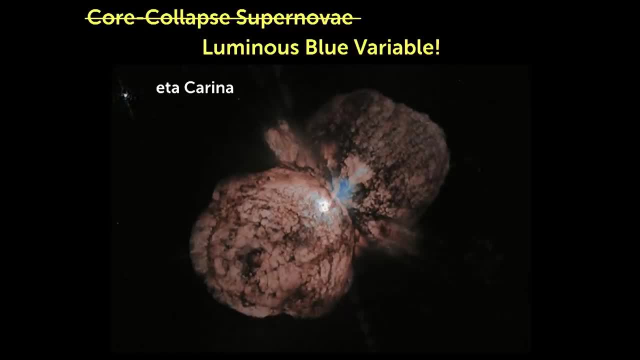 And it's faded away since then, But incredibly, the star is still in there. The star survived this explosion, And what we're left with is this very fascinating material from that eruption that we're still studying in the hopes of maybe trying to explain. 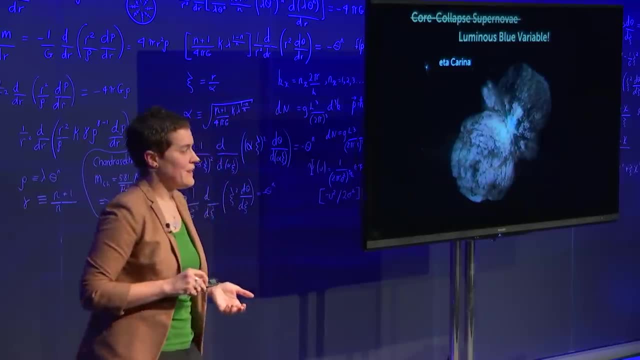 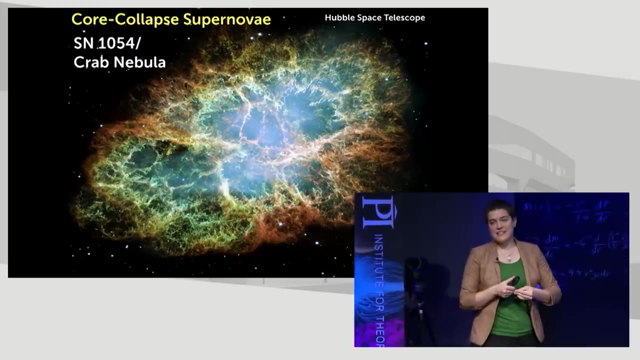 what luminous blue variables are up to. So I want to go back to the Crab Nebula, to this remnant of a supernova. I explained how a supernova happens. You have that collapsing core material tumbling down after it. 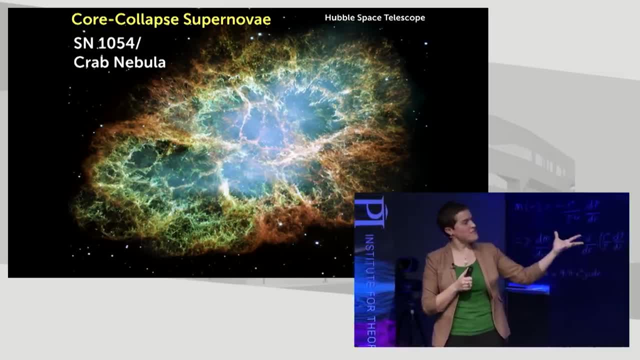 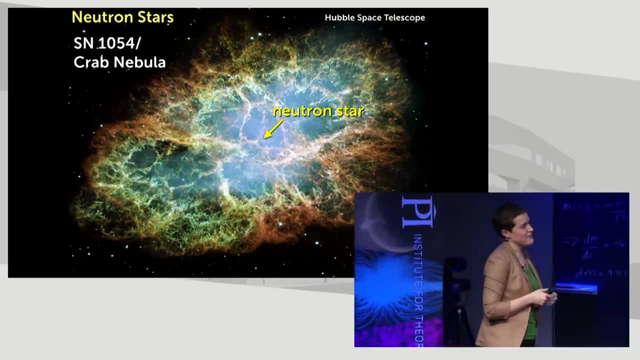 and giving us this explosion. The exploded material winds up, giving us something like a supernova remnant, like the Crab Nebula. But there's actually something else in here that's worth highlighting: At the heart of the Crab Nebula is something called a neutron star. 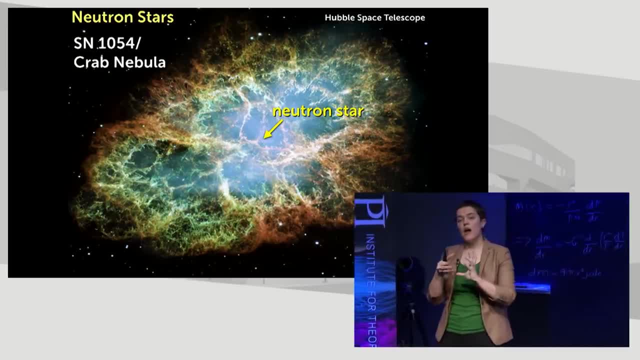 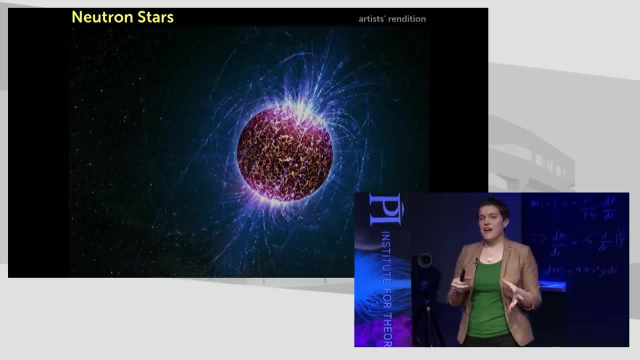 So a neutron star is what is left over when the core of a massive star collapses. Neutron stars are absolutely fascinating. They aren't working like the normal stars that I've described, these stars that have to fuse something in their cores to maintain a balancing act with gravity. 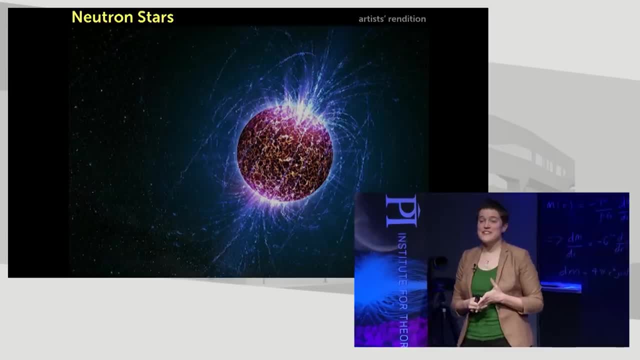 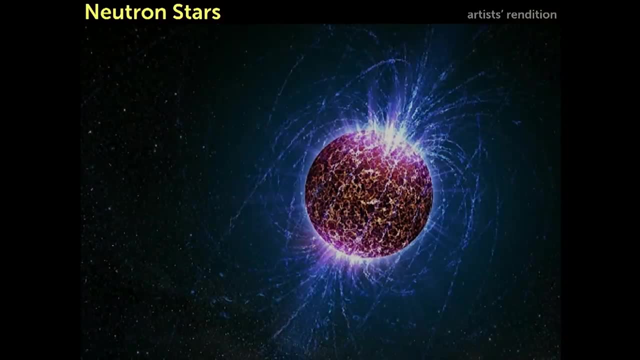 These stars are actually supported by principles of quantum physics. They're supported by something called neutron degeneracy pressure, hence why they're called neutron stars, And the basic principle behind this is that neutrons that are very similar to one another. they have similar quantum properties. 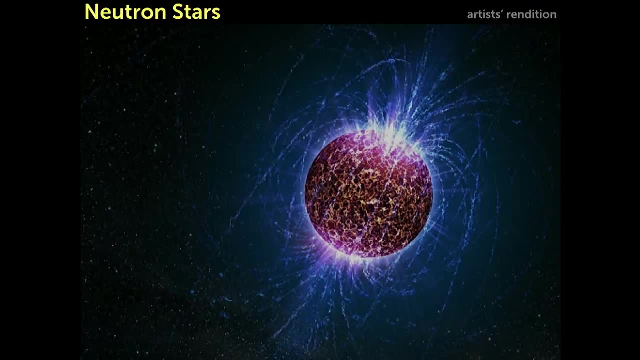 they occupy a similar state cannot be squeezed too close together. They will literally resist this to the extent that they're able to support themselves against gravitational collapse. Neutron stars are unbelievably dense and unbelievably small. One of these stars is the size of the city of Waterloo. 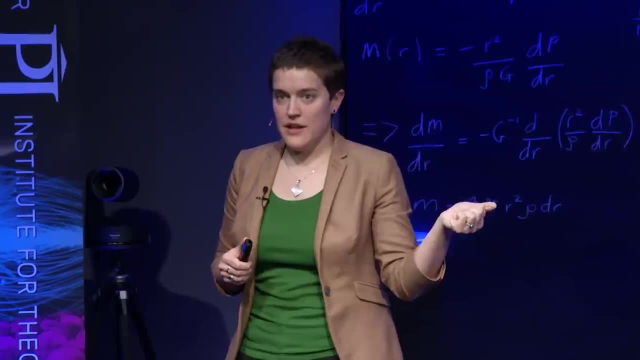 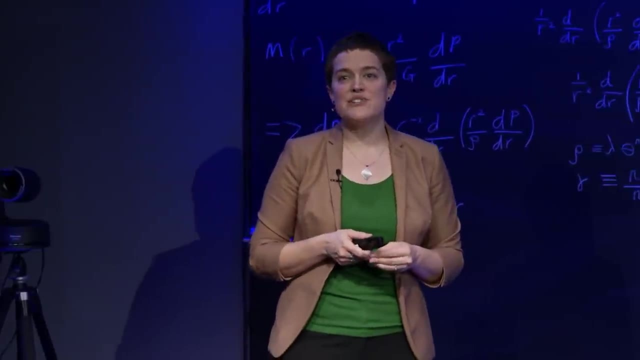 But if you took just one teaspoon of it, it would weigh more than a mountain. We're talking about a very extreme scenario in terms of the matter. in this star, You also sometimes see something interesting from a neutron star. This is an artist's rendition. 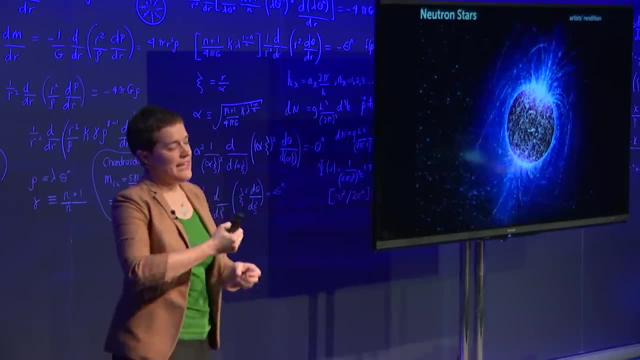 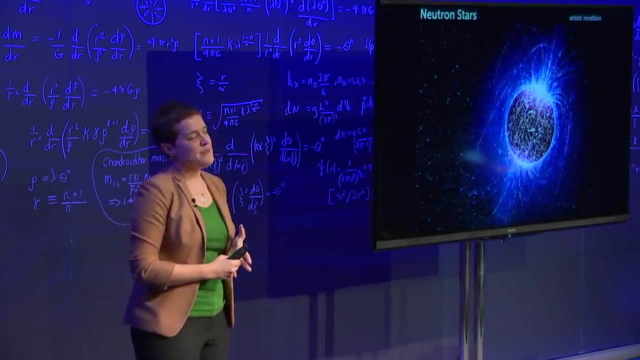 and you'll notice those lines sort of poking out of the star in opposite directions. Those are showing the magnitude of the magnetic field lines of the star and illustrating that some neutron stars can be what we call a pulsar. In some cases these stars will emit light. 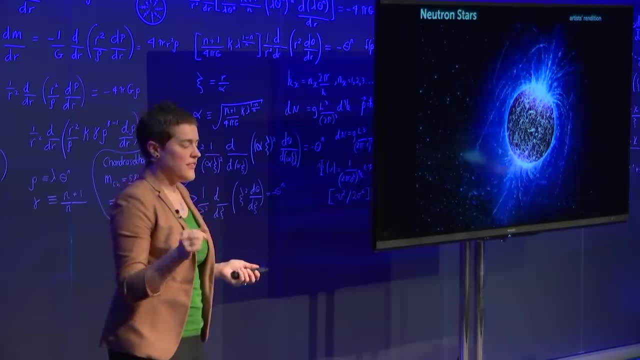 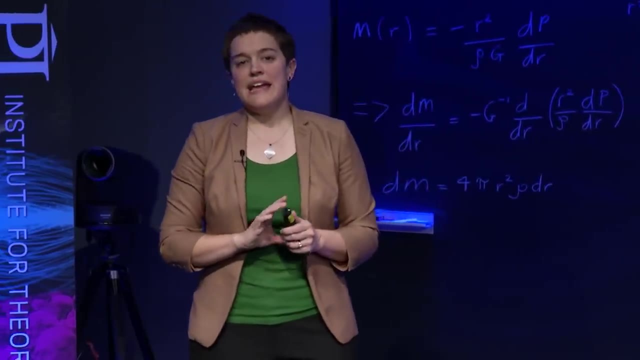 out of their magnetic poles. Now we know on Earth that our geographical pole, the actual pole that the Earth rotates around, is different than our magnetic poles. In an extreme case, like our neutron star, what you'll get is a beam of light. 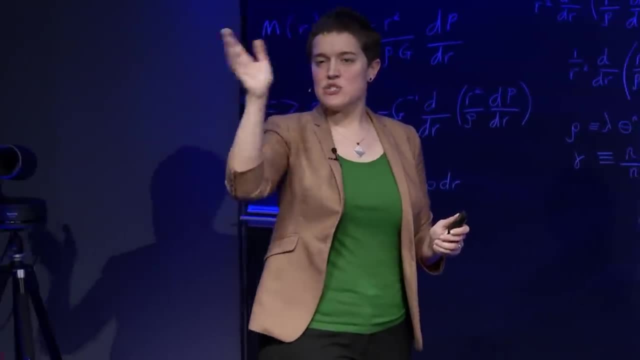 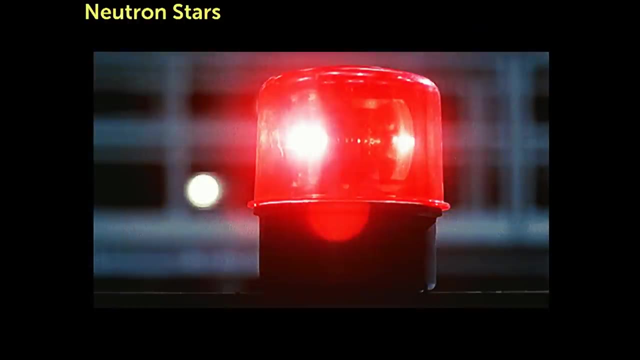 flinging around as the star rotates and sort of causing a flash as it goes by. The best analogy that I've been able to find is looking at something like an emergency light on top of a fire truck or a police car. Those are two beams of light. 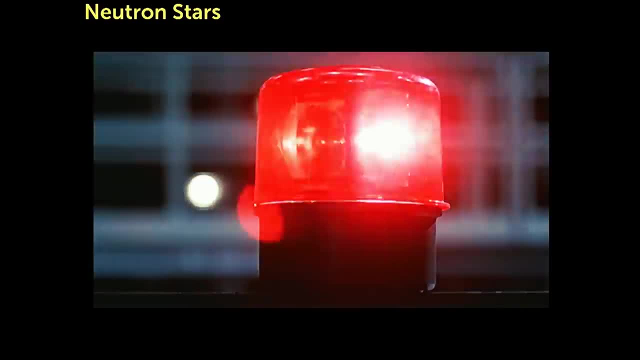 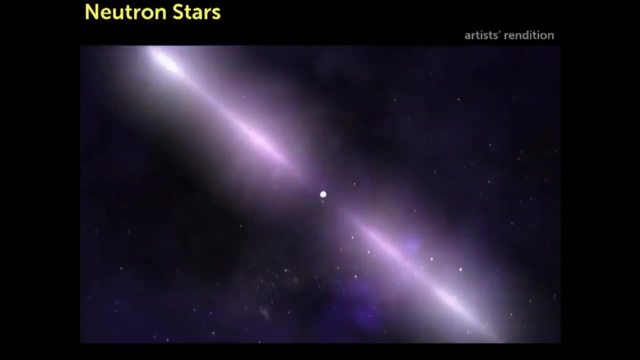 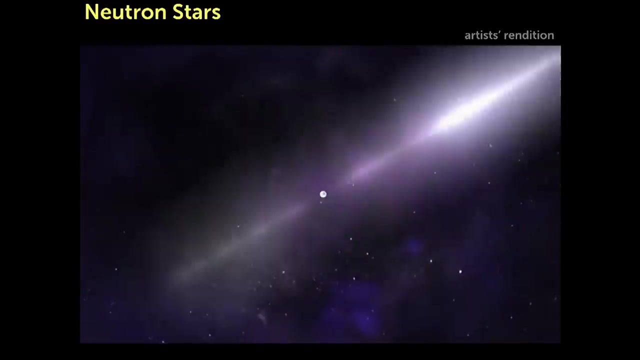 pointing out in opposite directions and as you spin it, it appears as though something is flashing. That flash is what we detect when we see something like this: a pulsar. Pulsars were actually discovered in a pretty interesting manner. They were detected by a woman. 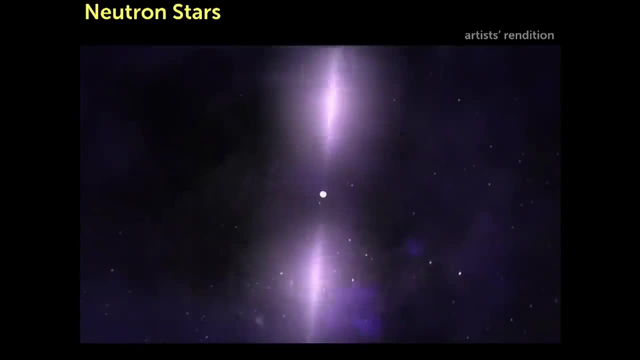 named Jocelyn Bell Burnell. in the 1960s in the radio She actually detected first one and then two and eventually got up to four objects like this. Their pulsations were perfect. It sounded like you were almost hearing a heartbeat from these stars. 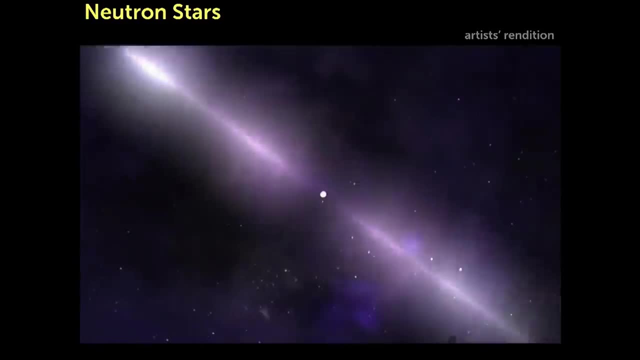 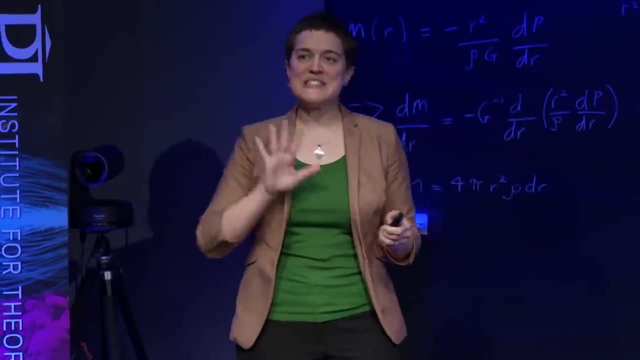 They temporarily nicknamed the objects LGM 1,, 2,, 3, and 4. And LGM was an abbreviation for little green men, And they were mostly kidding, But it was a sort of tongue-in-cheek nod to the fact that this was such. 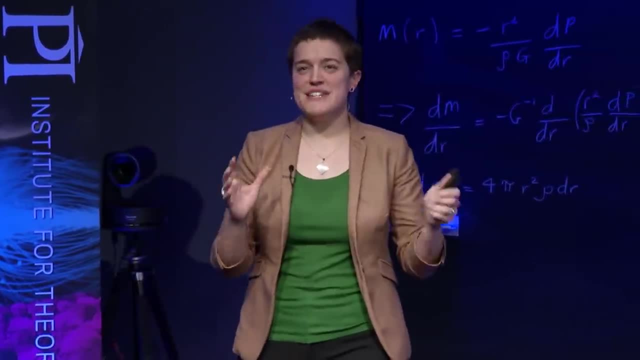 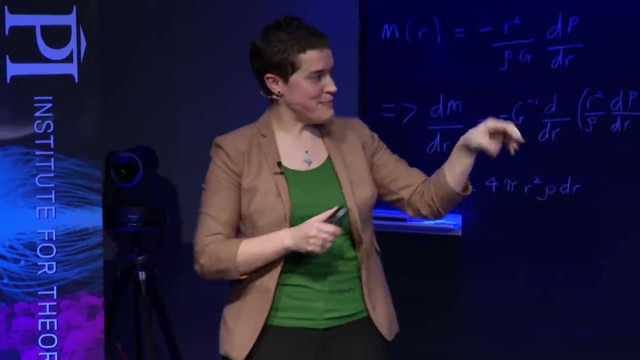 a perfect and regular signal that maybe, maybe somewhere, little green men were making this. It turned out that wasn't the case at all, and instead it could be explained by a neutron star that was specifically emitting this light and detectable as a pulsar. 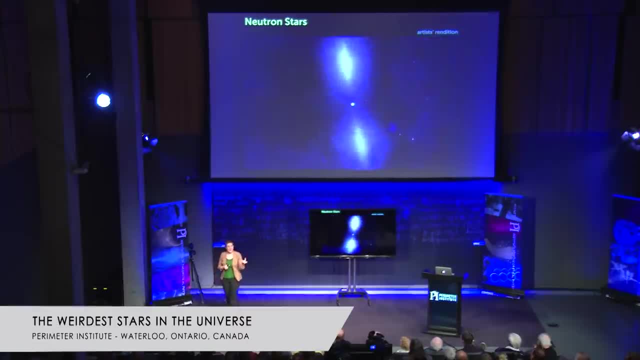 So I've talked about these neutron stars that can form when the core of a massive star collapses. If that collapse goes one step further, if we have more mass in the core, or if that neutron star gains mass with time, we instead produce something else. 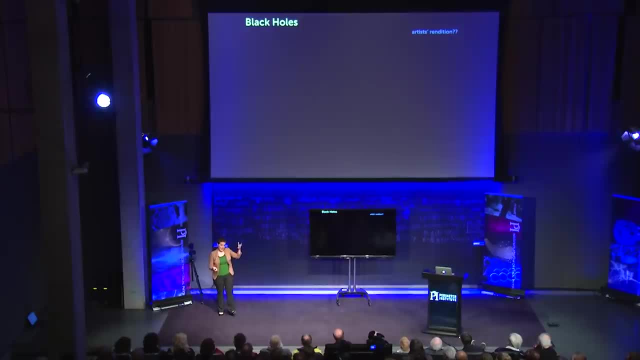 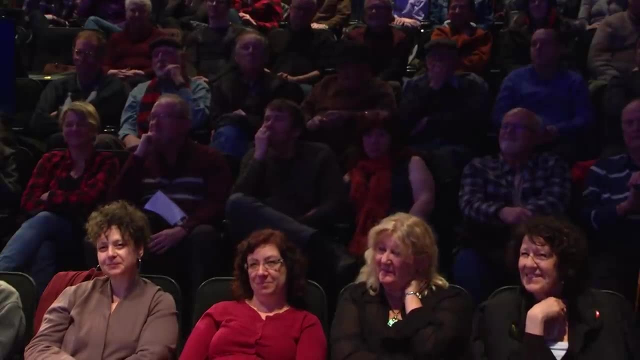 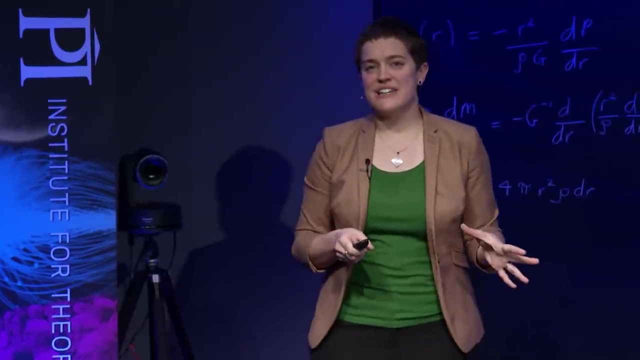 We produce a black hole. I apologize for the artist's rendition. You understand These stars will produce black holes as part of their deaths. Now, the black holes themselves are utterly fascinating, But what I'm particularly interested in are a subset of stars that actually 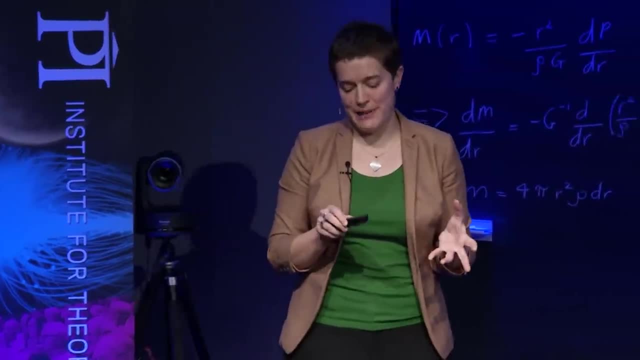 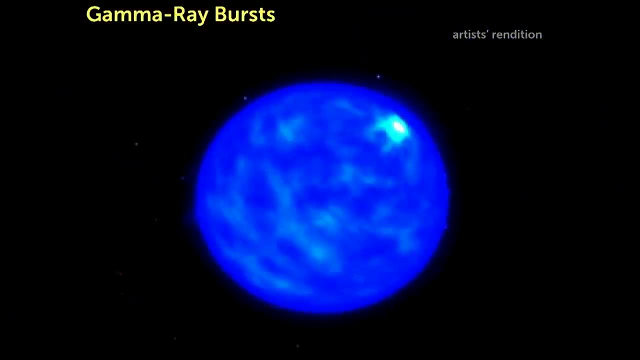 do something very strange. when they die and produce black holes, These stars produce something that we know as gamma ray bursts, And I have an animation of what this looks like. This is a massive star, something like 40 or 50 times the mass of our sun. 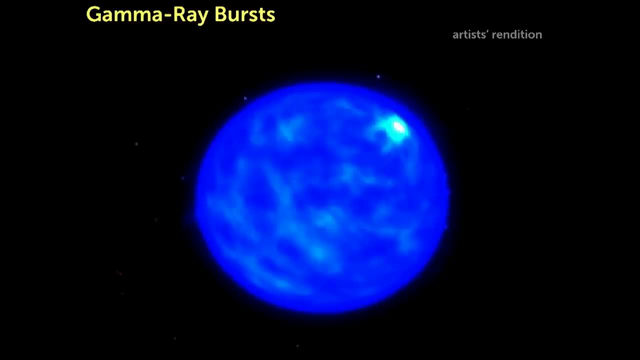 Now you'll notice. it's blue, It's not red. The outer layers of this star have actually been ripped off over the course of its life, exposing some of the hot inner layers. When this star dies, its core collapses into a very rapidly. 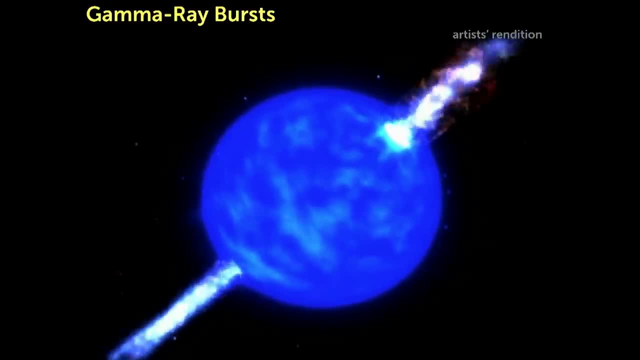 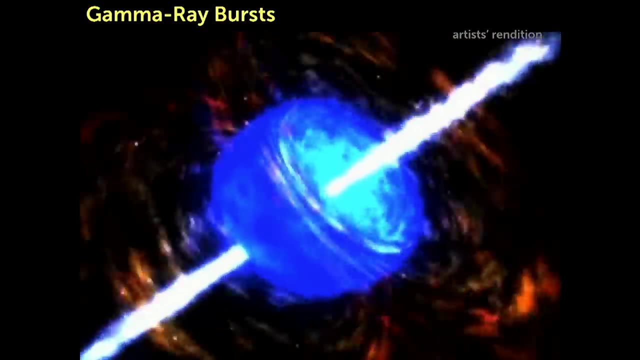 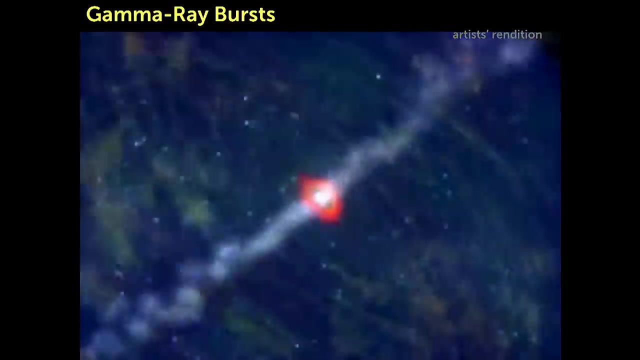 rotating black hole. That black hole starts consuming the star and almost shattering the star from the inside out. It's like high-energy jets of material shooting out. perpendicular to how that black hole is rotating, It consumes the star. collisions in those beams produce the gamma rays. 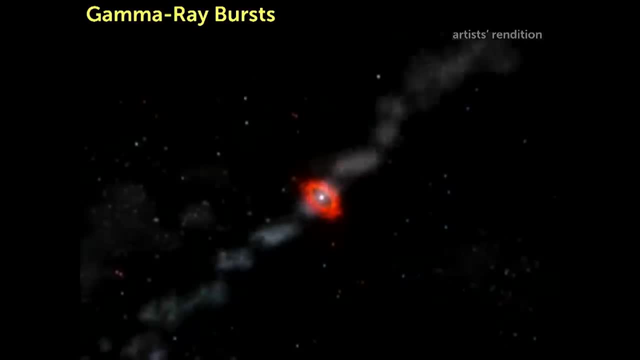 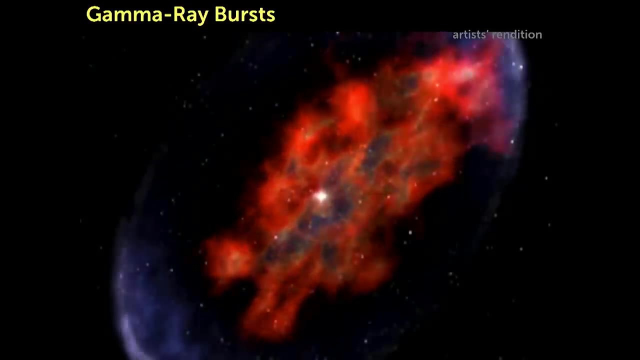 that we detect here on Earth and eventually the death of the star ends with the same sort of supernova that we talked about before. So that whole video took about 15 or 20 seconds. That was in real time A 40 solar mass star. 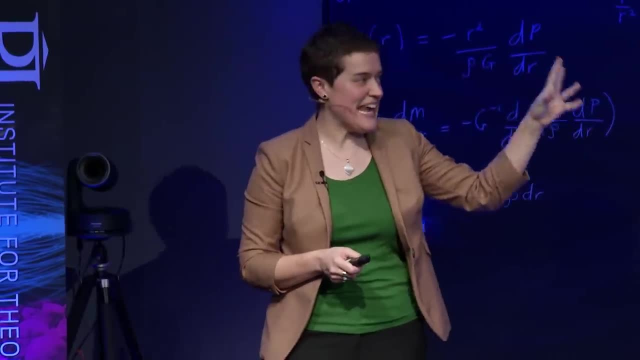 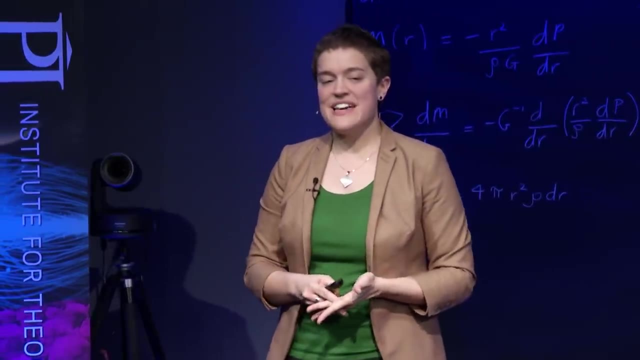 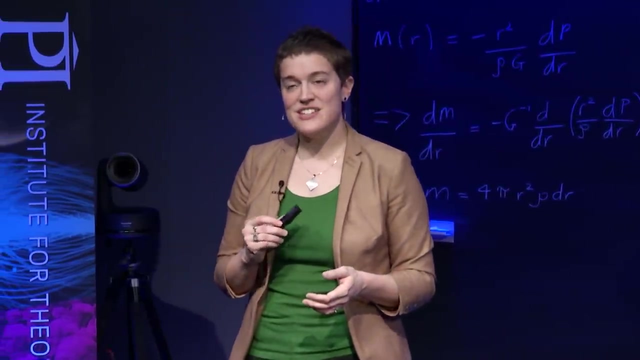 will actually die and produce a gamma ray burst in a comparable amount of time. So this is an incredibly violent death for a star. It's incredibly weird and that's an amazing timescale to work on for something that huge- Those flashes of gamma rays. 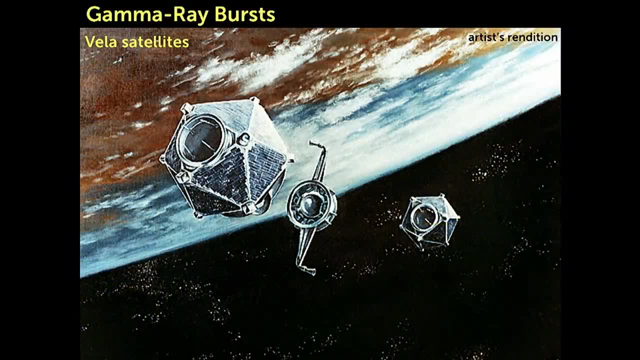 that we see from stars like this were actually discovered by accident. So these are the Vela satellites. It's a sketch of these satellites that were launched in the mid-1960s following the signing of the Nuclear Test Ban Treaty. These satellites would orbit the Earth. monitor the planet and look for signs that somebody was violating the treaty and performing a nuclear test which would have shown up as a flash of gamma rays. The satellites worked great and they detected many flashes of gamma rays And fortunately for world peace. 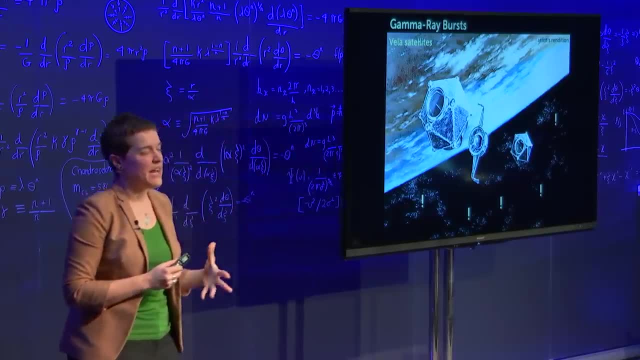 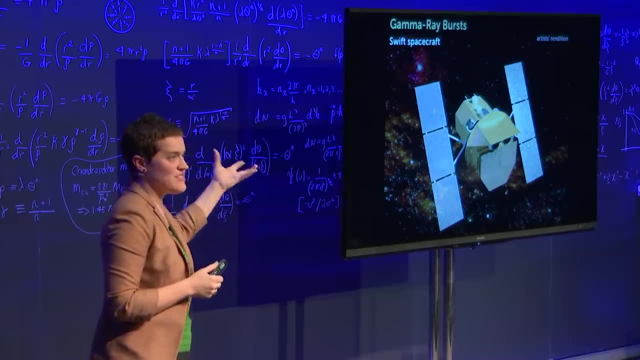 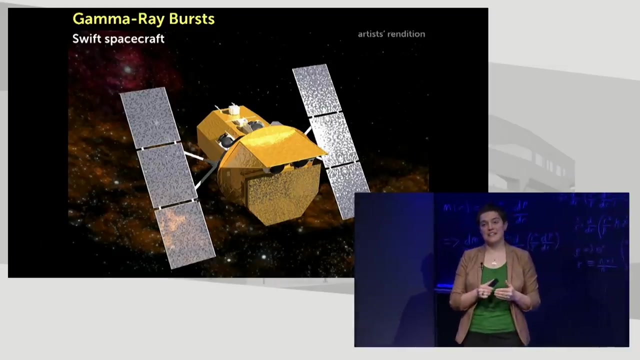 none of them were coming from Earth. Instead, they were coming from all over the sky. It took us a long time to detect these flashes, But what we finally determined was that we were seeing flashes of these dying stars from other galaxies. We've now put up dedicated telescopes. 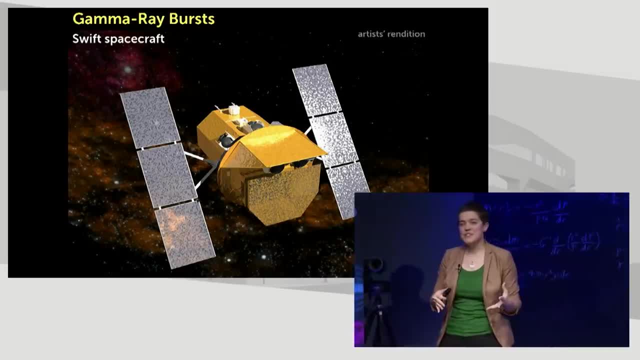 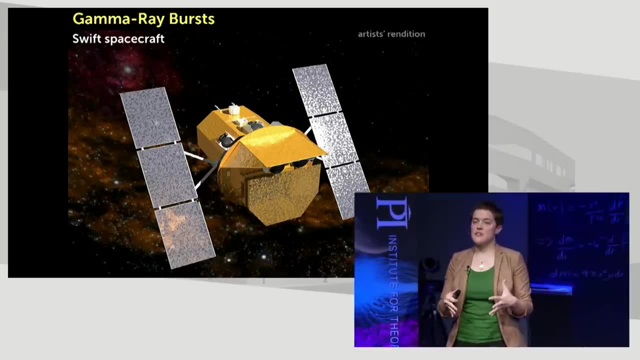 whose job it is to look for gamma ray bursts and to tell us when one has happened as quickly as possible so we can try and study them. So this is the Swift spacecraft. It's a tailored telescope for detecting these sorts of gamma ray flashes. 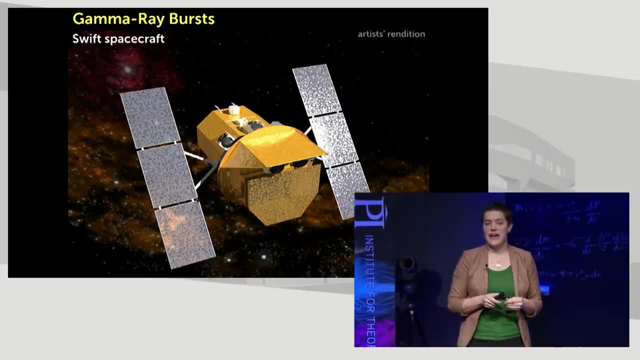 That flat panel that you see on the front is a gamma ray detector And then, under what looks like actually a sun shield, are X-ray and ultraviolet and optical telescopes that try to observe these objects as fast as possible. What Swift will do is it will sit there. 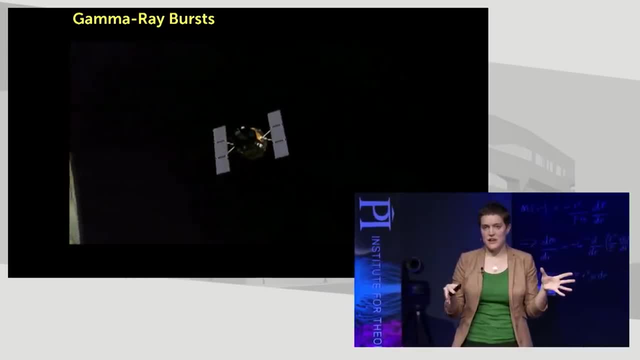 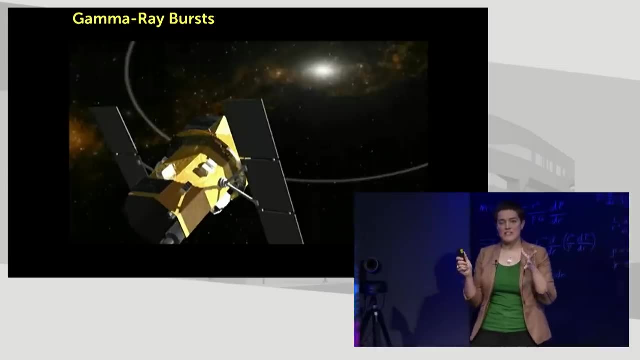 orbiting the Earth waiting for a gamma ray burst to go off somewhere in its field of vision. It'll spot a gamma ray burst out the corner of its eye. go, oh my god. turn and start taking data on the gamma ray burst. 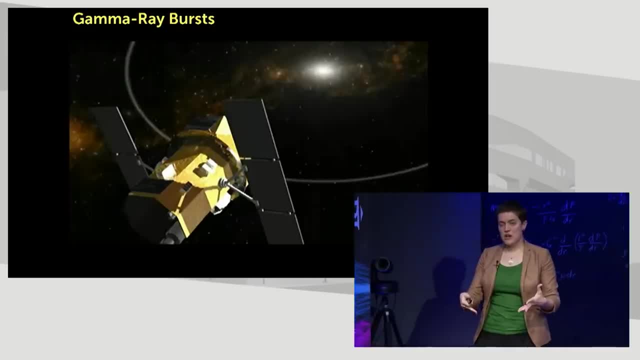 as quickly as possible. When it does that, it sends a notification down to Earth, to astronomers, saying a gamma ray burst has just happened. It lasts 20 seconds. We see light from these events in other wavelengths, but they still don't last very long. 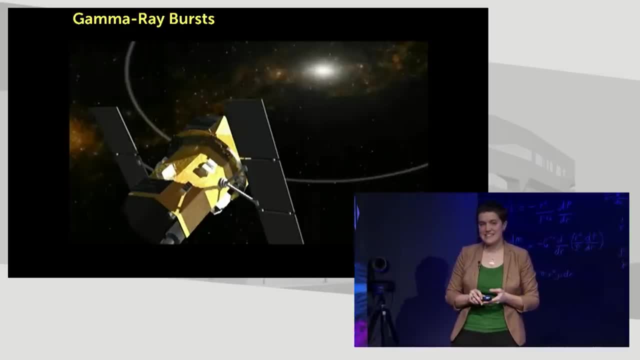 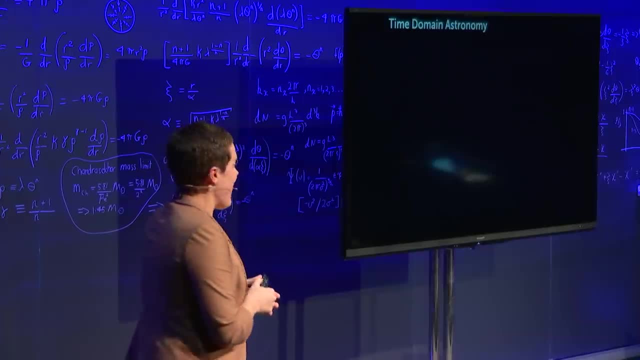 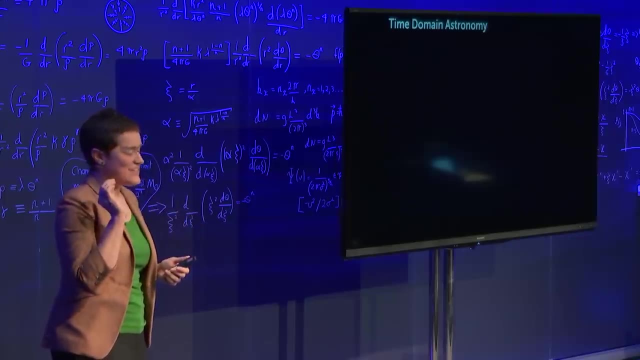 So there's a great reason to try and go after these events and study them as quickly as possible. So this gets into a type of astronomy called time domain astronomy. I love this discipline. It focuses on trying to study things that are very fleeting and very quick. 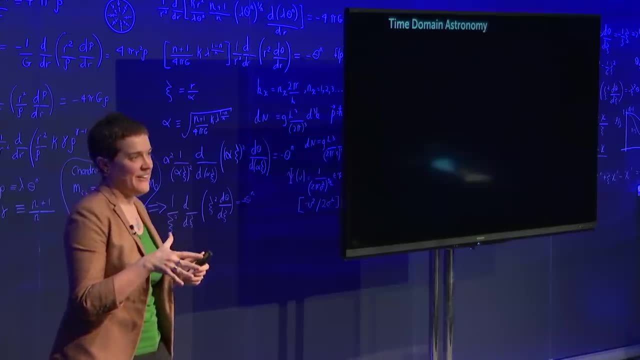 It's the closest, I think, that we get to sort of movie-style astronomy. So I want to do a quick comparison between how a movie might depict time domain astronomy- detecting a gamma ray burst and having to chase it very quickly- versus how it actually happens. 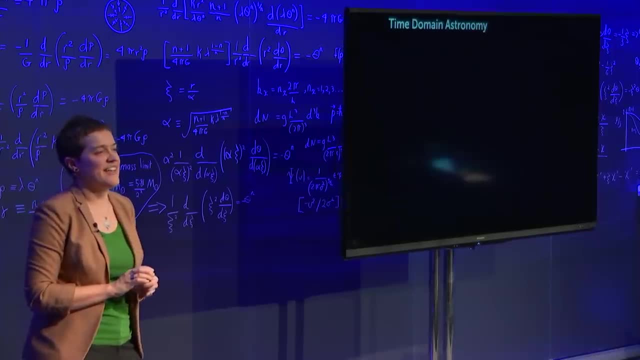 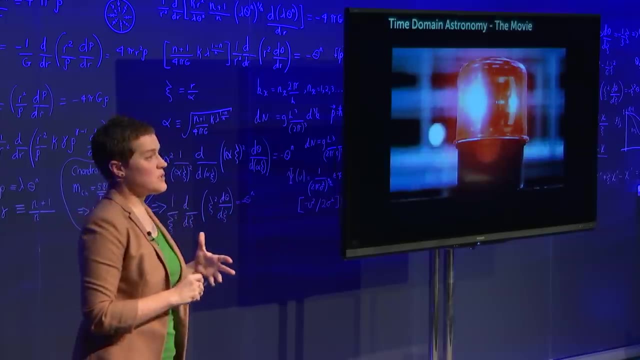 I would contend that I think the way that we actually study these could be more interesting than a Hollywood film. But in Hollywood, if you detected a gamma ray burst and you wanted to do something very quickly with it, the detection would be announced by the science siren going off. 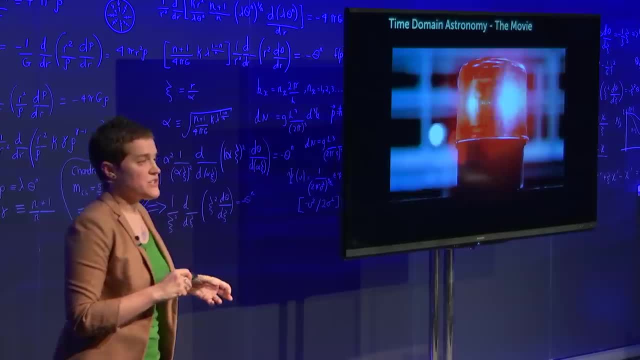 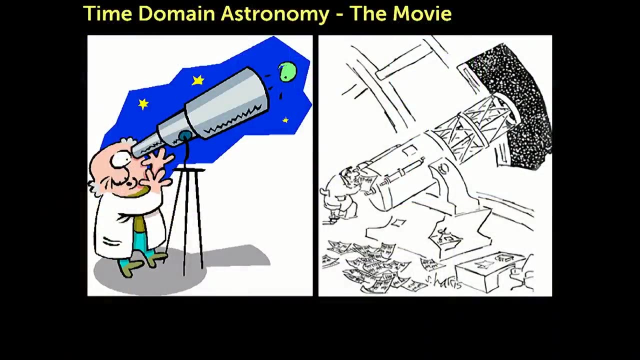 For some reason, this is always a very public and very easy thing to do. Astronomers would get this notification that something exciting happened. They would run to their telescopes wearing lab coats. for inexplicable reasons, They would look through the telescopes with their eyes. 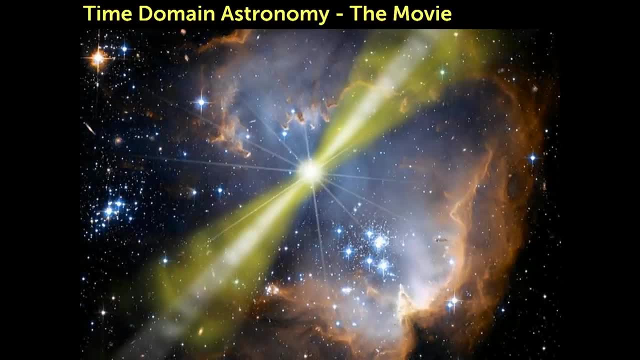 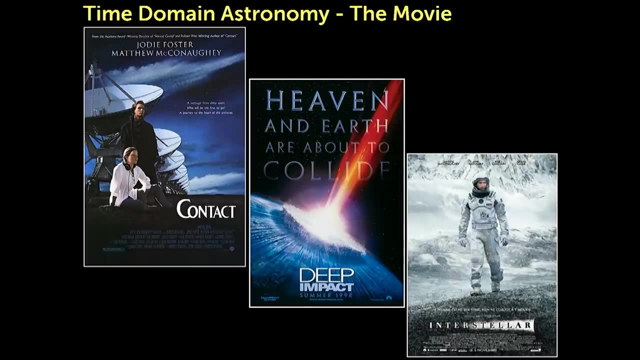 and they would naturally see something like this. They would see perfect, beautiful, colorful data. They would realize that something that they had observed would help them to save the world. They would dash off to talk to aliens or stop an asteroid or find a new home to live on. 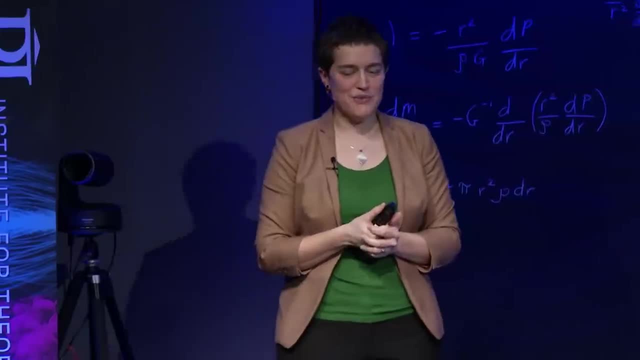 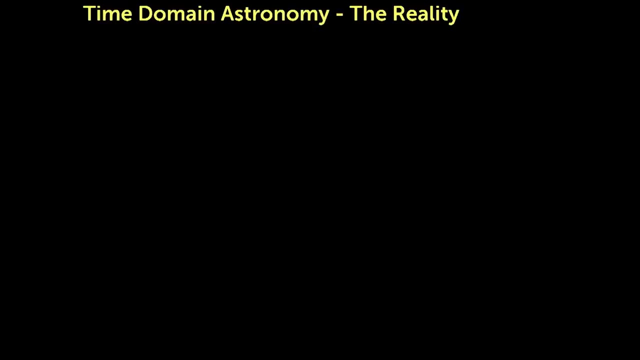 And that tends to be how the movie goes. The reality is a little bit different, but I think some of the things that we do are more fun. So, in reality, a science siren does not go off when a gamma ray burst is detected. Instead, 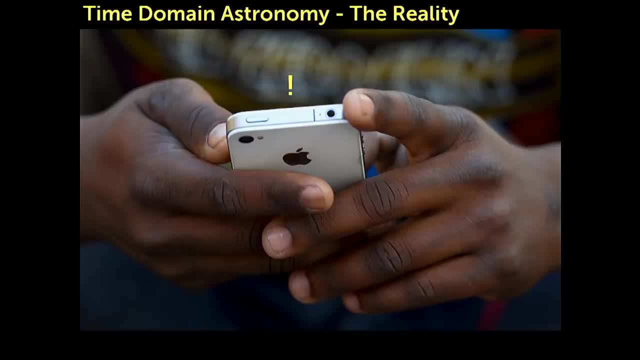 you get a notification on your phone, You will see a text alert or an email. There are astronomers who are signed up specifically to get notifications if something this exciting happens. Once that happens, the astronomer holding the phone gets to go alright. 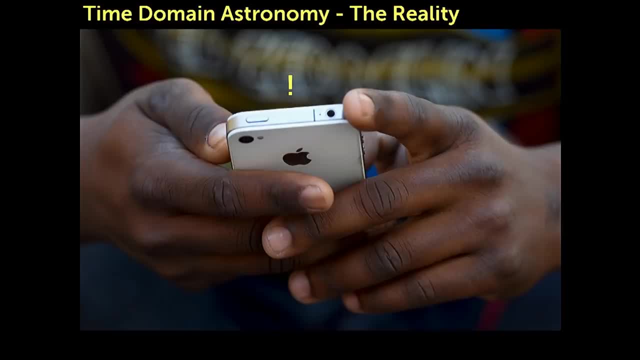 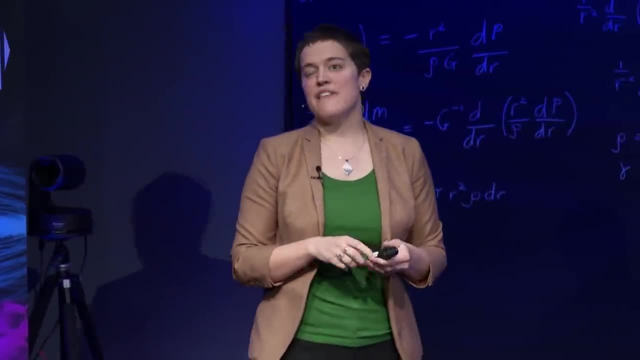 we have now triggered something called a target of opportunity. There's something that's happened in the sky that we want to follow up as quickly as possible with the best telescopes possible. They will have access to something like the Keck 10-meter telescopes. 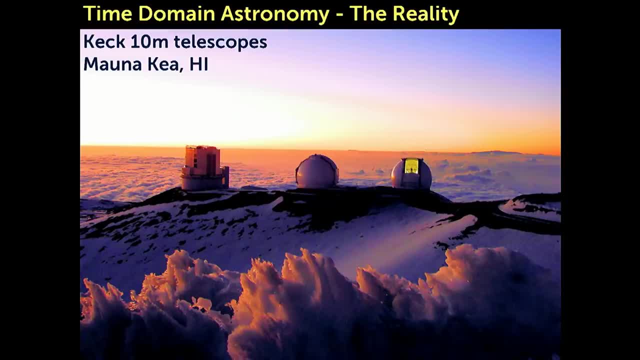 which are on the summit of Mauna Kea in Hawaii. They will contact these telescopes and say: you have to stop whatever you're doing. I'm sorry astronomer who is doing their own science. You have to stop whatever you're doing and take a little bit of time. 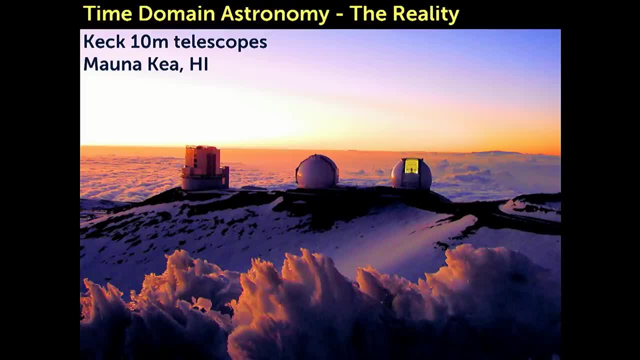 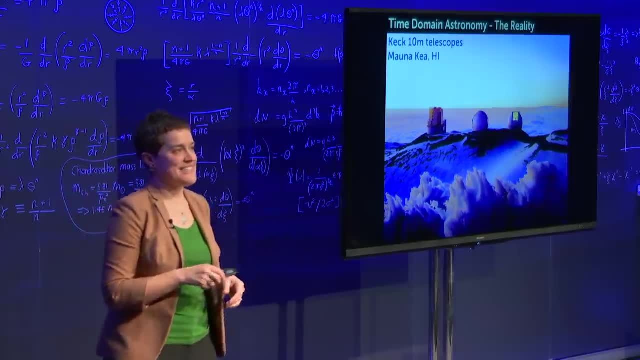 to observe this object in the sky very quickly, before our chance goes away. I think that these telescopes are unarguably cooler than the lab coat and eye version that you might see in a cartoon or a movie. To give you a scale of what a 10-meter. 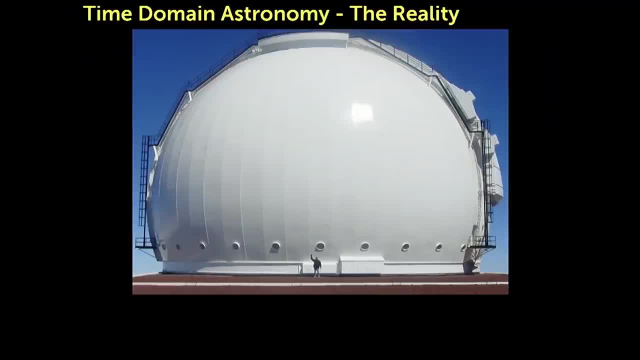 telescope looks like. that's an about 6-foot tall person standing in front of one of the two Keck telescope domes. You'll call in, you'll trigger this observation and you hope that the night looks like this. You hope that it's. 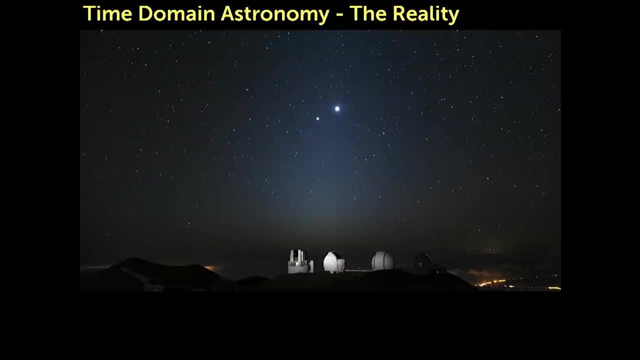 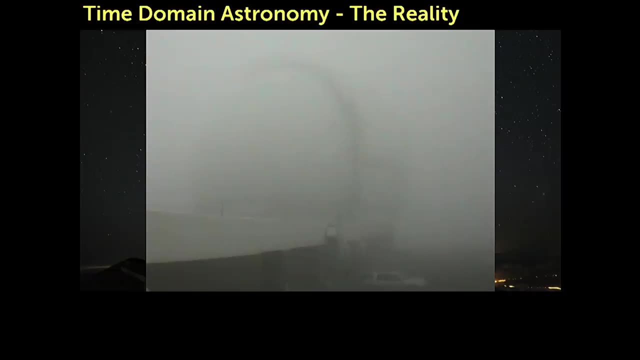 beautiful and clear and you can get amazing data of whatever you're wanting to observe. The night might look like this: This is an actual photo that I took when I was trying to observe at Keck. when you can't see the building, that's like 30 feet away. 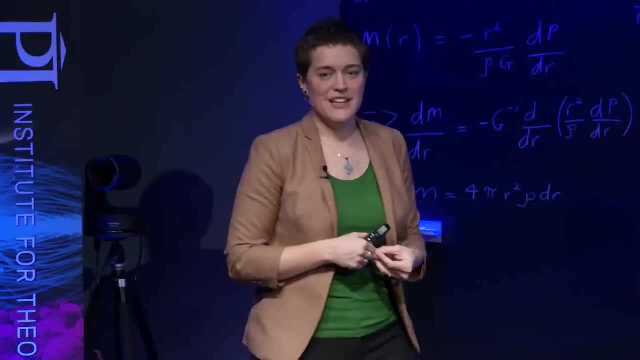 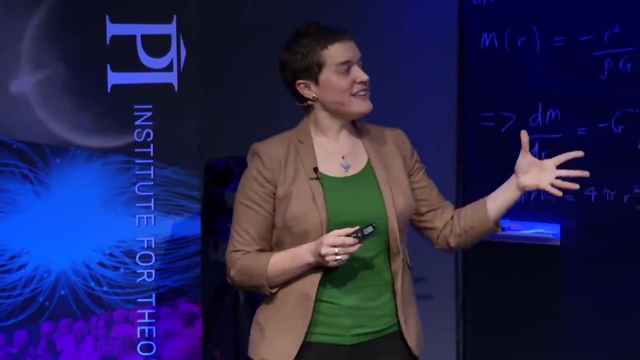 Your odds of detecting something in deep space are getting really bad. You can't even open a telescope when it's this crummy out. It's unsafe for the telescope and the instruments. Hopefully the weather is clear. you take observations and you get gorgeous data. 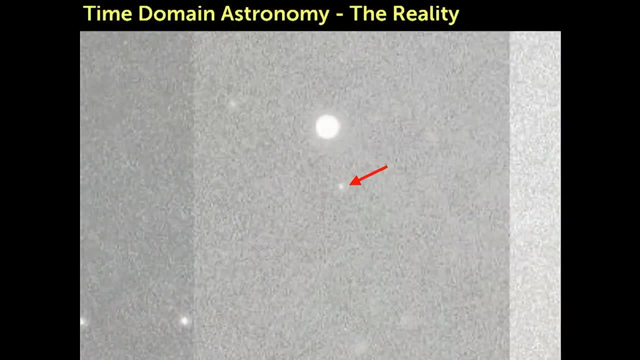 This is beautiful data and, by the way, that's the thing you're looking at. The bright object up top is something else in the way. There's a lot that has to be done to data before it can be finalized. You have to account for things like the background. 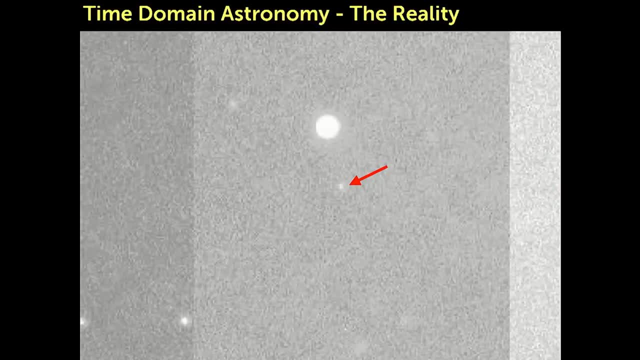 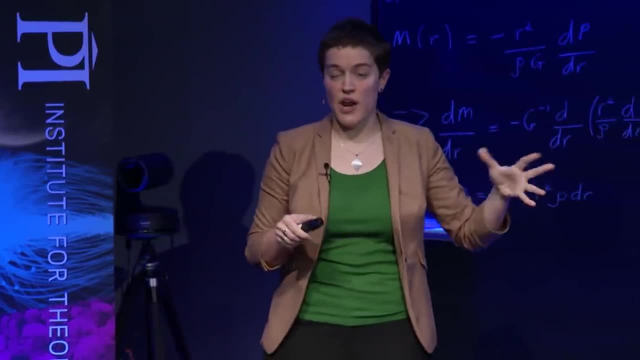 glow of the sky, electronic noise from the instruments on the telescope. There's a lot of effort that goes into eventually turning this into science. Once you have a discovery, you don't run off and call the president and save the world. You wind up posting your results. 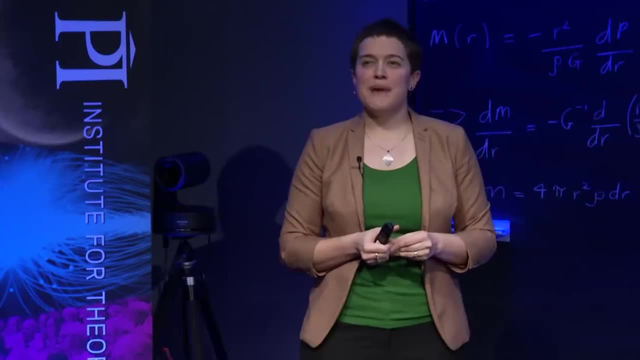 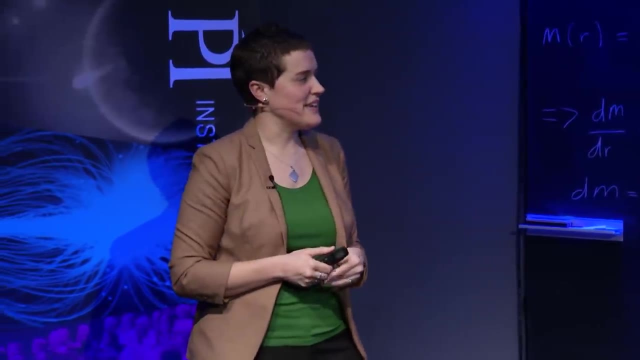 in some form of scientific publication. Something might be pretty quick. You might just want to say: we got a little bit of data on a gamma ray burst or on a supernova, so you'll put it on something like the Gamma Ray Burst Circulars. 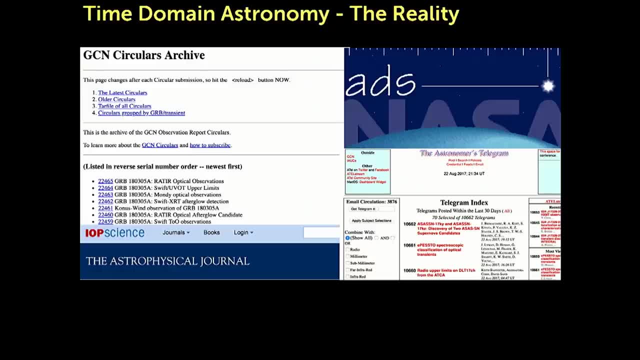 Network on the upper left, Or the Astronomer's Telegram, which is now a website on the lower right. You might write a research paper for something like the Astrophysical Journal. You'll put those papers on a public paper repository. This is how we tend to. 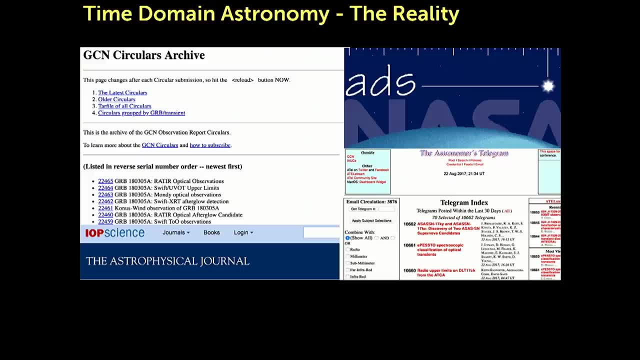 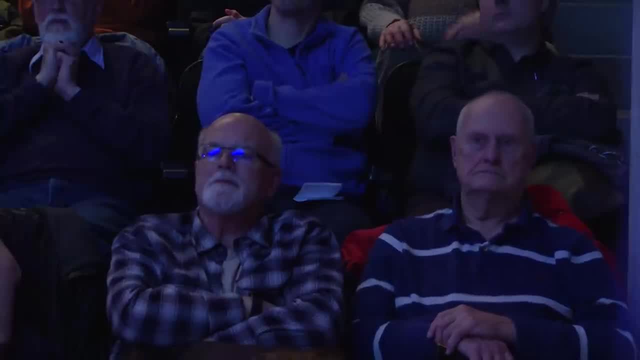 spread our results around. We'll work on something, we'll analyze the data, we'll very carefully, get to an end result and then we spread it around to the community. Astronomers can sometimes still be amazingly fast at doing this, But it winds up being a much more controlled. 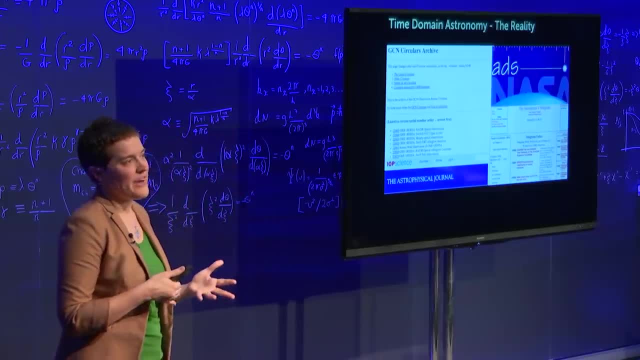 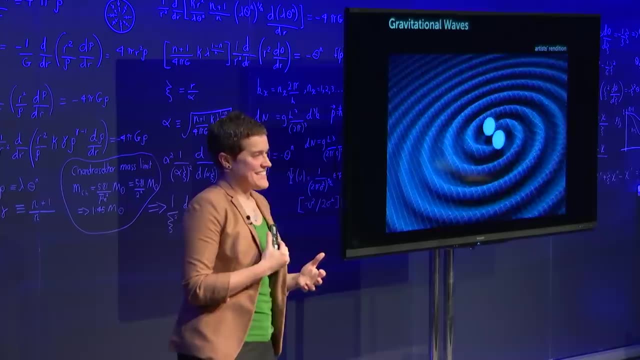 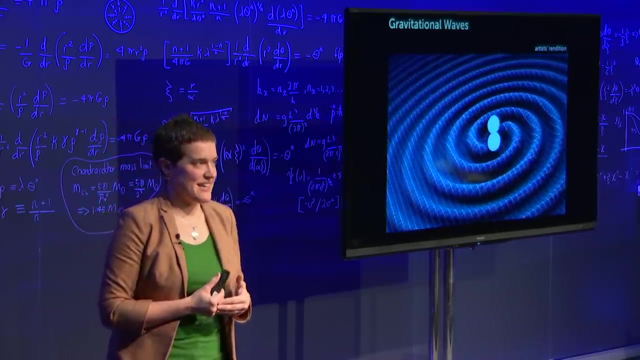 way to do the science and it ensures that a lot of what we wind up seeing is both incredible and accurate. I think my favorite recent example of target of opportunity and time domain astronomy was related to gravitational waves. I'll start by briefly explaining what gravitational waves are. 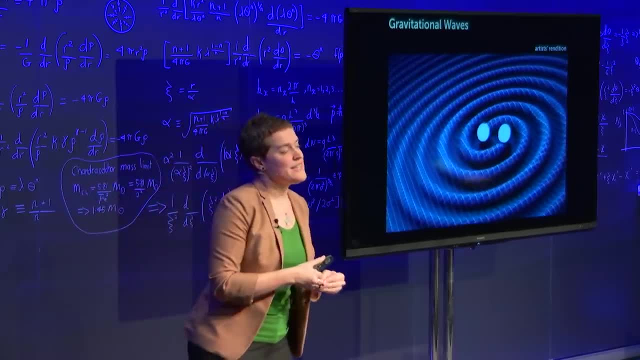 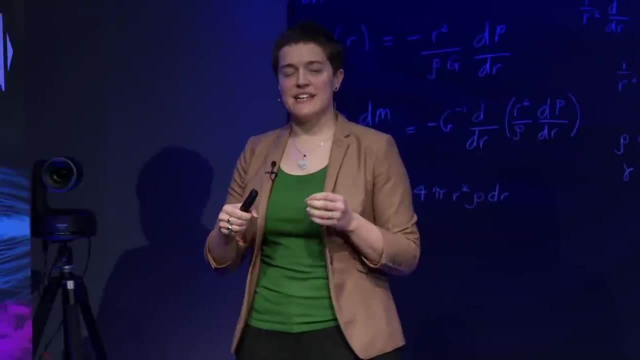 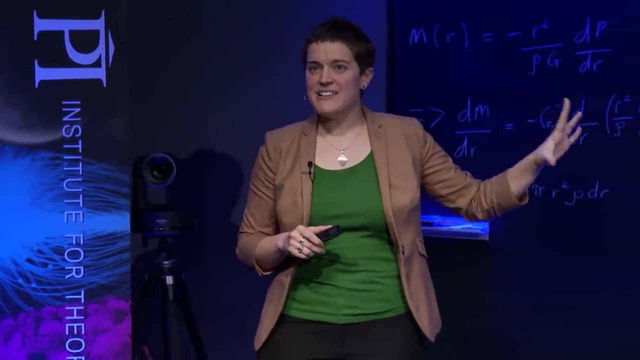 A lot of you probably recognize this animation. This animation came out when the first discovery of gravitational waves was announced in early 2016.. It detected gravitational waves from two black holes that were colliding. This animation was everywhere. It's excellent, but I like to use 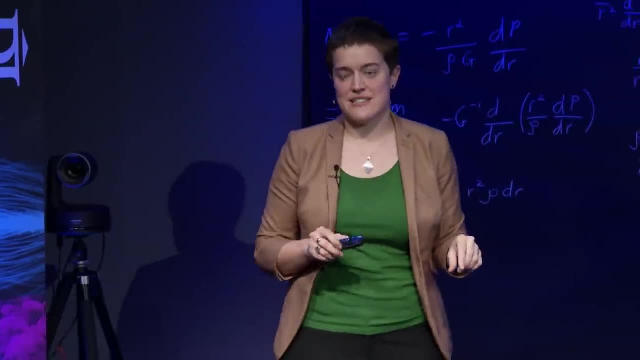 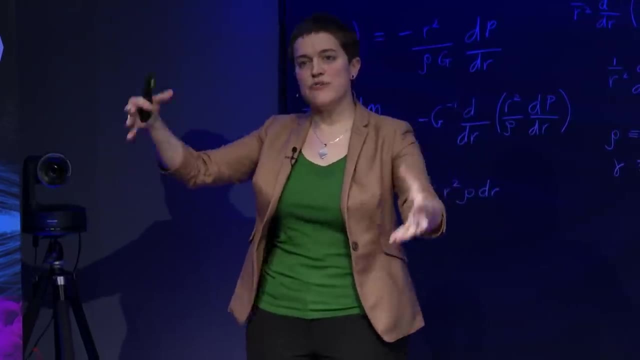 something a little bit different. to understand what a gravitational wave actually is, I want you to imagine that you're holding something like a slinky. If you look at the slinky between your hands, there's at least two different ways that you can cause a wave. 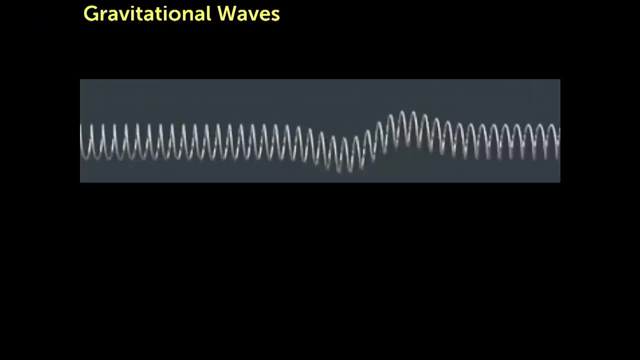 One is the obvious one: You take that slinky, you lift one end and you watch the wave propagate from one end to the other. Gravitational waves aren't quite this. These are waves traveling through space-time. What they're doing is something more. 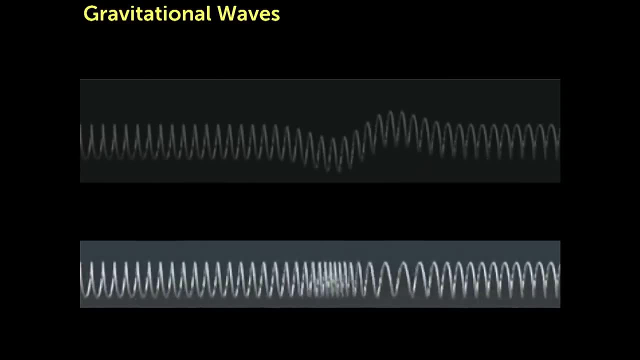 like a compression wave. If you took the slinky and shortened one hand and kicked off something like this. those compression waves travel through space-time and impact space-time along the way. When a gravitational wave reaches Earth, we see something like this: This is a 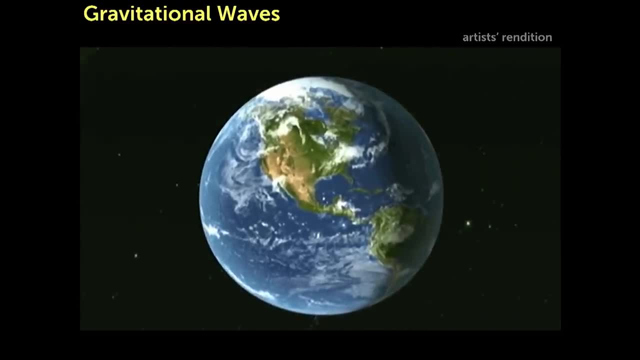 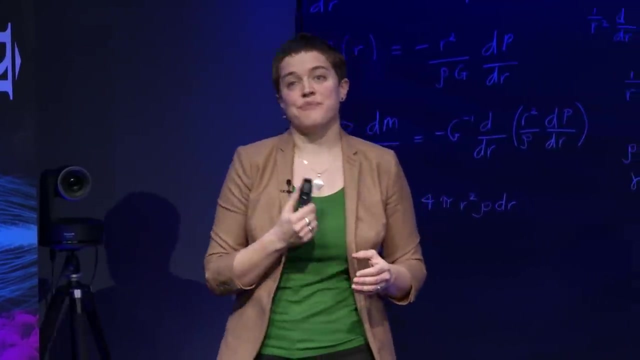 wildly exaggerated effect, but you can see Earth getting squeezed and then stretched as a gravitational wave propagates by and squeezes and stretches the space-time that Earth is in. We take advantage of that squeezing and stretching effect to detect gravitational waves. This image is LIGO. 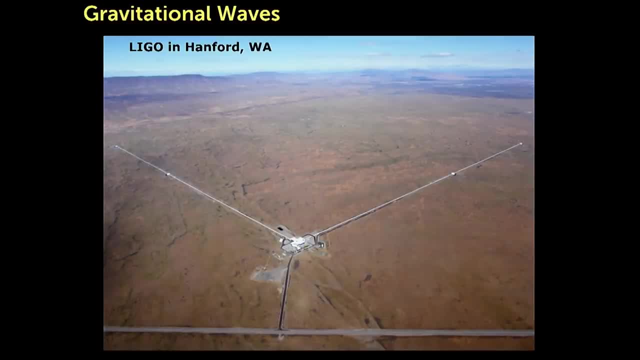 This is the Laser Interferometry Gravitational Observatory in Hanford, Washington. There's three of these in the world. There's one in Washington, one in Louisiana and one in Italy. They're all specifically designed to detect gravitational waves. 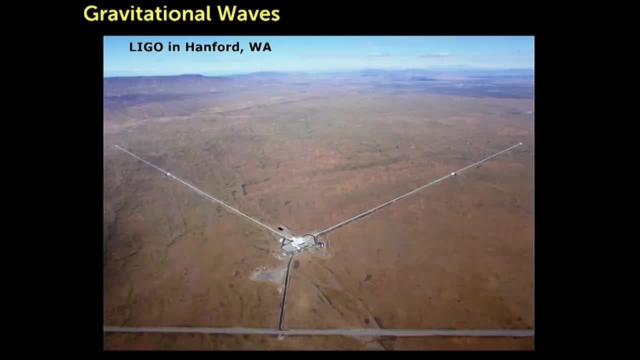 They consist of these two arms set at perfect angles to one another. Each of those arms is exactly four kilometers long. There is a laser and a beam splitter in that central building. What you can do on a normal day, on a day when there is not a gravitational wave, 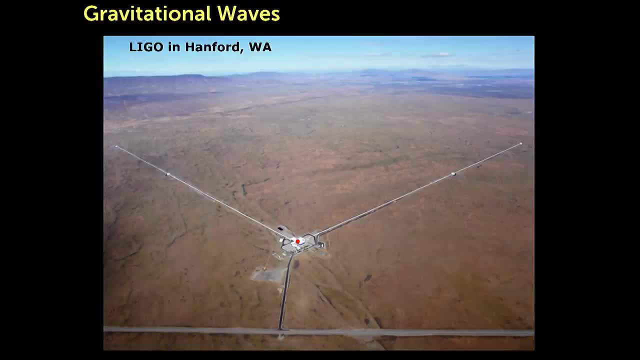 is fire a laser beam. using the beam, splitter down both of those arms at once, With each arm being exactly four kilometers long. the laser will travel. the length of the arm will be reflected off a mirror at the end come back and the two laser 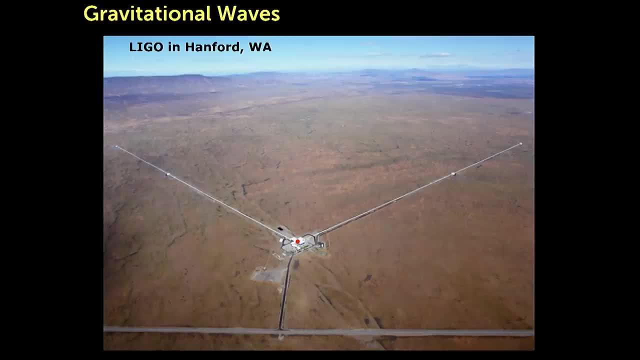 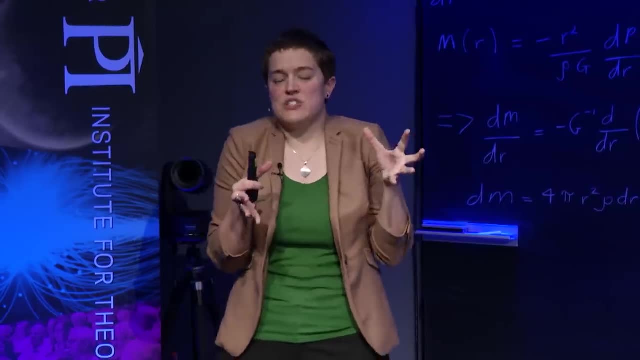 signals will have traveled the exact same distance in the exact same time. They'll cancel each other out and you know, okay, there's no gravitational wave. Now imagine a gravitational wave actually happening and squeezing space time and squeezing the detector. What I've just done is squeeze the 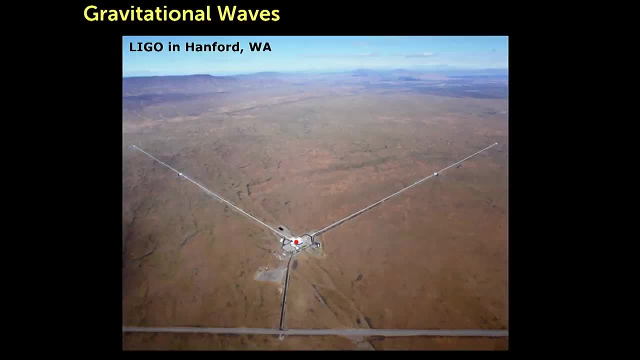 picture, so that the arm on the left is now a little bit shorter. Now, if you send lasers along those arms, they will arrive at slightly different times. The one on the left had a slightly shorter trip than the one on the right because of the 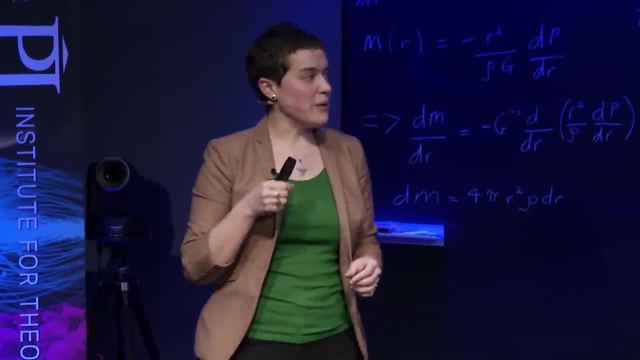 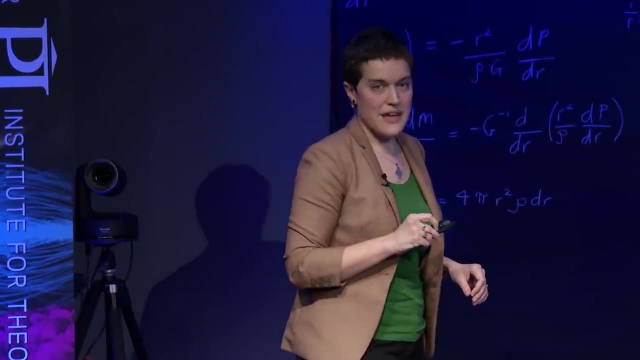 effects of gravitational waves. We now see a signal and we can confirm that we've detected a gravitational wave. This started out by detecting two colliding black holes, but last year, on August 17th, we detected something else. So these are. 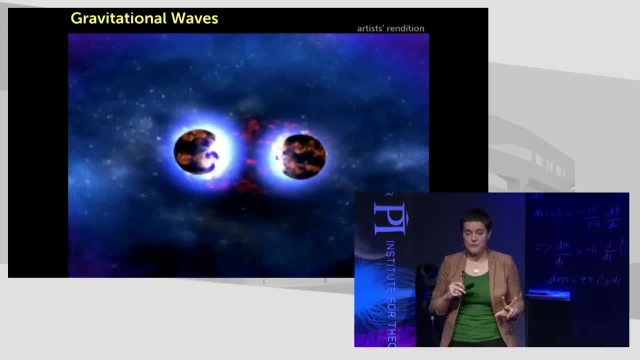 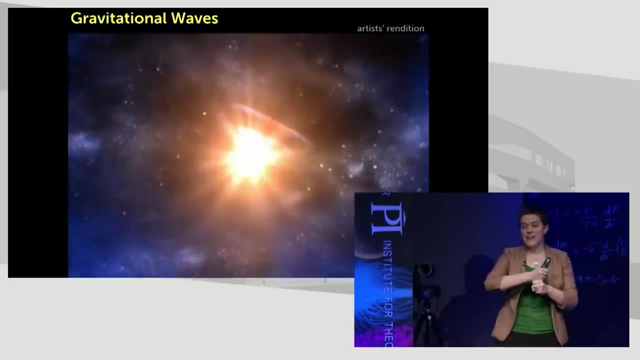 two neutron stars, the same stars that I talked about before. They're orbiting one another in a very close binary. They're spiraling in, spiraling in, getting ready to collide. When they collide, they emit a very short flash of gamma rays, even shorter. 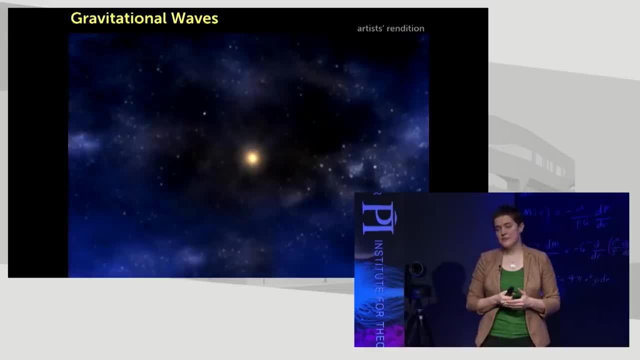 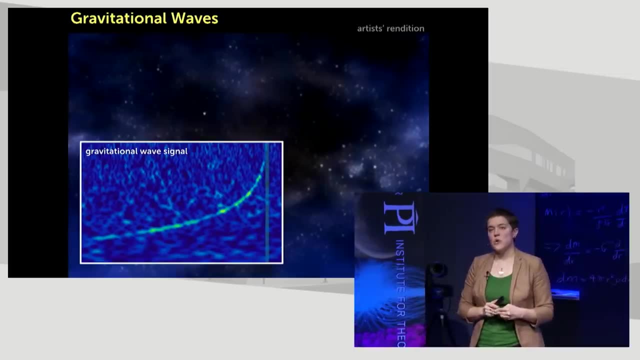 than the kind I talked about before, and they emit gravitational waves. We thought that this was going to happen for quite a long time, and on August 17th a gravitational wave signal from two colliding neutron stars was detected. So now we had something else. 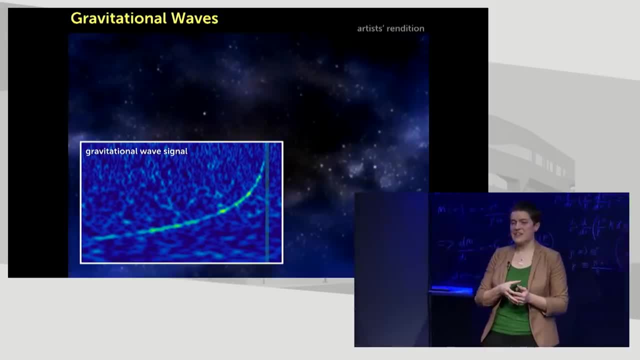 exciting to do When two black holes collide. we don't think there should be any light emitted by that process, but these neutron stars are emitting gamma rays. They're emitting light throughout the magnetic spectrum. So we had to move very, very quickly to try and find. 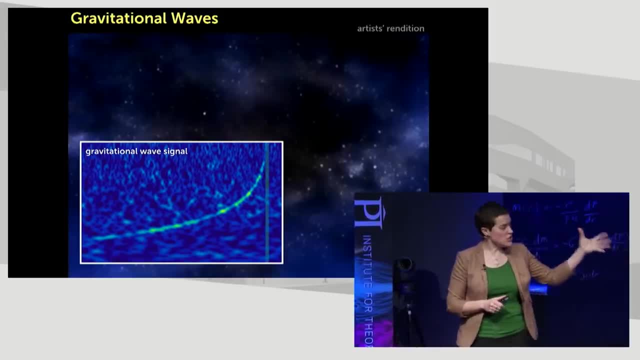 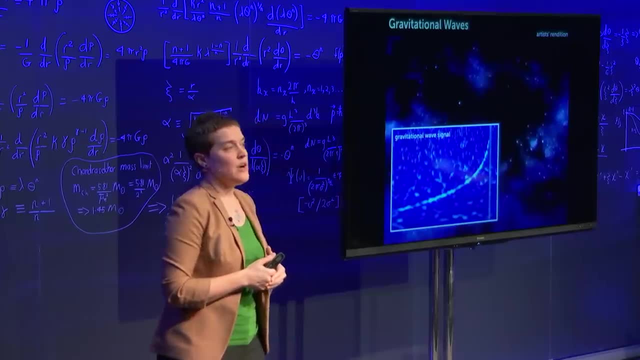 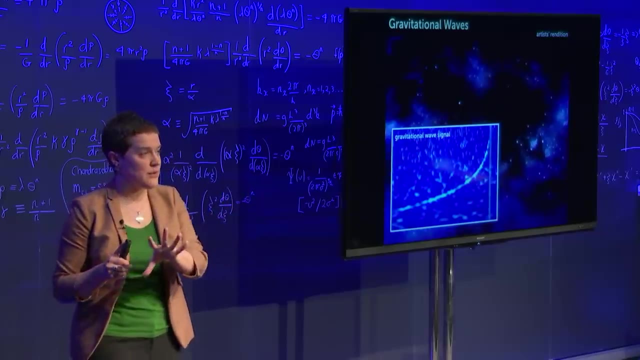 the electromagnetic light counterpart to the gravitational wave. So there was a team in Santa Cruz that was working on this. They had very quick observations with one of their telescopes of nearby galaxies where they thought this could have originated from, and they were frantically looking through them. 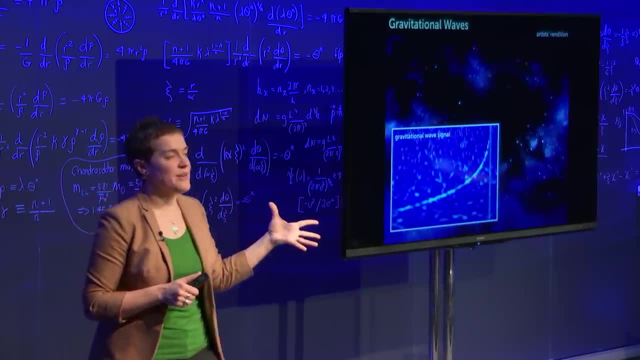 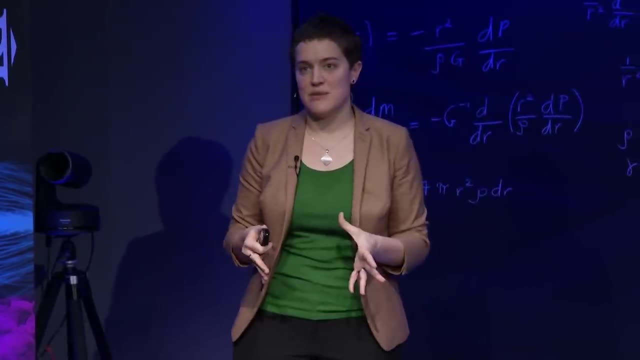 to try and see if one of them showed a sign of the flash of light coming from this event. It's very hard to tell exactly where gravitational waves are coming from, So they had a big list of images to look through And one of the researchers on the team. 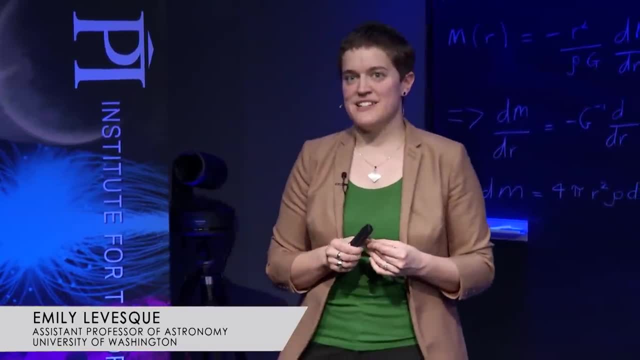 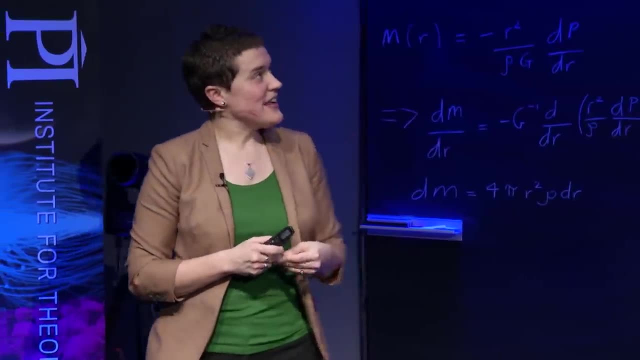 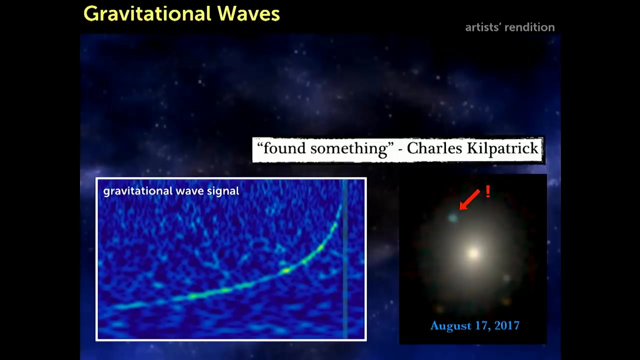 had about the most understated response to this discovery ever. He sent a message around to the team that just said: found something. In one of the images they saw the unmistakable sign of one of these events. So this was time domain astronomy. This was astronomy that had to happen. 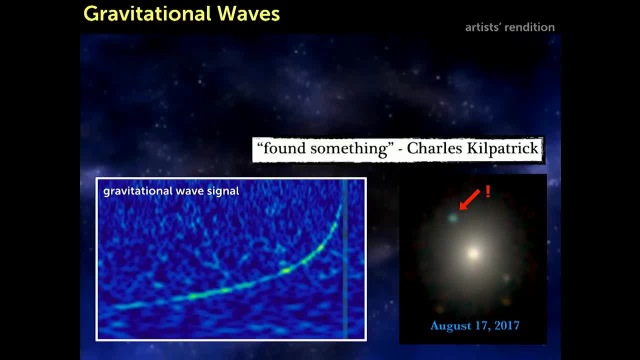 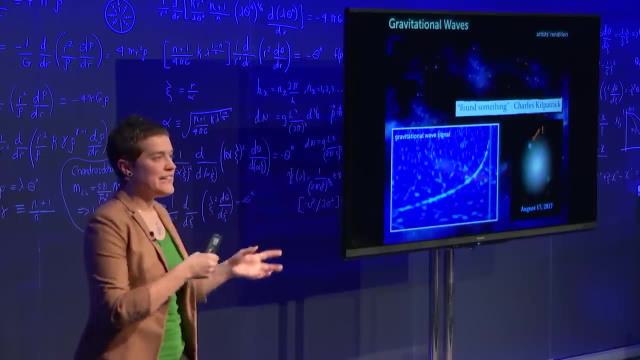 quickly and also had to happen carefully, But it resulted in us discovering for the first time gravitational waves and light coming from an object in space, which was really just incredible. I've been talking a lot about weird discoveries and surprising discoveries and fast or fleeting or 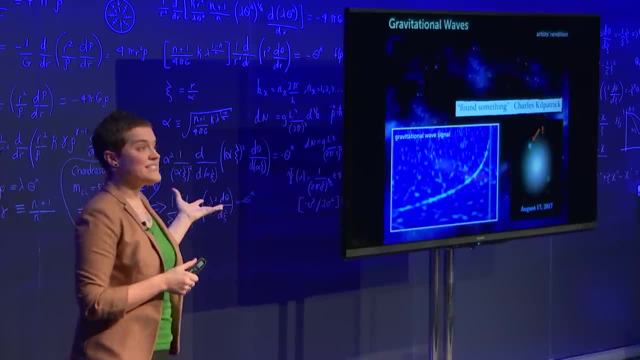 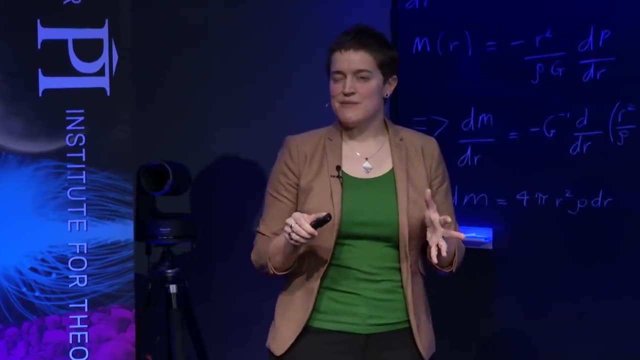 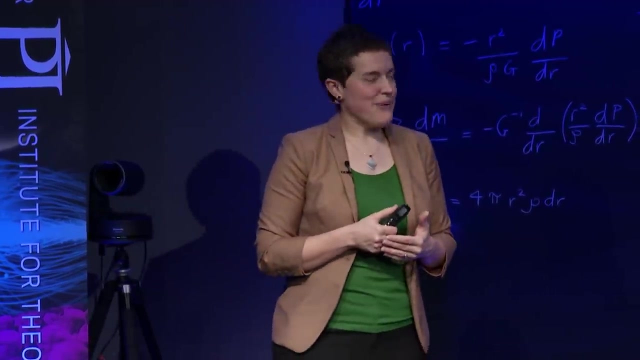 unusual discoveries. Sometimes this means something amazing, like detecting gravitational waves and light from two colliding neutron stars. Sometimes it's maybe a little less dramatic. Sometimes it can even be a little bit disappointing once you look at the real reason why. One example that I like: 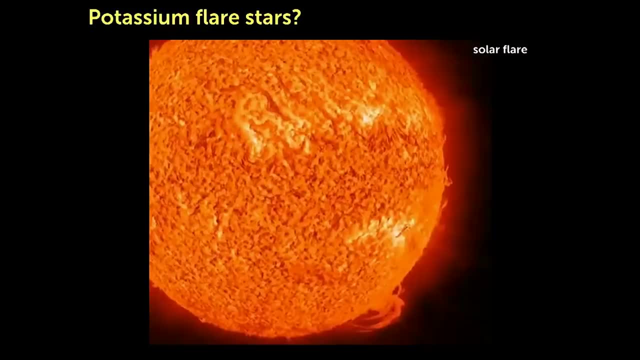 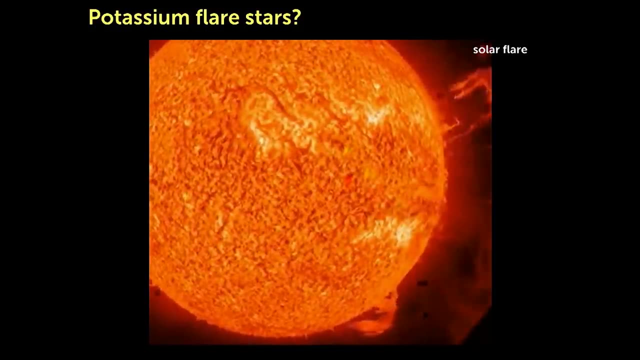 pointing to are potassium flare stars. So we know that our sun will produce what we call solar flares. It's this eruption of material from the surface of the star, and it shows up to us like a little tiny brightening. Other stars will also behave this way: Stellar flares. 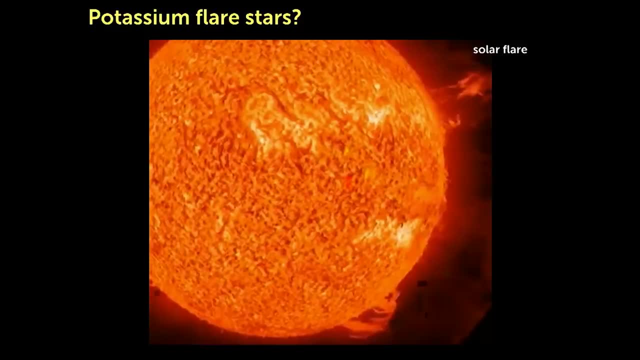 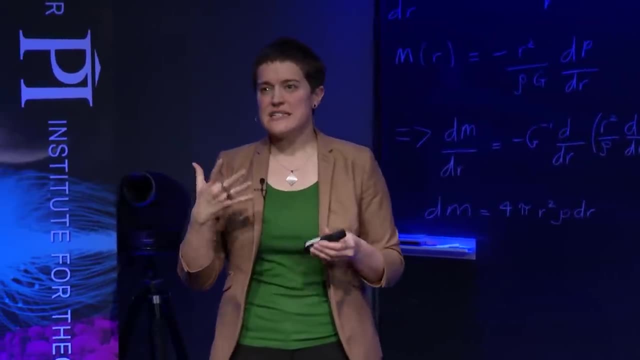 are fairly typical And at the distances of the stars that we're talking about, the flare has to be very bright. So for years studying stellar flares and understanding stellar flares was somewhat commonplace In the 60s at Haute-Provence Observatory. 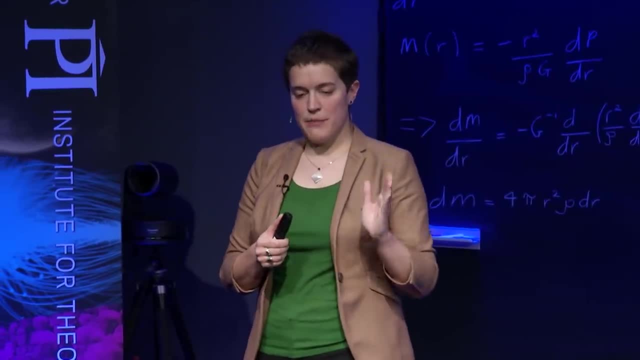 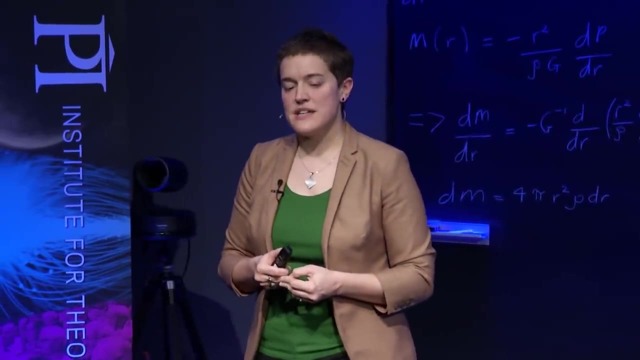 in France, some astronomers were observing and taking data on a bunch of stars and analyzing the data as it came in, And they were extremely surprised by one of the results that they found. They saw a star that in its spectrum appeared to show a stellar flare. 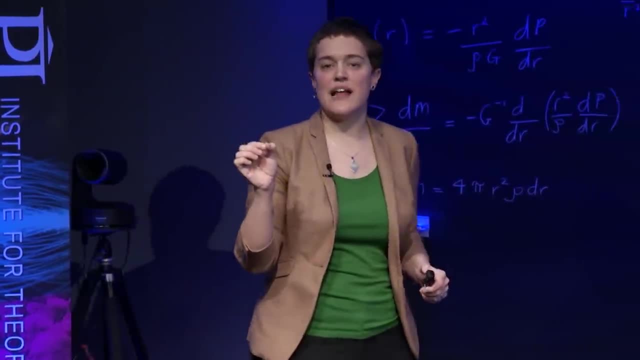 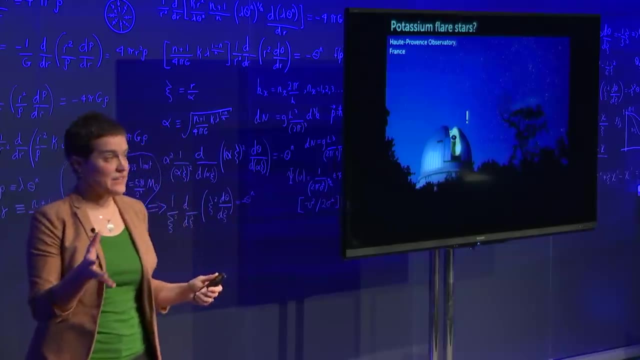 that was very strong in a specific element. It was very strong in the element potassium. Nobody had ever seen this before. This wasn't a prediction of normal stellar flares And they were really surprised. They were going: wow, we found a new type of physics. We found a new type. 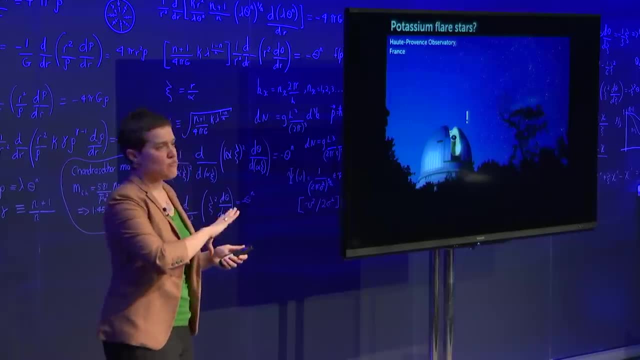 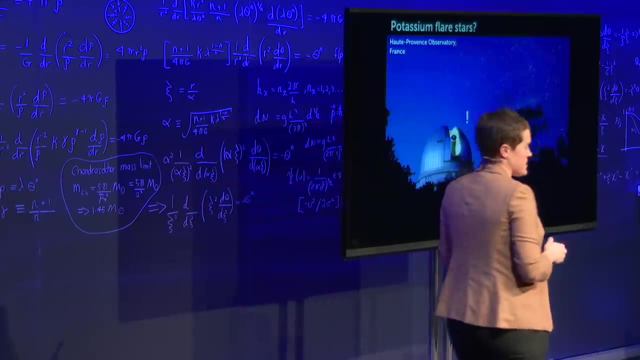 of flare. We're seeing potassium flares from these stars. They wrote a research paper. It was really fascinating And the community was really interested. They were going: okay, how do you explain potassium flares from a star? And it got better. 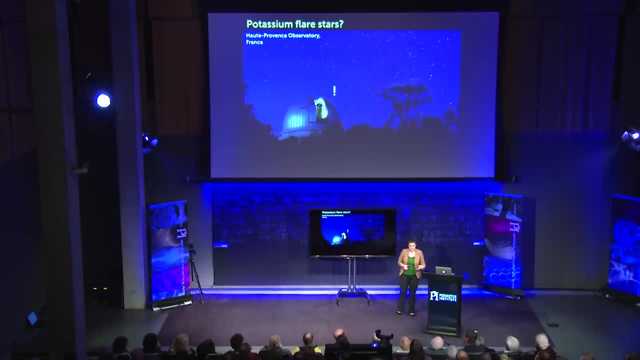 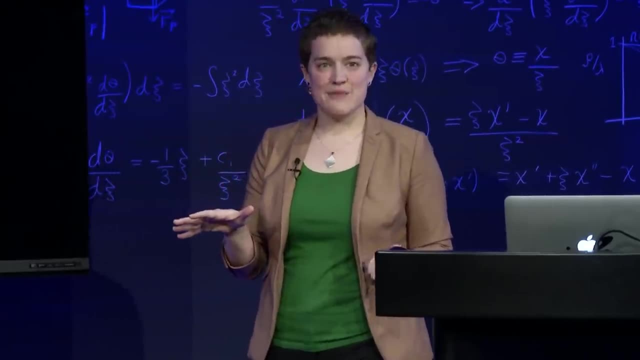 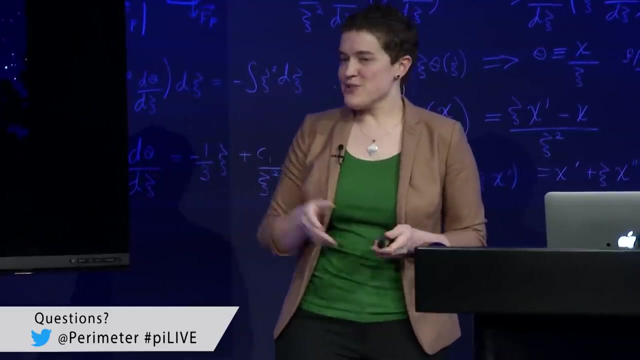 Two more potassium flare stars were discovered. In those discoveries, though, we started to see a little bit of a problem. Nobody else was finding potassium flare stars except for this team, And they were only finding them at this telescope. So another research group in 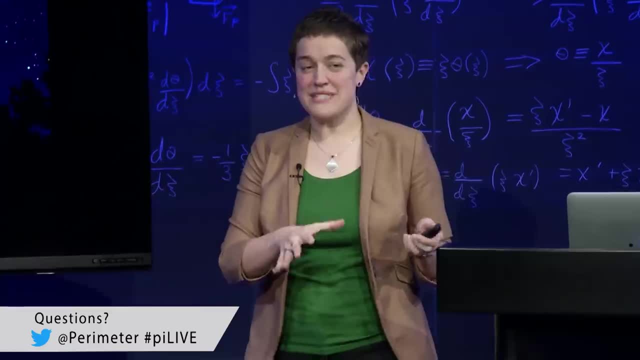 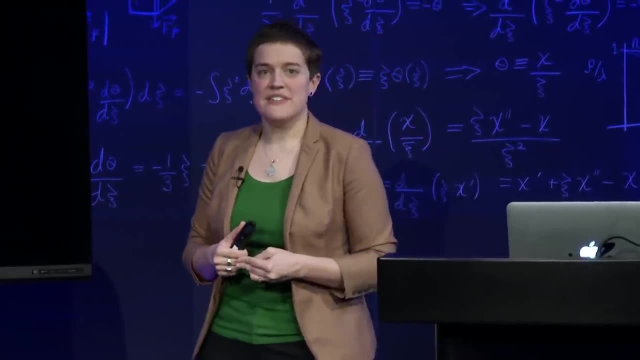 California decided to look into this, Decided to see if maybe there was some other explanation for what was going on. So to understand why it's good to look at how telescopes like this are built. This is a very typical telescope design. It's known as a casagraine. 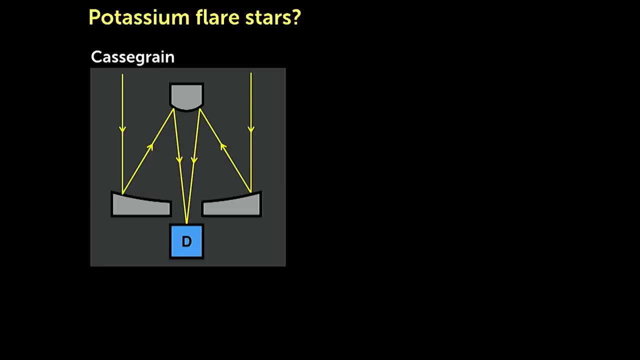 Light will come down onto the primary mirror depicted in the bottom. It will bounce up to a secondary and then bounce from the secondary down to the detector that we're showing in blue. This can be a photographic plate. This can be a digital camera, like we have now. 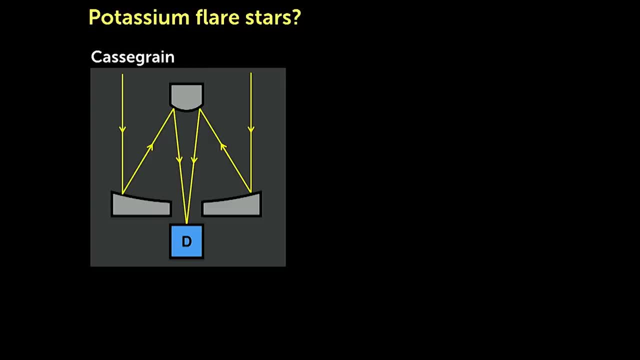 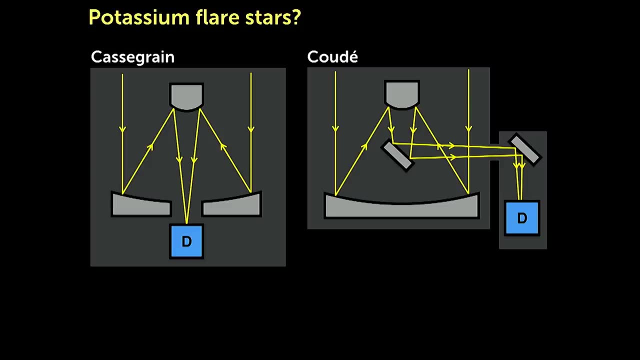 It's a fairly straightforward way of gathering light from a telescope. The telescope that was being used in France was taking advantage of something called a coude design. In this case, we're bouncing off a couple of other mirrors along the way, and we're actually 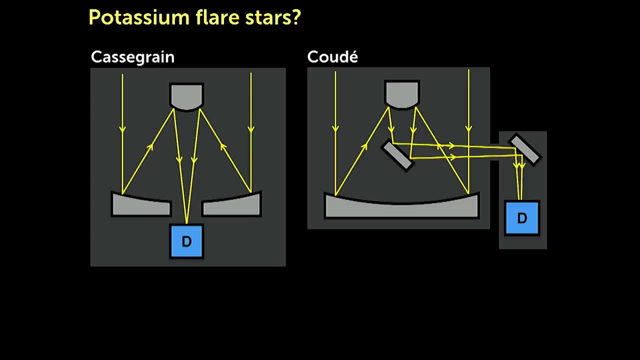 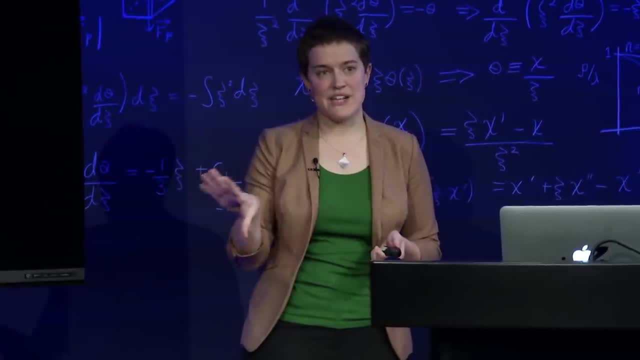 sending light to a detector in a completely separate room. There's good reasons for this: That travel that the light has to go through actually improves the quality of the image, And sometimes it's nice to have the detector in a completely separate room- In this case, that separate. 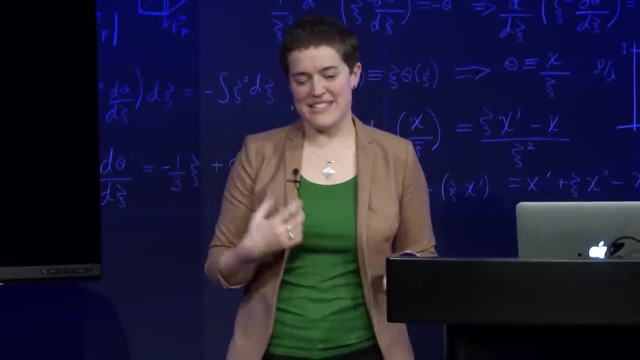 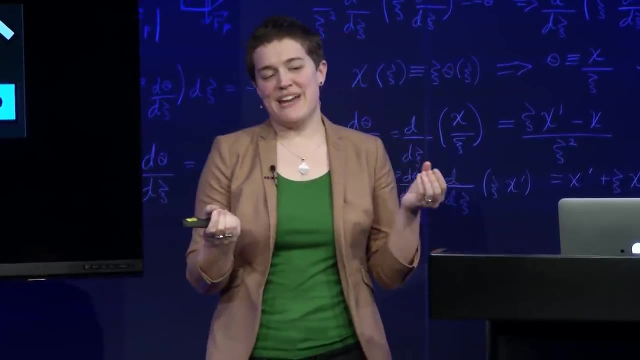 room was a nice little place where you could maybe go and take a break partway through the night. It's the 60s, It's France. Maybe you're taking a break and you decide to have a smoke break and strike a match. 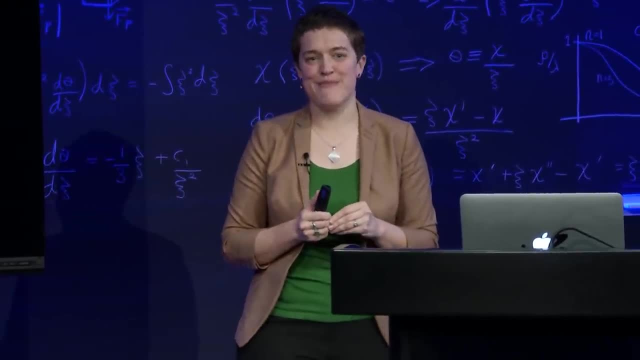 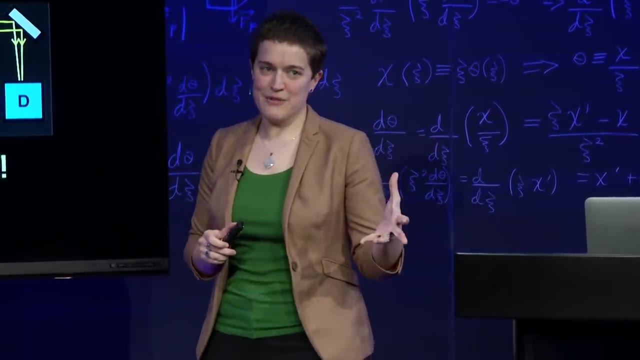 Potassium is the strongest element in the spectrum of match. So people at Berkeley figured out that this might be what was going on. They had an amazing research paper where they tried to debunk this, and it essentially involved running around the dome of one of the 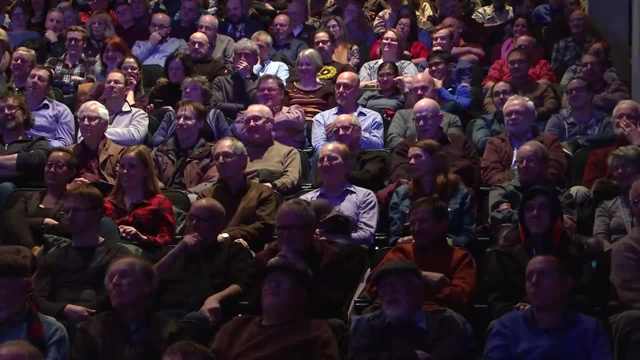 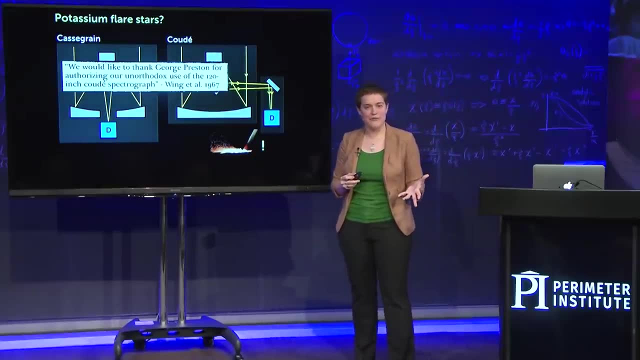 telescopes, playing with matches and striking matches to see if they could reproduce a potassium flare. They acknowledged in their paper George Preston, who was the director at the time, for authorizing their unorthodox use of the 120-inch Cadea spectrograph. 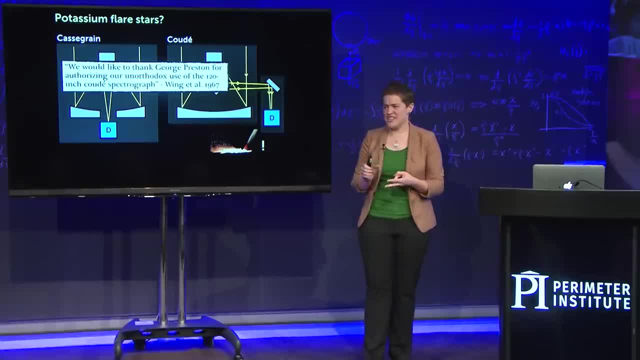 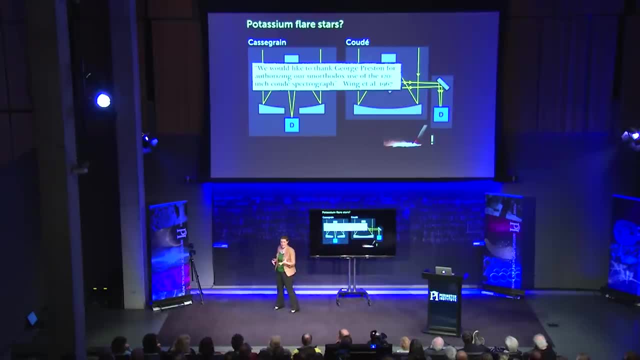 The paper is amazingly thorough, by the way. They check book matches, They check kitchen matches, safety matches. They contacted the people in France who were perhaps a little surprised that this was the explanation, but scientists at their core And they said, hey, let's try our matches. 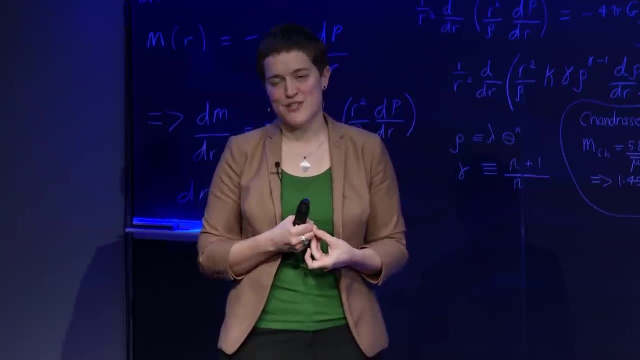 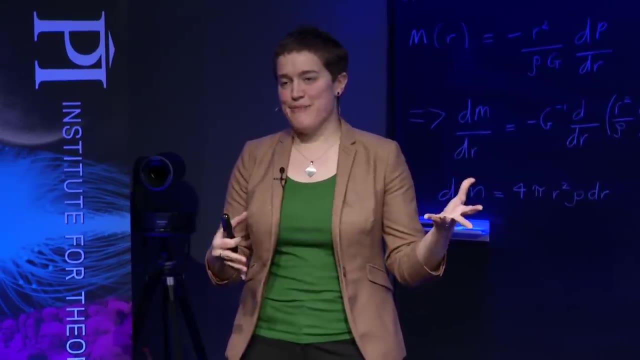 There's a line in the paper explaining that there is no spectroscopic difference between French and American matches, And we now have a research paper that includes data on, you know, the spectrum of a match. I assume that that room in the telescope in France is now non-smoking. 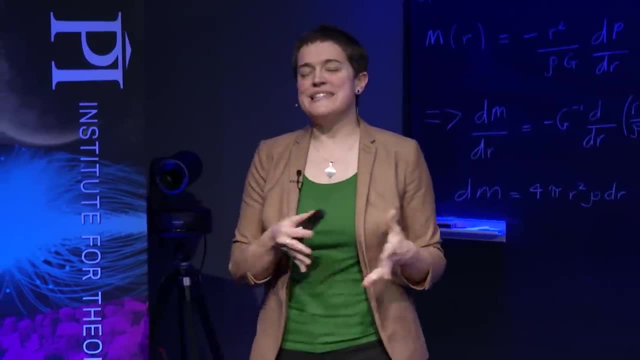 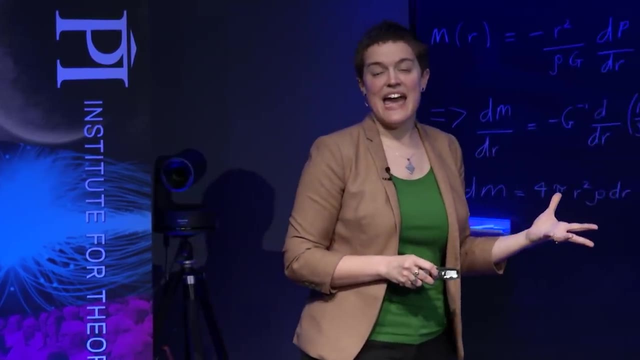 And you would think that the potassium flare stars had then been debunked. What's great is that a few years later, another observer was observing a star and did see excess potassium in the spectrum, And they took care to note in their paper that the 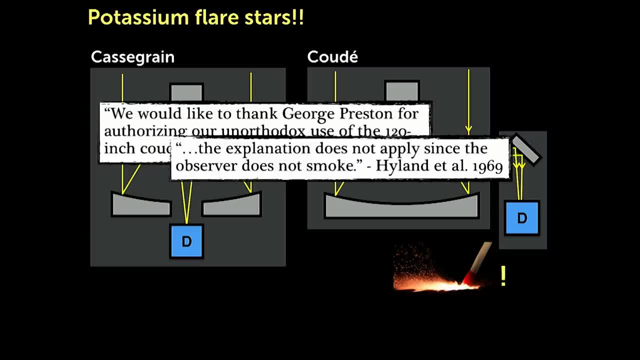 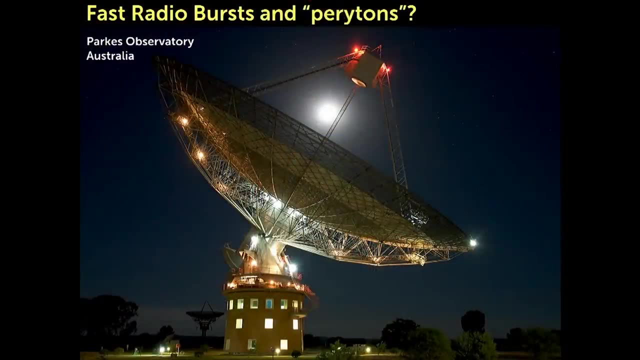 explanation did not apply since the observer does not smoke. So potassium flare stars really are out there, but perhaps not in the manner that they were originally discovered. Another good example of this happened at Parkes Observatory, which is a radio telescope in Australia, And this has to do. 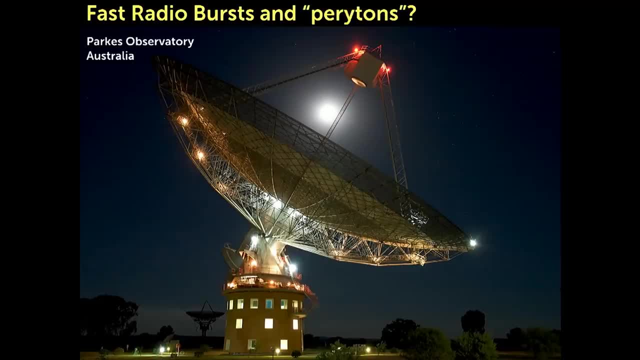 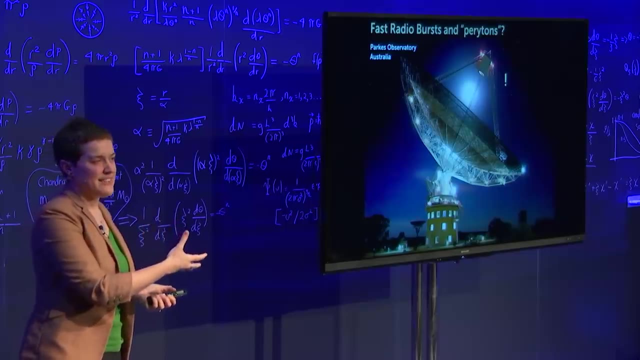 with phenomena called fast radio bursts and something called a periton. So during observations with this radio telescope, they detected a brief burst of radio emission. This was surprising. This was very interesting. We've seen gamma ray bursts, but a radio burst like this and 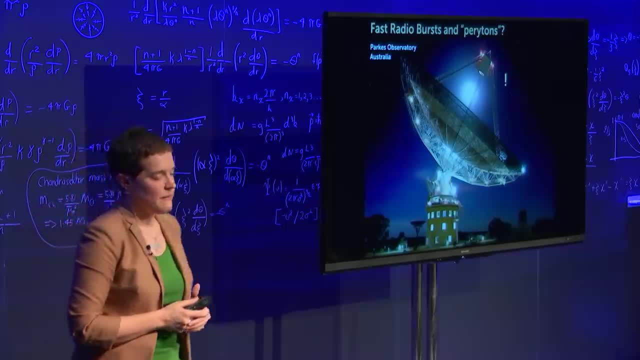 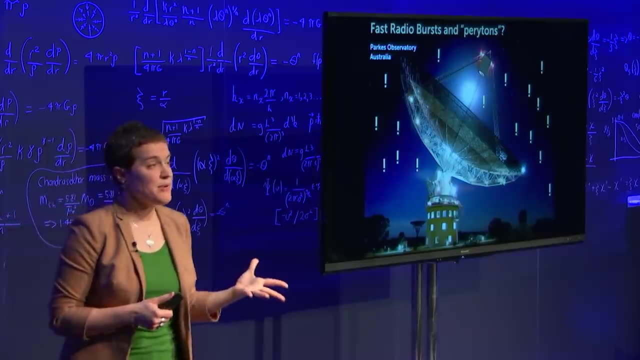 especially one on that rapid time scale, was really puzzling. Now, when they put this out, some responses started coming in going: oh, a flash of radios- Yeah, we see those all the time. There's lots of these. This is probably something really cool. We should figure. 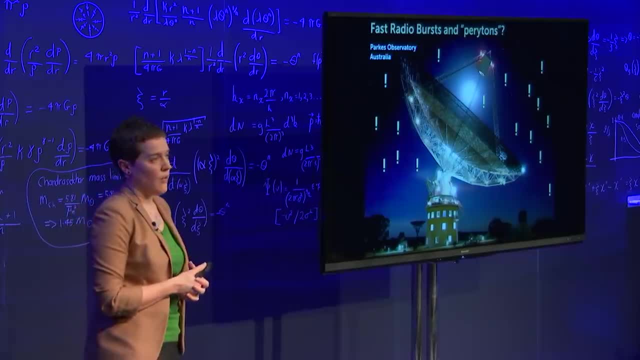 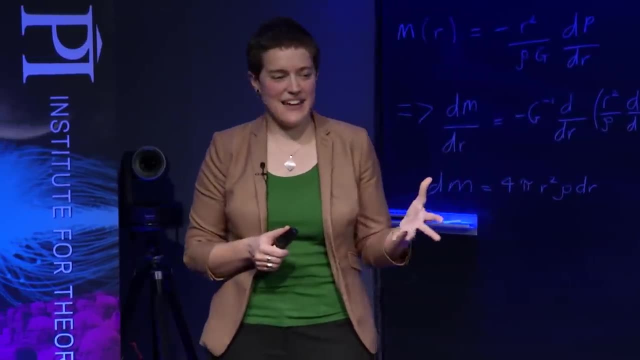 it out And they started digging into the data as a whole to see what these were. Now those other detections were nicknamed peritons And it was a sort of tongue-in-cheek name saying maybe these aren't entirely celestial. Maybe we have some other explanation for this, but we don't yet. 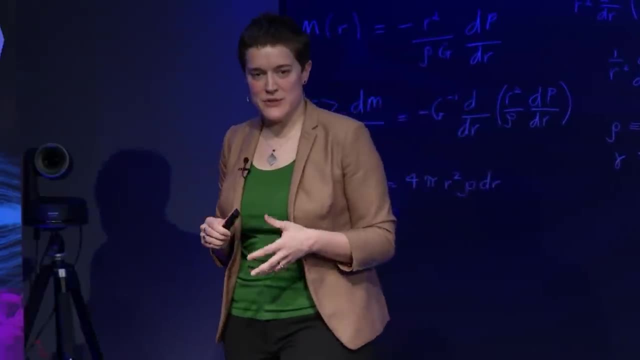 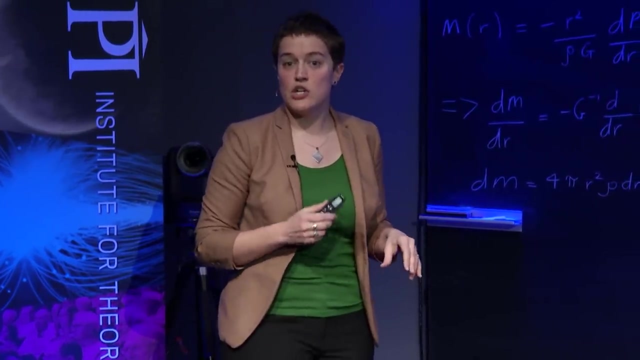 know what it is Now. the key came when you sort of step back and look at where the Parkes radio telescope is in the larger observatory. There's a couple of other buildings, There's a couple dorms or administrative buildings, And in the paper, 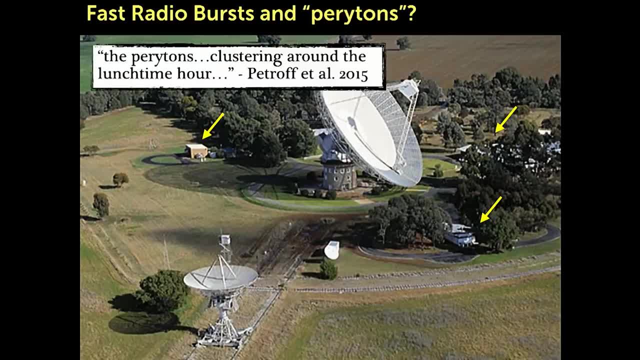 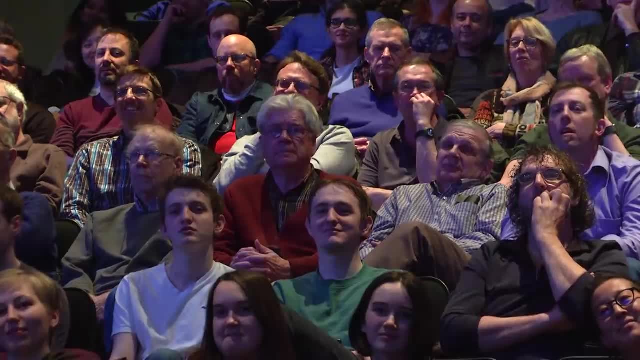 that finally explained this. they noted that peritons were clustering around the lunchtime hour of the day, So everybody in here, I assume, has microwaved popcorn or dinner at some point, And you know how that goes: You're hungry, you're waiting and you're looking at the microwave. 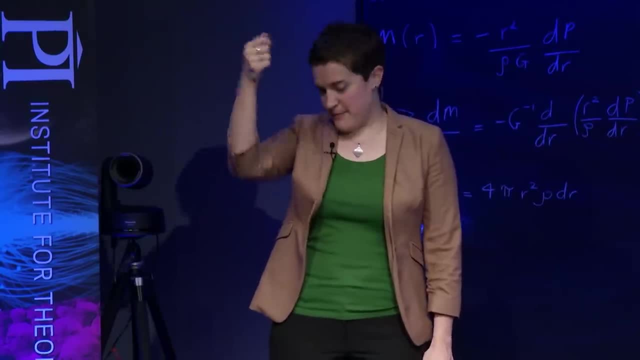 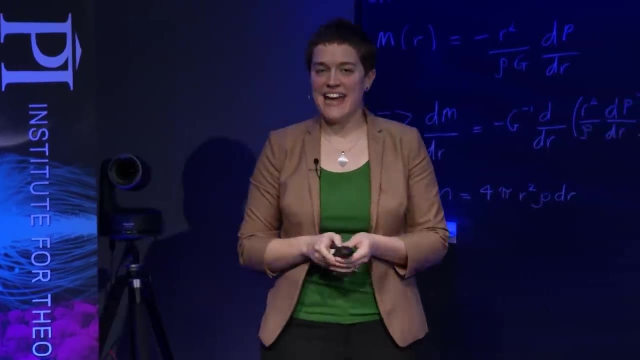 and it's going five, four, three, fine, And you just open the microwave door to stop it just a second or two before it's done. In old microwaves, doing that can sometimes cause a brief flash of radio waves that were being detected as peritons. 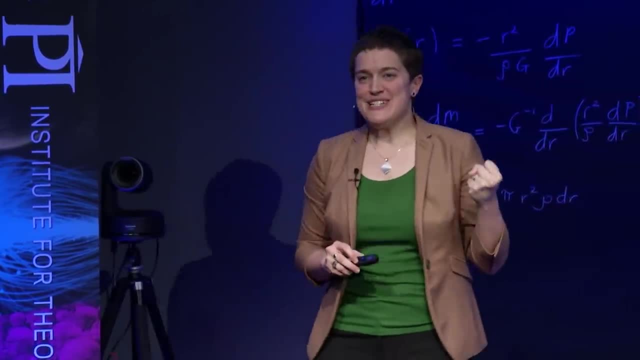 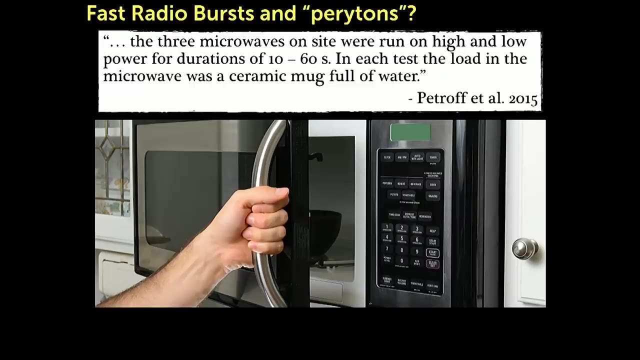 So again, there is a delightful research paper showing how this happened. They tested all three microwaves on site. There's a paragraph where they probably learned more about microwave design than I think they ever wanted to in their lives. Microwaving a ceramic mug full of water. 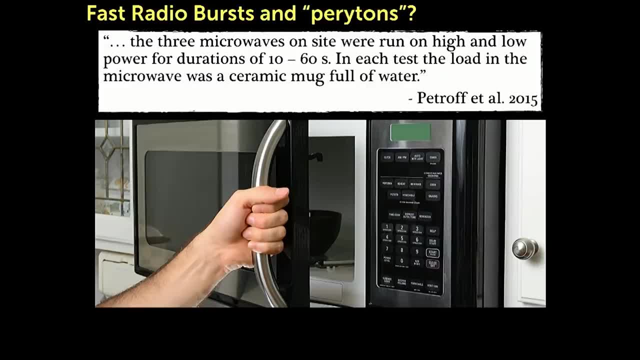 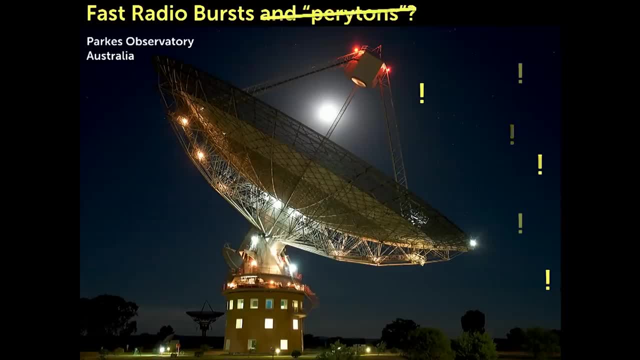 microwaving the same thing every time, But ultimately determining that, yes, that was what these peritons were. All of those detections were probably just flashes from microwaves, right, Most of them were, One of them wasn't. 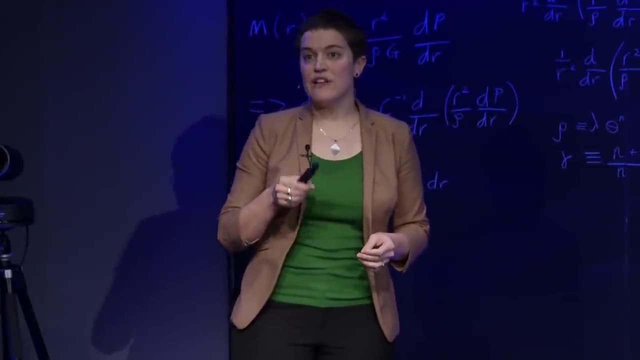 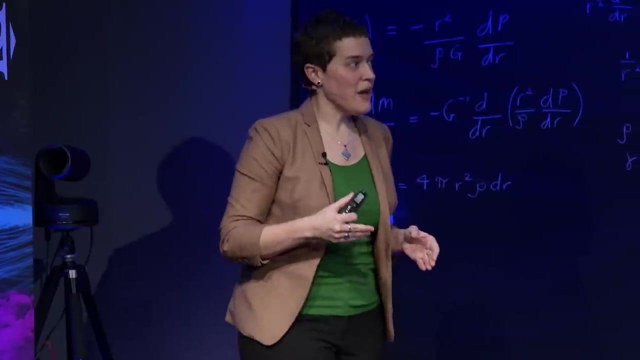 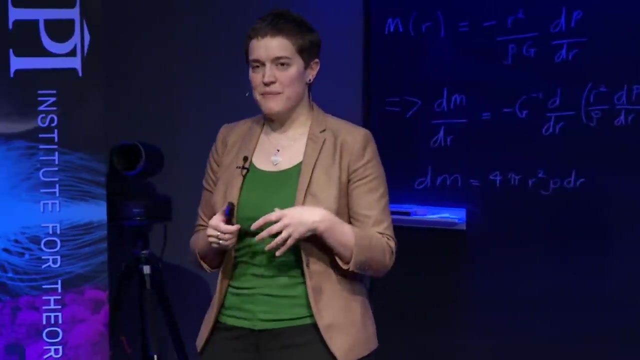 Fast radio bursts again are real phenomena. They are fascinating phenomena that we're still trying to understand. We are now detecting more of them. We know how to separate them from something like being impatient with lunch, And we're trying to figure out whether these are coming from. 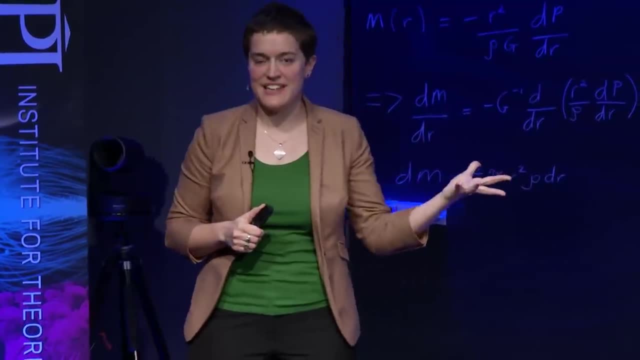 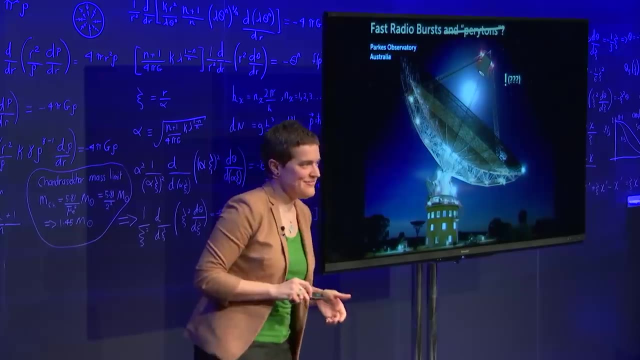 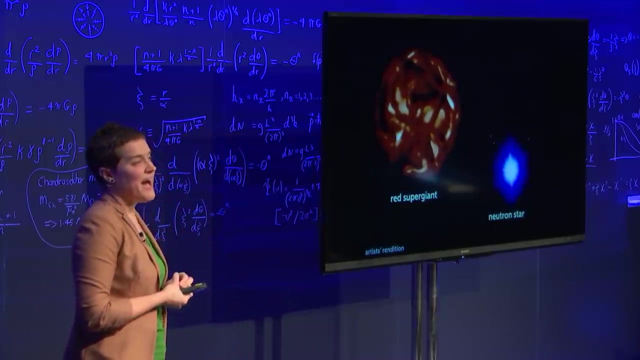 stars from objects that we maybe can't fully explain yet. They're a great example of a weird object in space, but one that was discovered in a slightly unorthodox manner. The last type of weird star that I want to talk about actually combines: 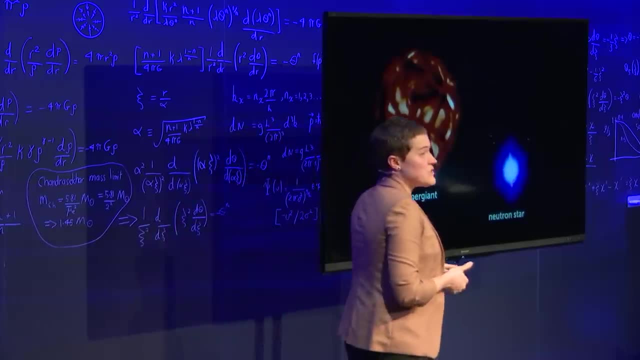 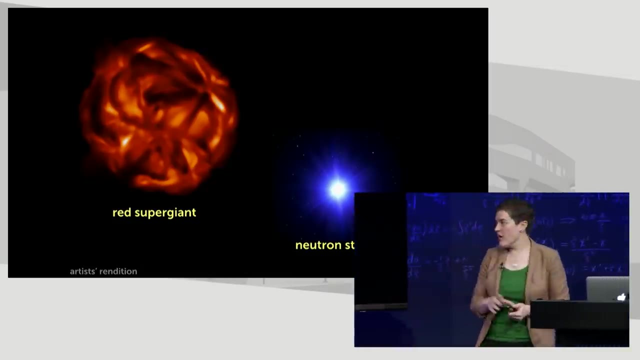 two types of stars that we've talked about before. I've explained red supergiants- what they are, how enormous they are, how cold they are and how they work, And I've talked about neutron stars, these quantum physics supported stars. 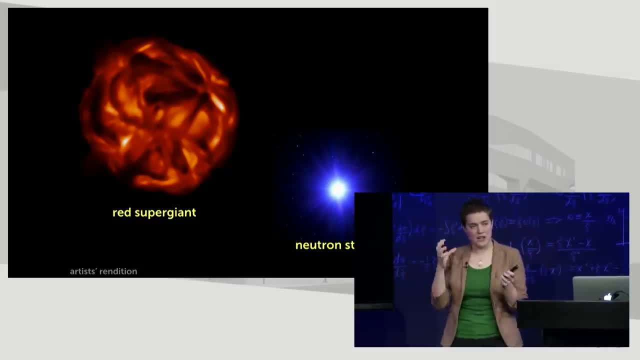 tiny and sort of dead remnants of a collapsed massive star. There's really only one way that you could possibly make these weirder, and it's to stick them together. So if you imagine a red supergiant and a neutron star in a binary, 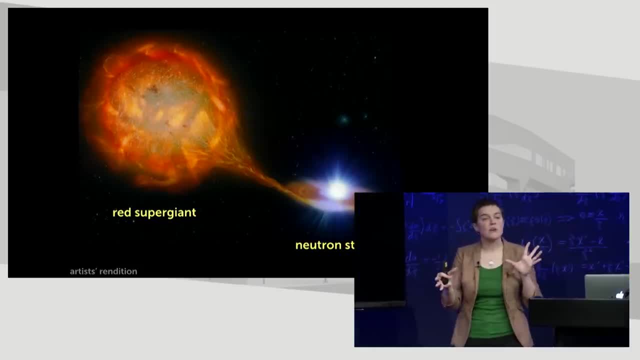 system. these are two stars that are orbiting one another and perhaps interacting with one another, exchanging mass, inspiraling closer and closer, kind of like those two neutron stars that we saw making a gamma ray burst. There's a really fascinating thing that can happen in a system like this. 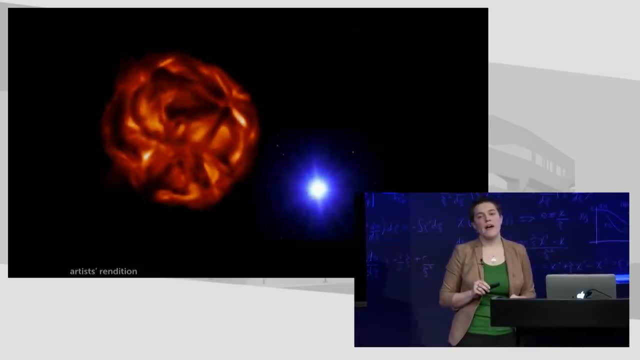 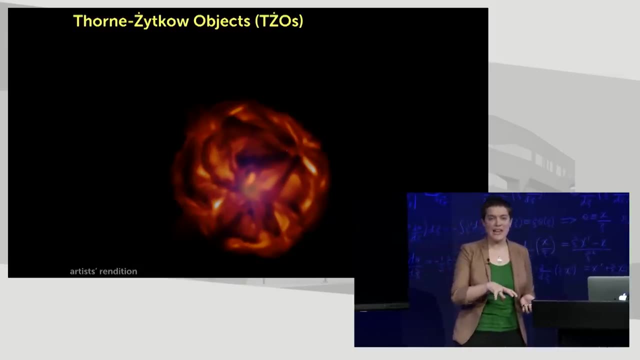 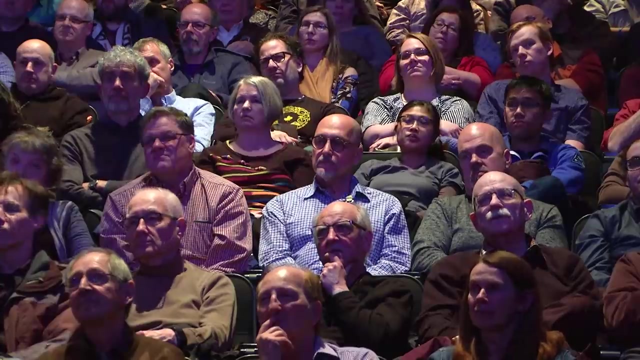 That neutron star can effectively be swallowed by the red supergiant. It can spiral in, settle into and eventually replace the core of the red supergiant and make something called a thorn Zhitkov object. I found out about these for the first time around. 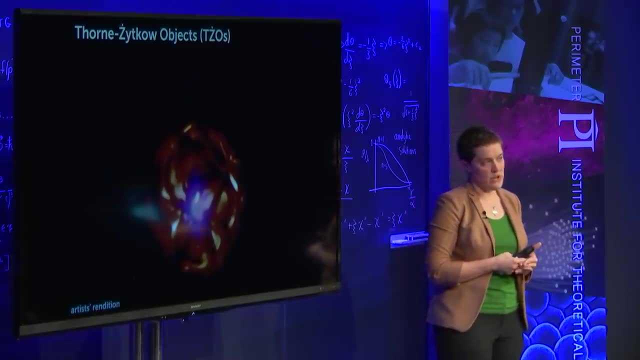 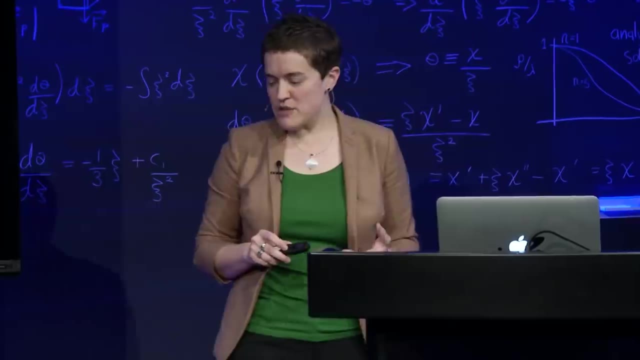 I think the year 2010.. I've been working on red supergiants for years, publishing papers on them and noticing some strange red supergiants, or red supergiants that we couldn't perfectly explain. And in response to one of those emails, 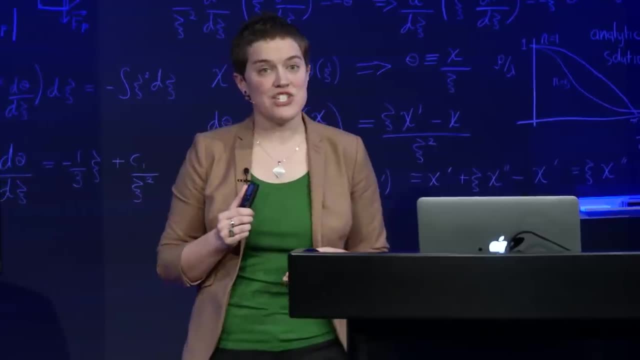 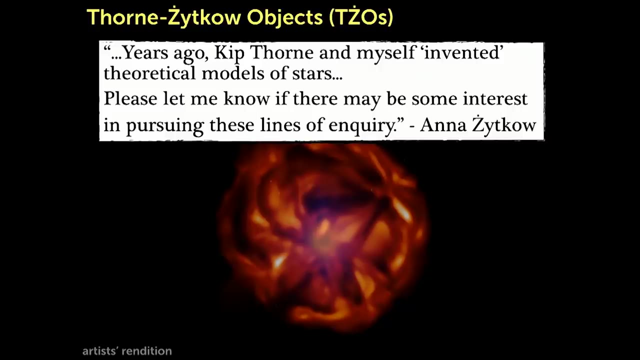 or one of those papers. I got an email from Anna Zhitkov saying years ago, Kip Thorne and myself invented these theoretical models of stars, which is just fascinating all on its own, and asking if we were interested in trying to look for them. 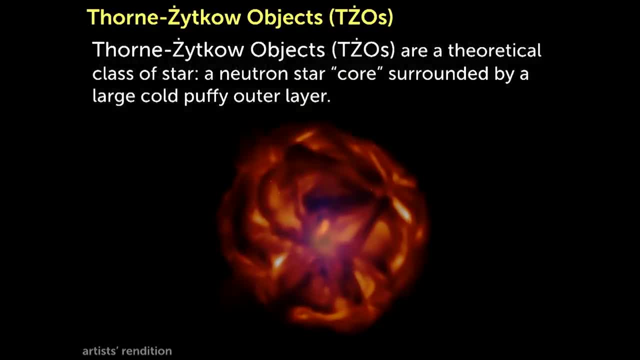 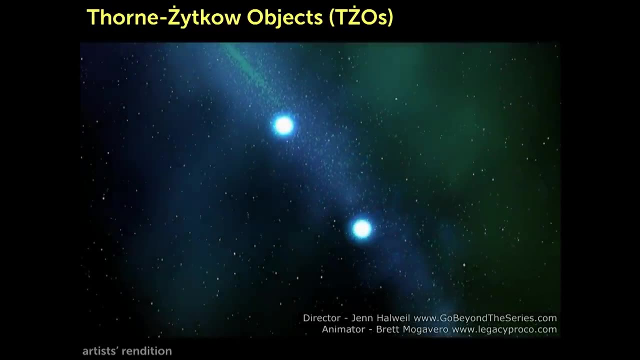 So Thorne-Zhitkov objects predict this neutron star core surrounded by a big, cold, puffy outer layer. They had predicted these back in the 1970s, but they'd never actually seen one. We had this rough idea of how they should work, You're imagining. 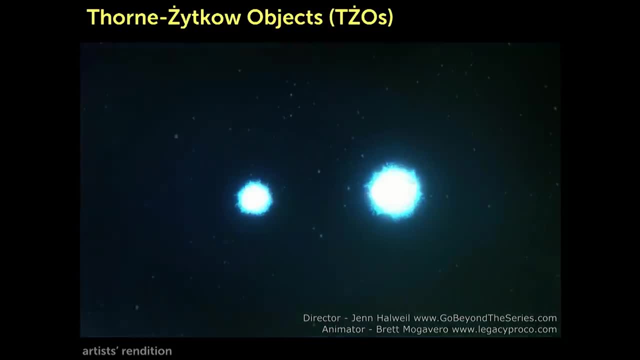 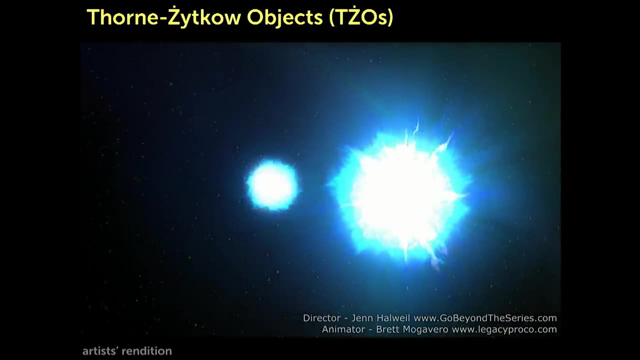 these two stars in a binary, two normal massive stars, two blue supergiants. The more massive of those stars, the one in the foreground, will collapse, undergo an incredible supernova, and what's left behind after the dust settles from that supernova is 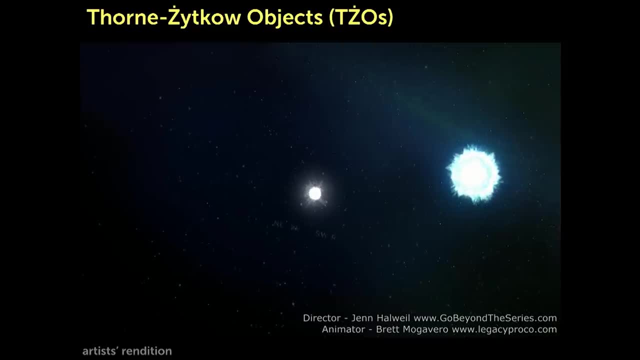 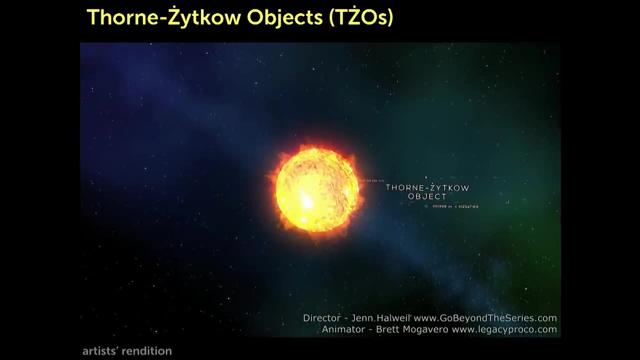 a neutron star. The companion of that star will start to expand, cool off, go from the blue supergiant to the red supergiant stage and swallow the neutron star along the way. It's a scenario that absolutely seems like it could happen, and 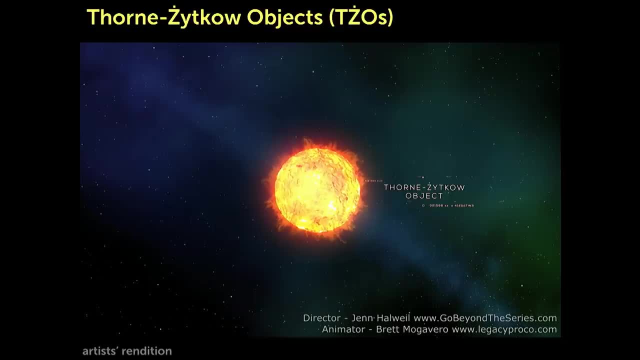 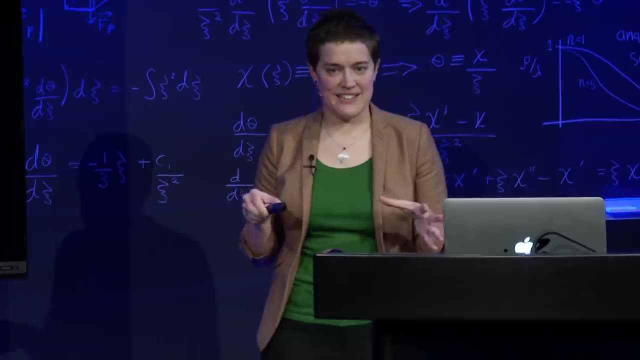 the physics saying that these stars should be stable seemed quite solid, but detecting them was a really big challenge. If I back out and look at this again for a second, remember a red supergiant is the size of Jupiter's orbit. A neutron star is the size of the city. 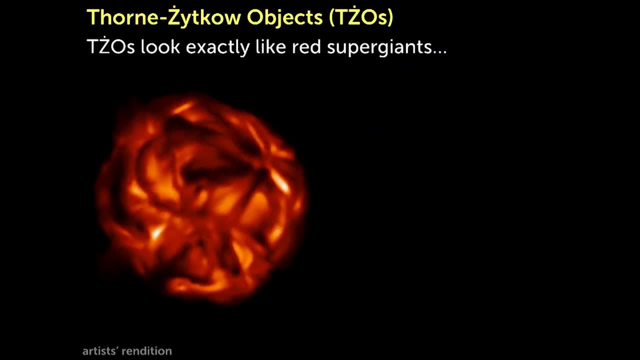 of Waterloo, So that neutron star cannot simply be seen inside the star. It's buried deep in the heart of the star And from the outside a Thorne-Jitgov object will look exactly like a red supergiant- almost We can take advantage. 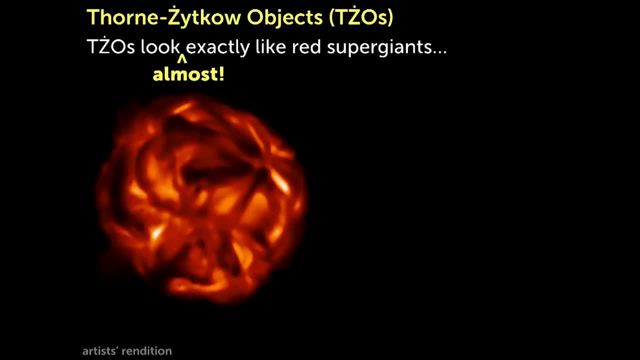 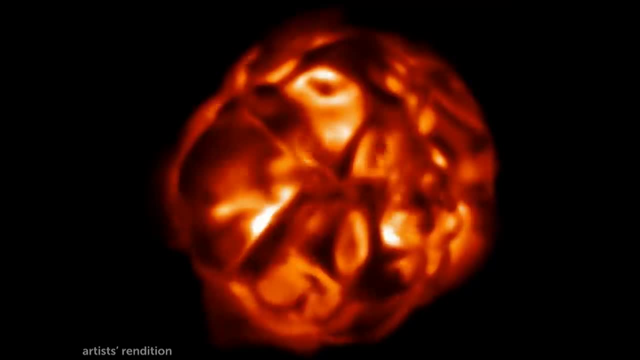 of the fact that there's a neutron star in the core of that star, to search for it in a very subtle way. So to explain this, I want to first remind you of that boiling convection that we see in these very cold, massive big stars. 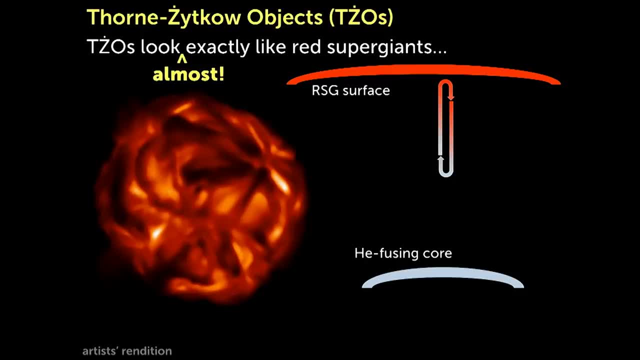 If I were to take a slice through a star like that, you can see the surface of the red supergiant, you can see the helium fusing core and you can see that convective cell in the middle. If I now change this from. 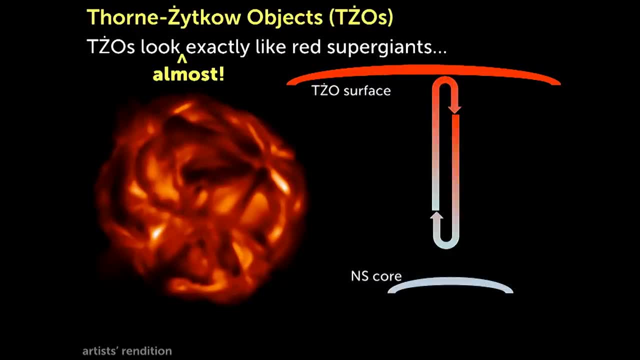 the cross-section of a red supergiant to the cross-section of a Thorne-Jitgov object. you can see a couple differences. One is that the core is now a neutron star. The other is that this star is quite cold. It's as cold as the cold. 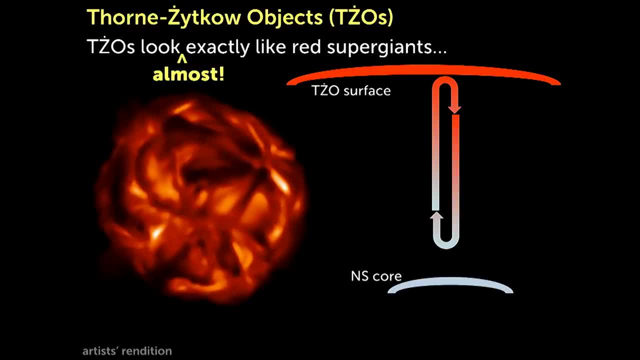 oldest red supergiants that we know about. That means that that convective region is huge. It actually takes up the entire outer portion of the star, from almost at the surface to almost down where the neutron star is. This means that we can see some really 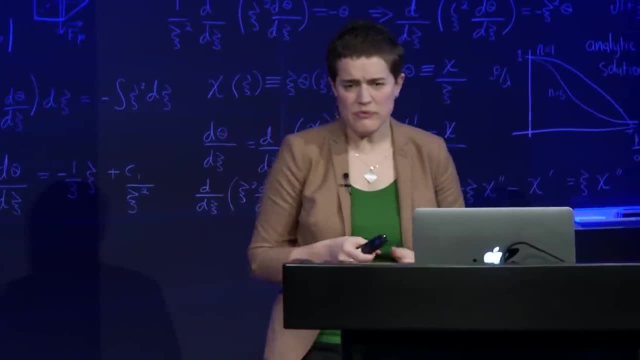 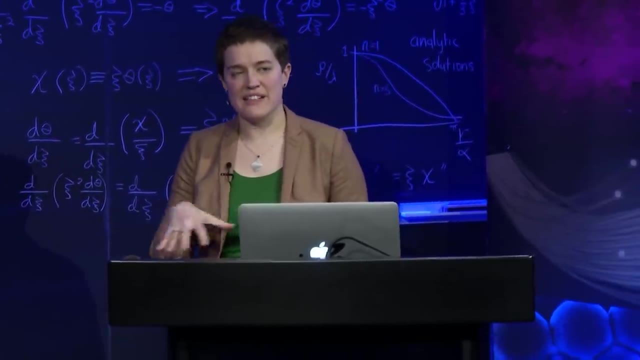 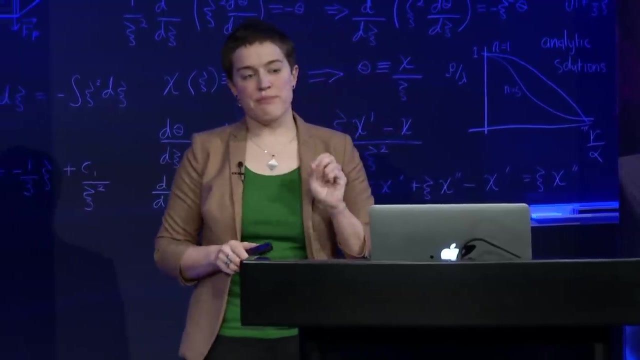 strange chemistry going on in the star. So if you imagine a packet of material traveling through that convective layer, it will get dragged down to that area right near the surface of the neutron star where the temperature and the pressure are really extreme. In that region protons. 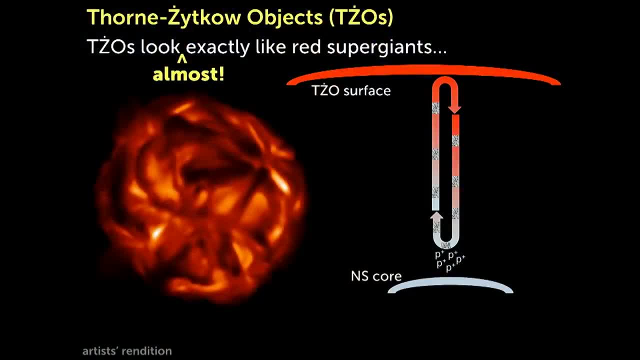 start getting rapidly shoved onto the nuclei of atoms in that packet of material And if you remember your periodic table, that means that these objects are starting to climb up the periodic table. Every atom is slowly increasing in atomic number. The thing is, material only stays there for about a hundredth of a. 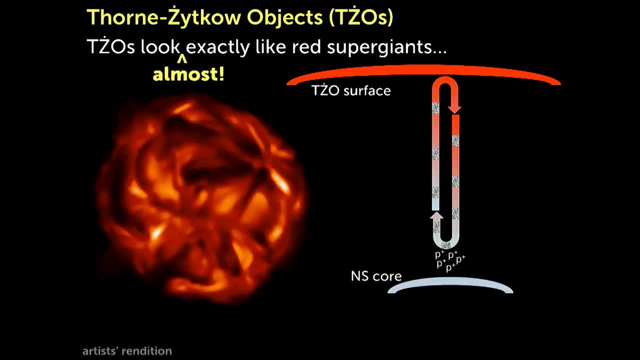 second. So it'll be bombarded with protons for a little while, drift back out into the cooler, quieter parts of the star's outer layers and start to undergo something called beta decay. It'll start moving back down the periodic table Before it can finish that. 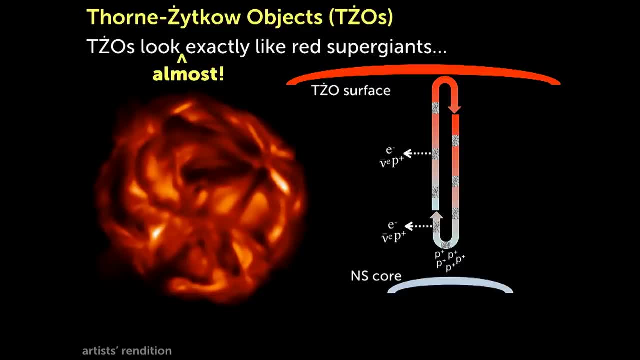 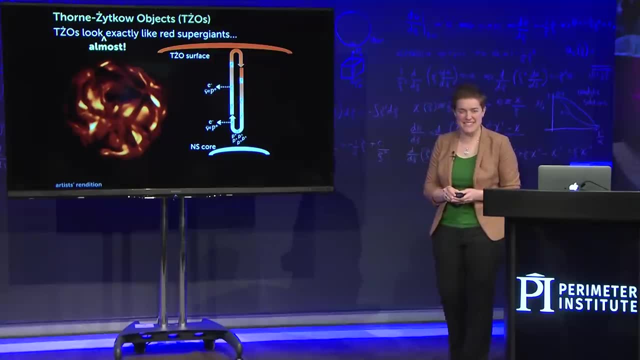 trip, it gets dragged back down to that lower region and bombarded by protons, and the whole thing happens over and over. This is a type of reaction that we can't expect in any other type of star, And it should produce a very 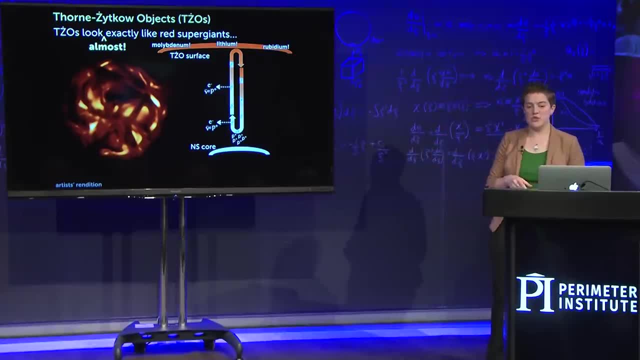 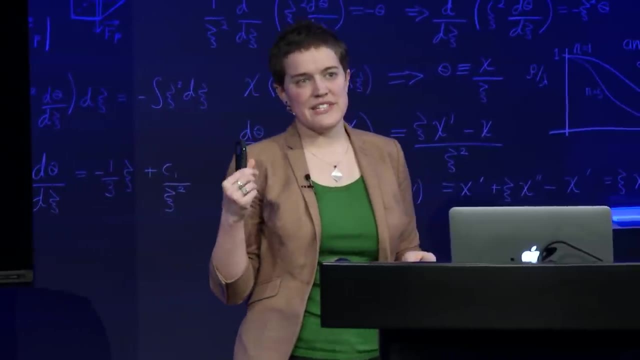 distinctive chemical signature. We should see huge excesses of things like molybdenum and rubidium and lithium, things that we would not normally expect to see a lot of- So we decided to use this odd predicted chemical signature to look. 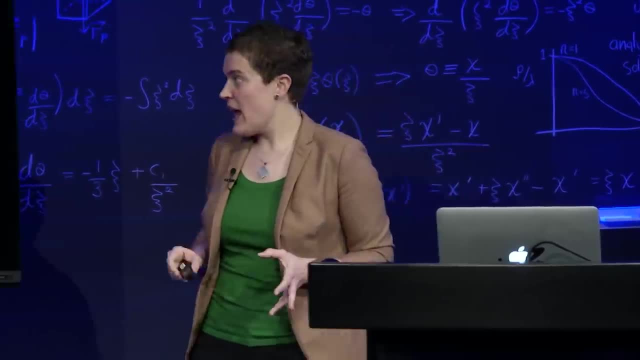 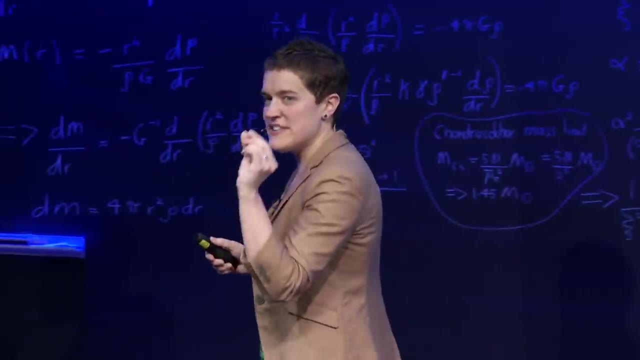 for Thorne-Zitkov objects. I showed you what the spectrum of a red supergiant looks like before. This is a very nice spectrum, but in order to look for these little individual elements, we had to basically take observations that let us zoom in. 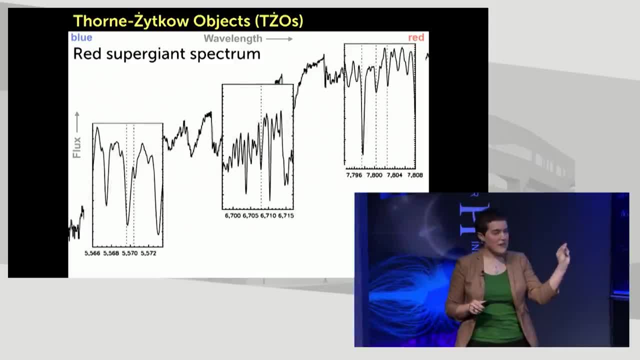 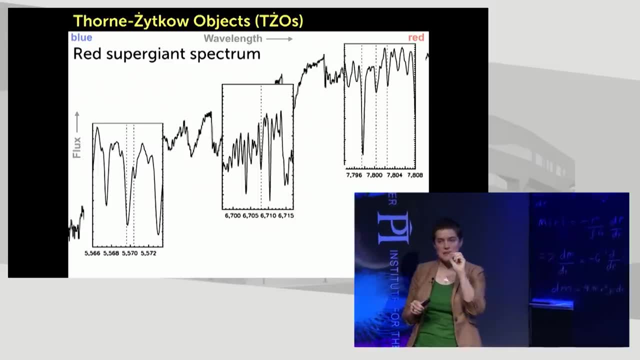 We could zoom in on very specific, small regions of the spectrum and look for the exact color that you would expect to see in a red supergiant. This is what you would expect to see absorbed by something like molybdenum. 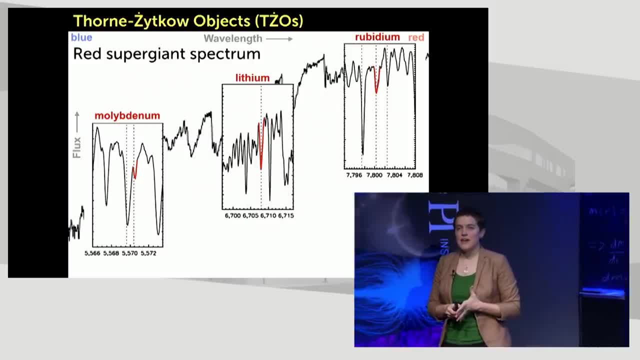 or lithium or rubidium. So you see again these little bites out of the spectrum coming from molybdenum, atoms absorbing light at a very particular wavelength, or lithium or rubidium. This is what a normal red supergiant would look like. 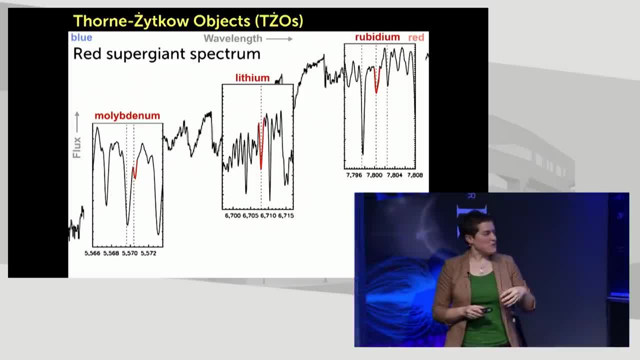 zooming in on these three regions and trying to look for these three elements, We observed about 70 stars, thinking you know what. Nobody even knows how much molybdenum is in a normal red supergiant. This is going to be step one of the project. 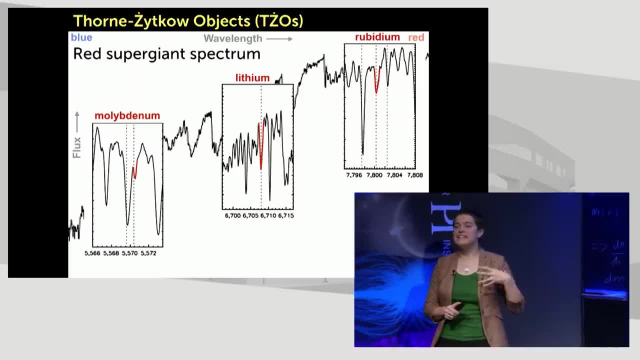 We'll look at what normal stars are like and then we'll start trying to move on. We'll survey more red supergiants and maybe one day we might find a Thorne-Jitkov object. So out of 70 stars, 69 of them looked like this. 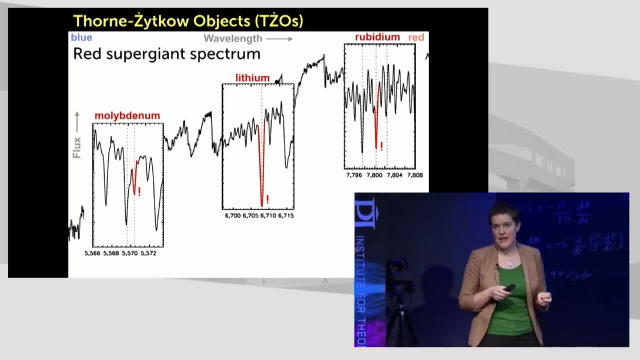 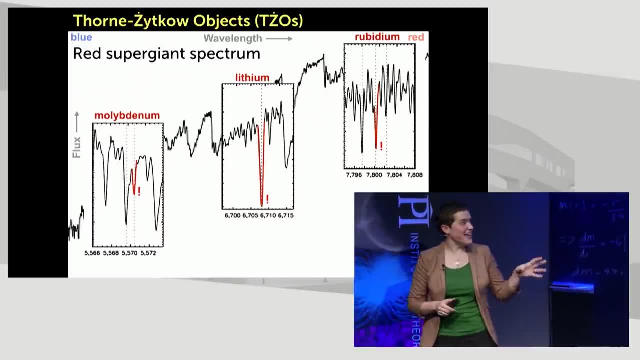 One of them looked like this. Now, if you'll notice, all those little dips just got a lot bigger. That means there's much more molybdenum or much more lithium or much more rubidium absorbing light. You can detect three elements. 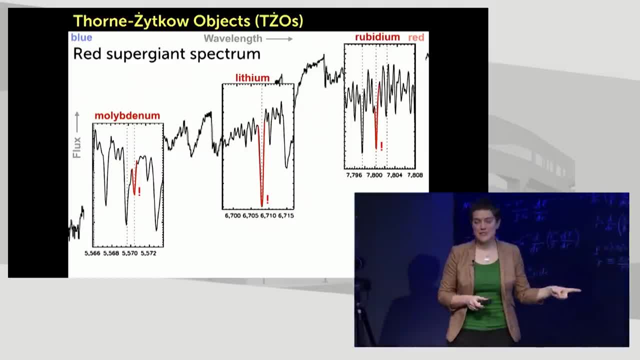 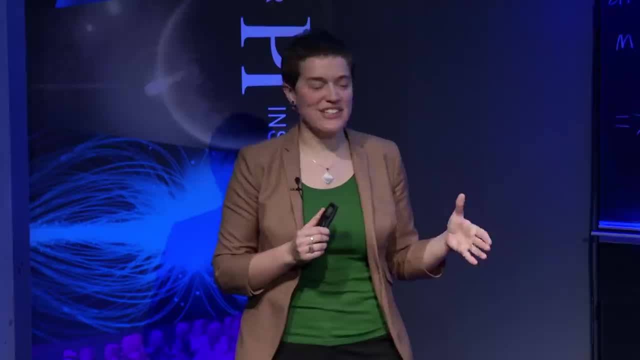 the elements that you would predict from a Thorne-Jitkov object in the spectrum. We were amazed by this. We looked at every aspect of the spectrum we could possibly think of and we eventually had one of our collaborators say this, looking at the star. 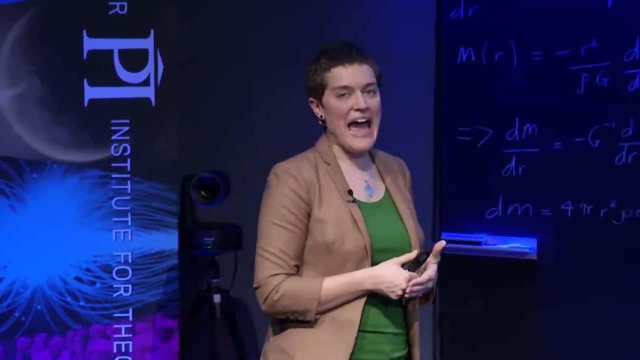 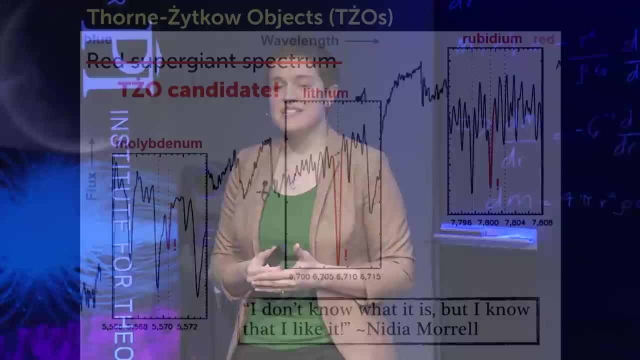 I don't know what it is, but I know that I like it. When we compared what we had to the predictions of Thorne-Jitkov objects, it fit beautifully. So we now have what we think is the first candidate for detecting a Thorne-Jitkov object. 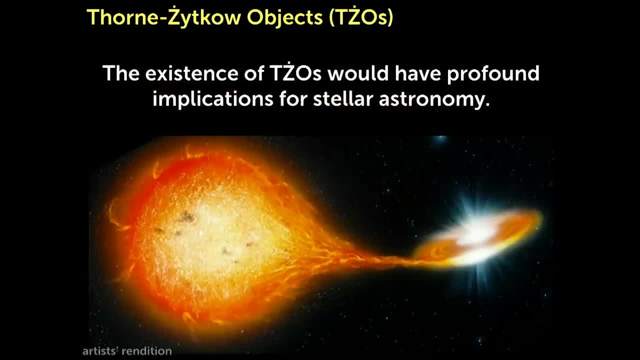 I'm very careful to use the word candidate here. The existence of Thorne-Jitkov objects would have really profound implications for stellar astronomy. The fact that you can have a stable star with a neutron star for a core is really surprising. It gives us a new 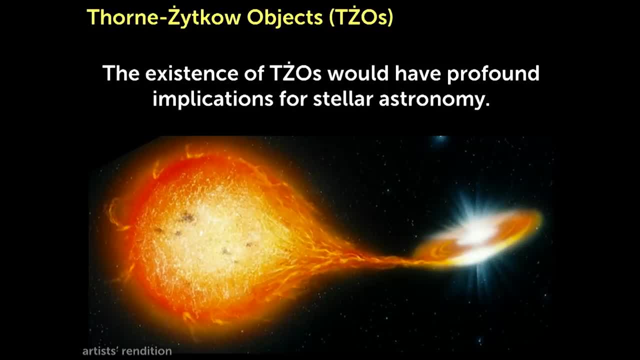 understanding of how stable stellar interiors could work. It came from a system like this: these two stars in a binary that merged, So it gives us a slightly better understanding of how binary stars can behave, And it's a great tool for me for making things like molybdenum and lithium. 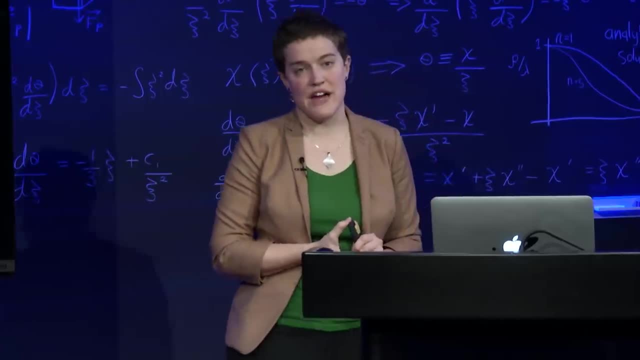 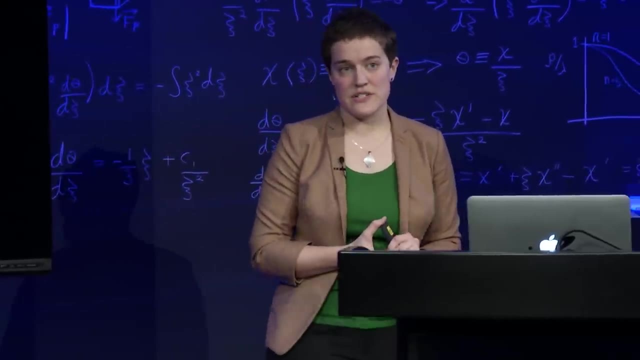 You'll hear this phrase- that we are all made of star stuff and stars really are factories for producing most of the atoms that we see and most of the elements that we see in the universe. So a new way of making some elements is always fascinating. 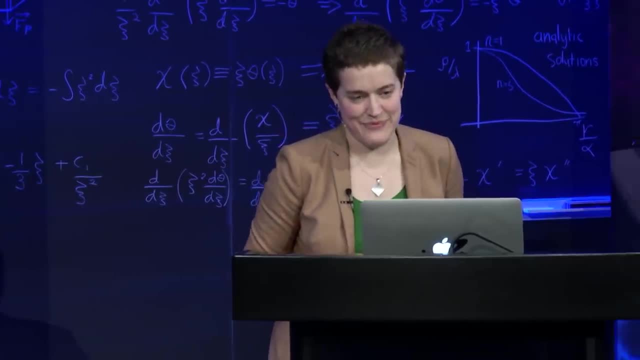 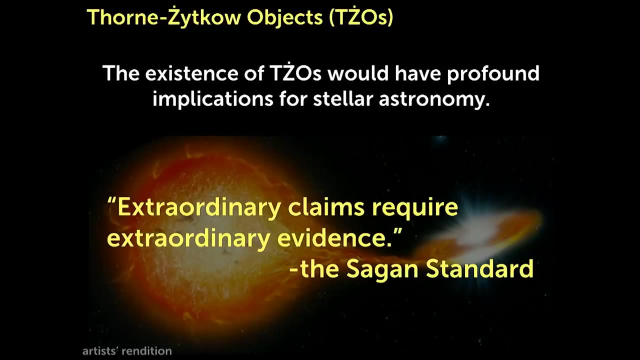 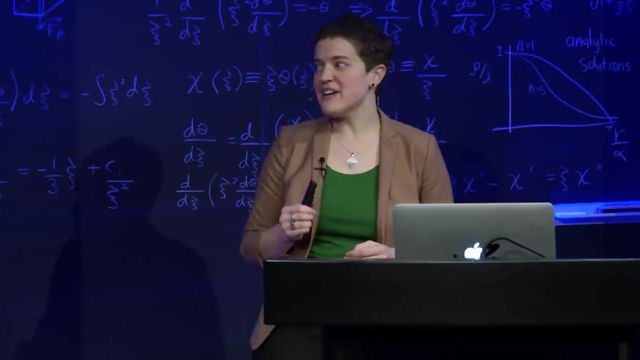 Because of this, we love to call our object a candidate. Extraordinary claims require extraordinary evidence. We have three little bites out of a spectrum that got bigger. It's extraordinary in its own right. These are very difficult measurements to make and it fits perfectly with the predictions of theory. 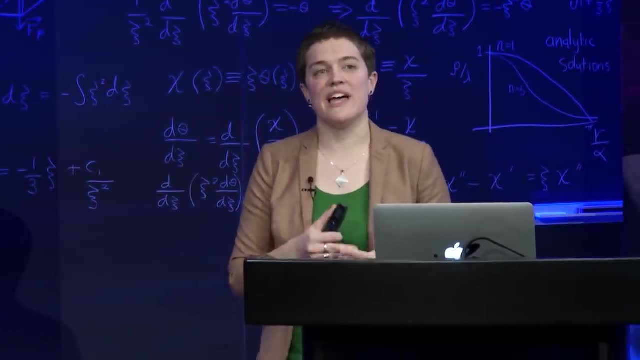 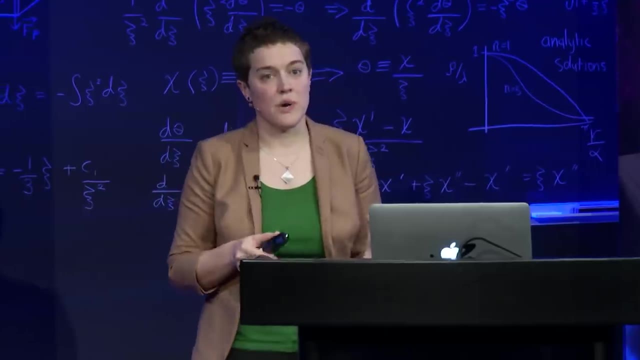 But we're very eager to get more observations of this star, to try and find others like it and to really try and piece together a more complete understanding of how something like a Thorne-Jitgov object could work. So I want to wrap up by leaving you. 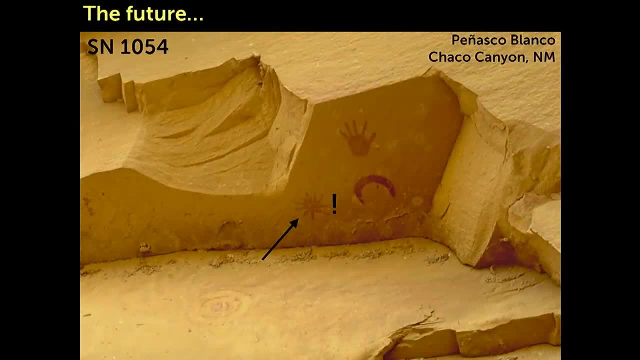 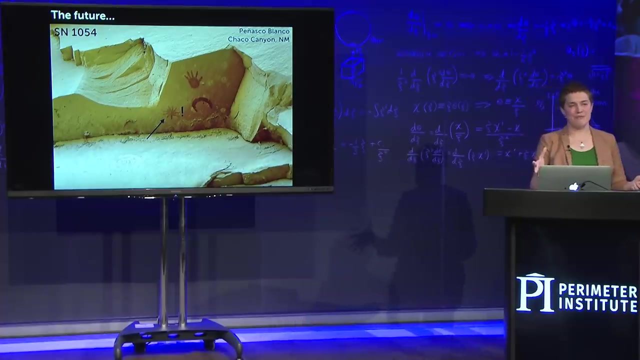 with one last thought. I talked about supernovae tonight. I talked about these exploding stars and how unbelievably bright they are and how we observe them. Nowadays we observe them by seeing those little dots that turn on in other galaxies. These represent violent explosions from massive stars. 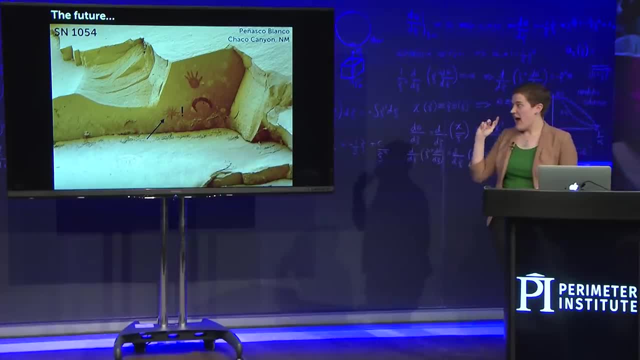 and in other galaxies. that's what we see. I like thinking about this supernova from the year 1054.. This supernova that happened in our own galaxy that was so bright- you could see it in the daytime sky for two weeks- that you could read by it at night. We have last seen a supernova in the Milky Way like this in the year 1604.. Because of how many stars we have in the Milky Way and how often we think they should die, we think we should have seen a supernova like this about once. 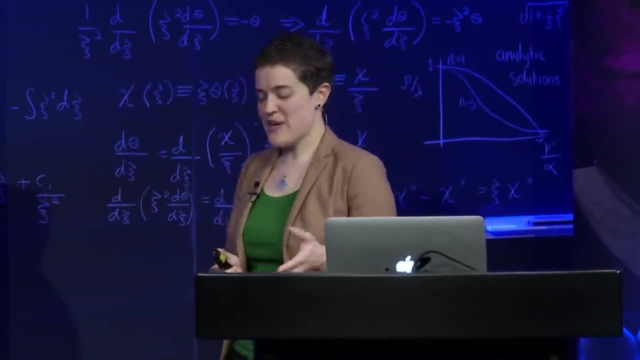 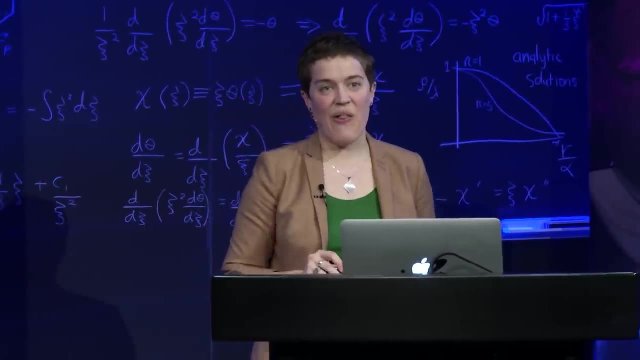 every hundred years. So by that measure we're 300-ish years overdue, And I love imagining what it would look like if we had a galactic supernova right here in our own Milky Way go off tonight, If we walked out of the building and saw this. 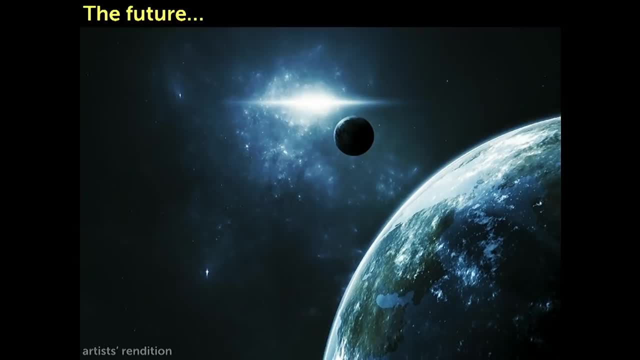 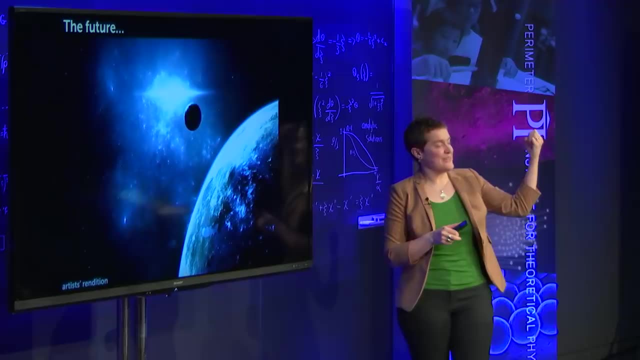 in the night sky. It's a really fun thought experiment to do. I mean, at first it might actually cause a little bit of panic. You're seeing something bright in the sky, slowly getting brighter and brighter. I think, depending on the current geopolitical situation, you might get a little nervous. 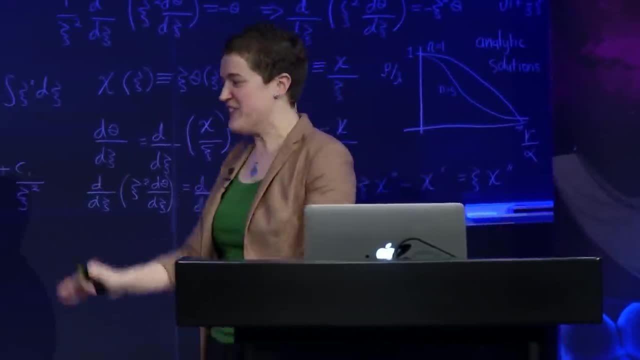 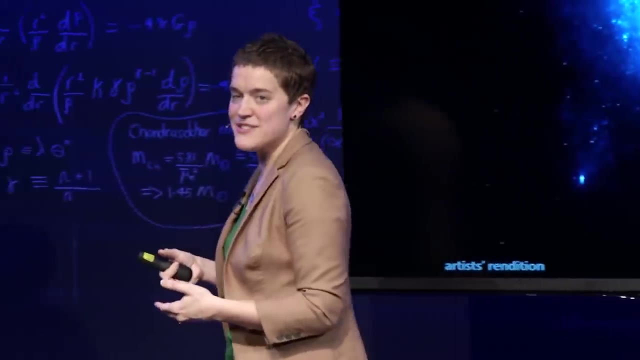 But once we'd established that it was definitely a supernova and nothing else, it would be really interesting. It would immediately get a hashtag. Nighttime hosts on shows would be talking about it. Every cell phone in the hemisphere would probably have a photo of it. 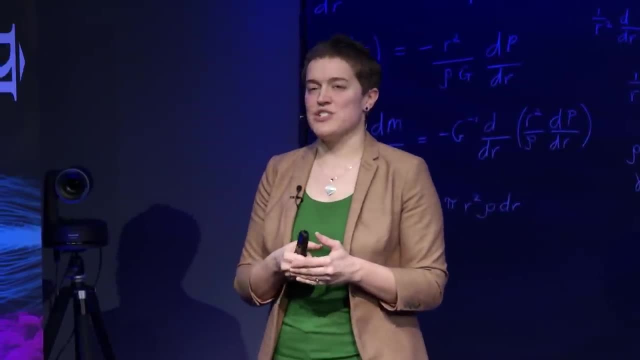 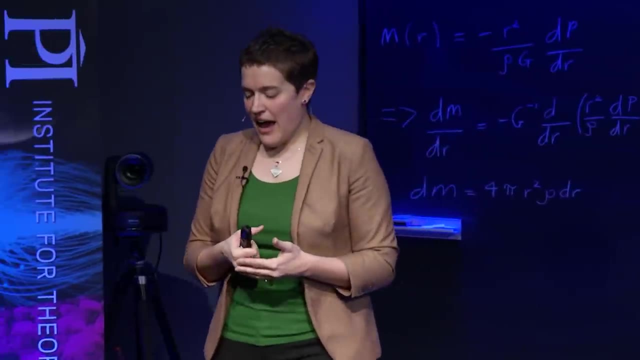 that somebody snapped And I guarantee you that every stellar astronomer would just up and lose their minds, including me. I really hope that we get the chance to see something like this happen. I participated in the eclipse that happened last August And it was a wonderful chance. 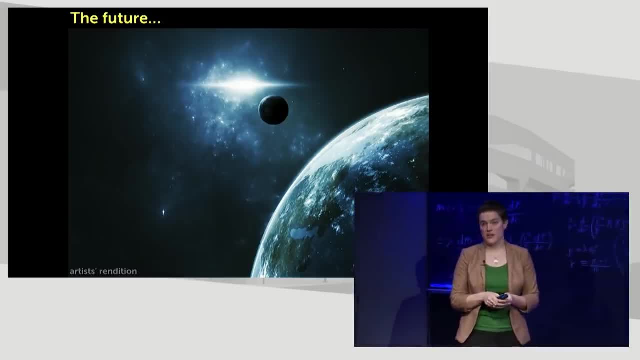 to see people from all over the US and all over the world flock to the path of that eclipse in the pursuit of astronomy And in the pursuit of loving something like astronomy. I think a supernova like this would do something similar: That very bright object appearing in the sky, something. 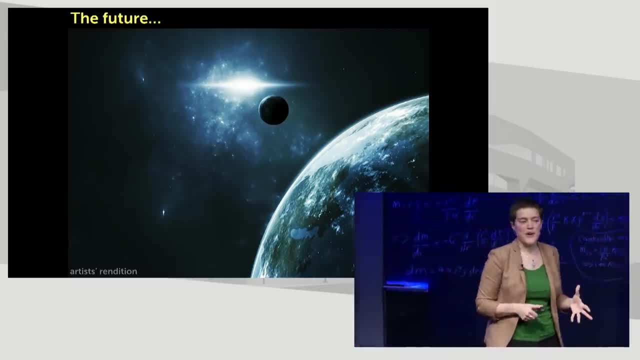 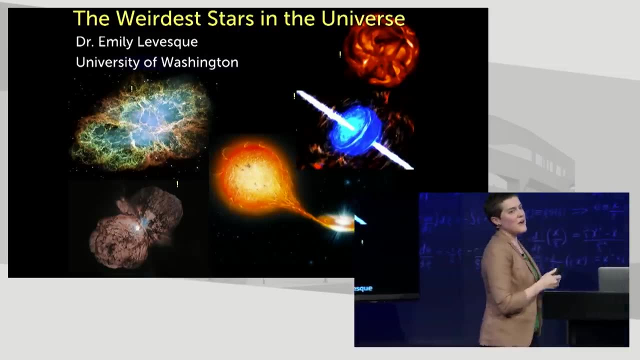 that you couldn't help but notice and something that you couldn't help but get curious about, would be a really interesting thing to study, And, oh my god, the data we get will be amazing. So, on that note, I'll go back to the slide. 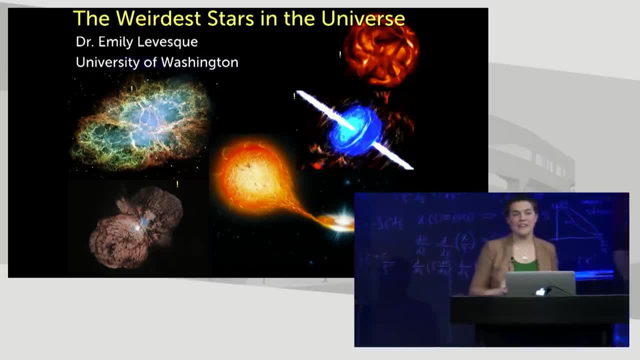 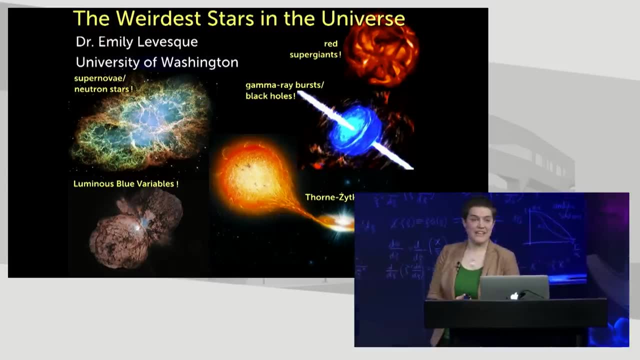 that I had up at the very start of the talk. Remember, I promised you that you could name everything on this slide And now you can. And on that note I will say thank you so much for being here tonight, And I'm happy. 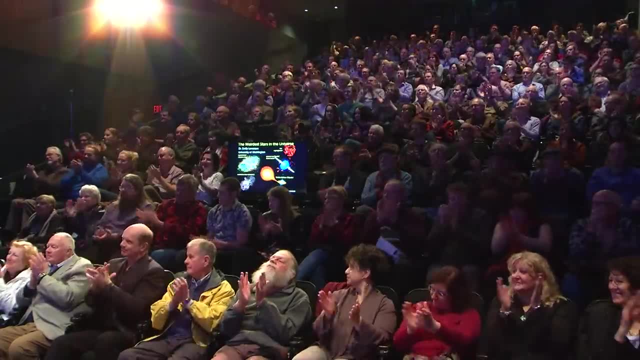 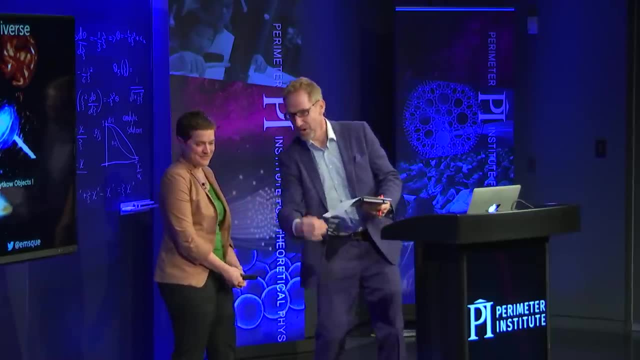 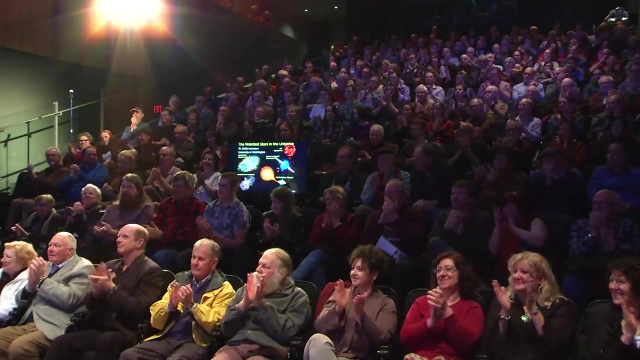 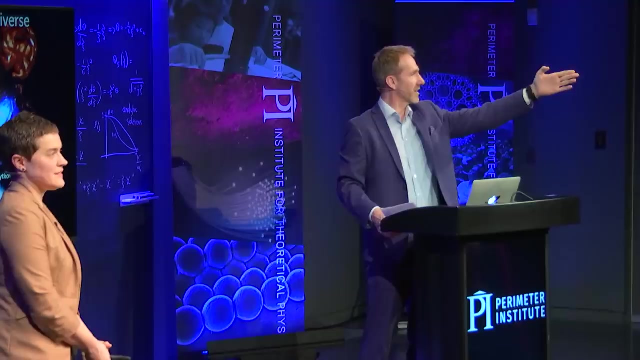 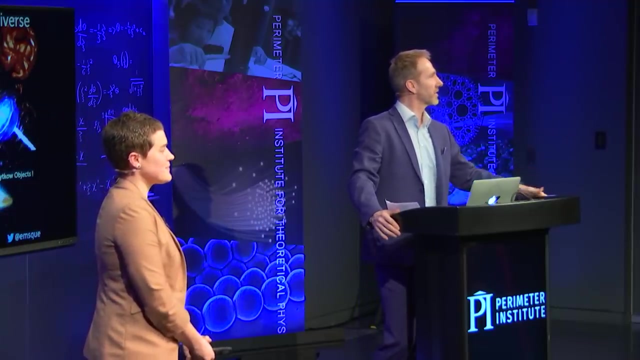 to answer any of your questions. Thank you. applause, applause, applause, applause, applause, applause, applause. So let's open the floor to questions. There's a microphone right there. If you have any questions, just form a queue behind it. And well, let's go to a question in the theater. 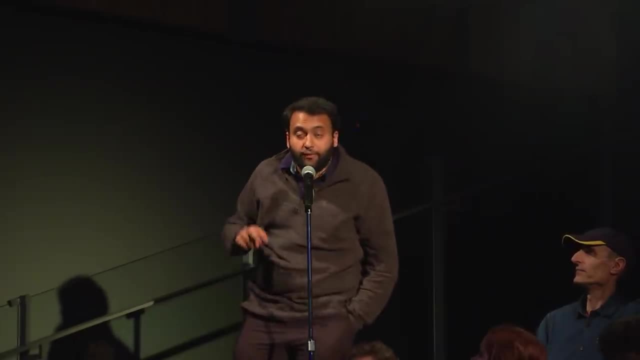 right off the bat, Away you go. Great presentation. I actually have two questions, if that's okay, Absolutely. The first one is: I was curious about the gamma-ray burst sort of forms that you have online. I was wondering: do you guys share? 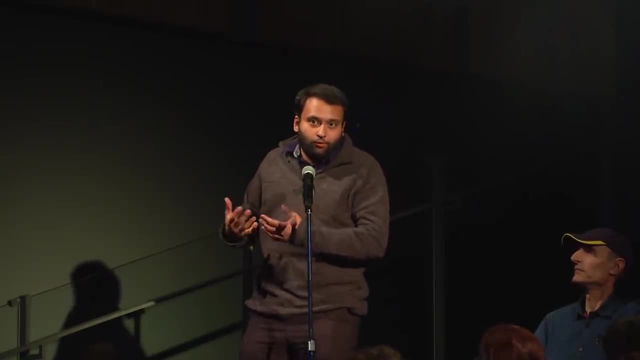 the raw data in order to get the meta-analysis. In the medicine world we've been kind of forced to do that. So I'm curious if you guys are doing that. You know what. It sometimes depends on the type of data or the type of group. 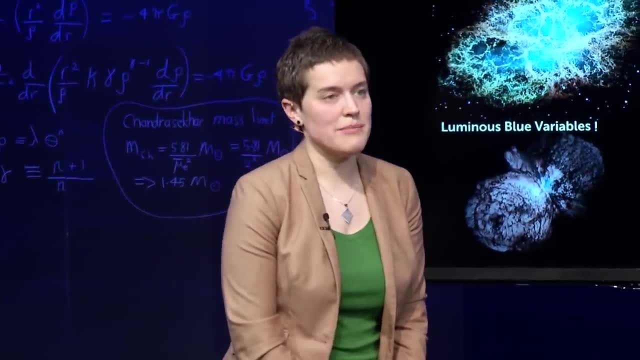 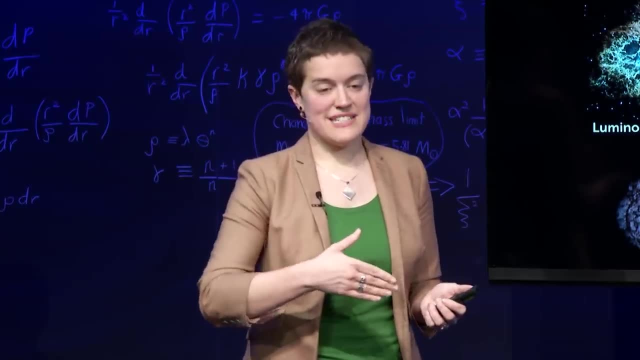 We will usually post results So somebody will take the data and very quickly look and try to determine, for example, how far away it is, And then write a post saying: here's this object, It's at this distance. Sometimes you'll have a couple groups, sort of racing to be. 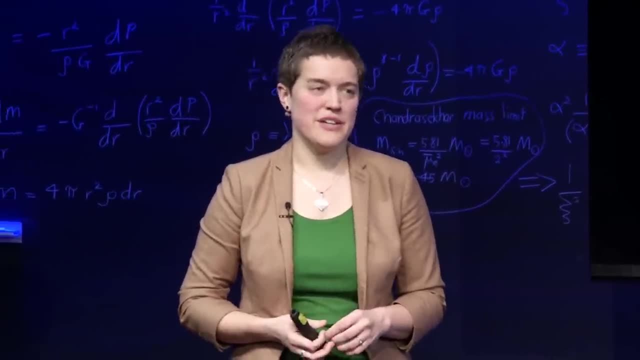 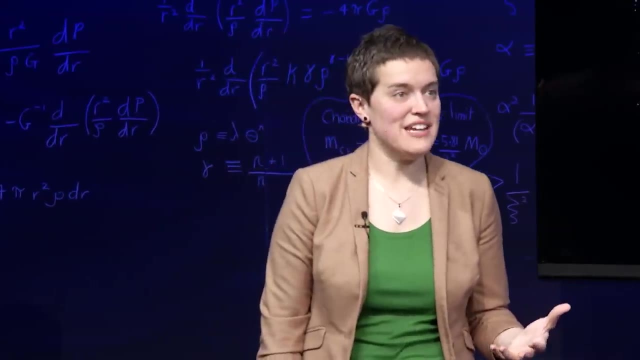 first. But generally if you email someone and you say, hey, I'm curious about this data, they'll either send you the data or they'll send you their analysis of it. So there's very much an encouragement toward collaboration. It just sometimes happens. 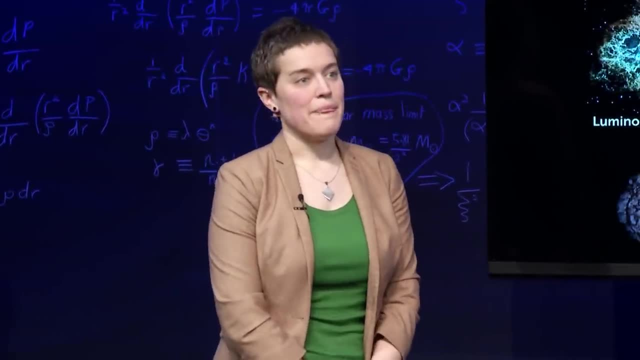 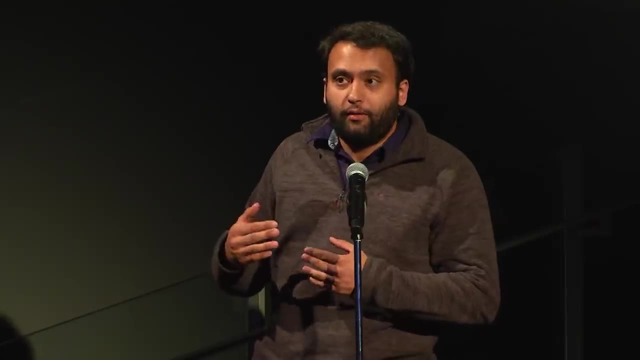 organically rather than as a default when the data come. Fair enough. The second question is actually has to do with the gravitational waves and the fact that the one that you guys found, you guys got to observe the light as well as the gravity at the same. 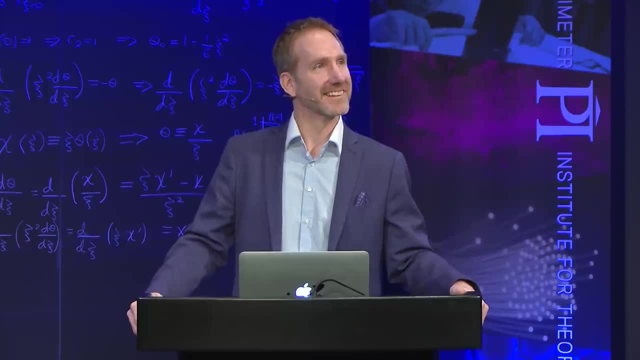 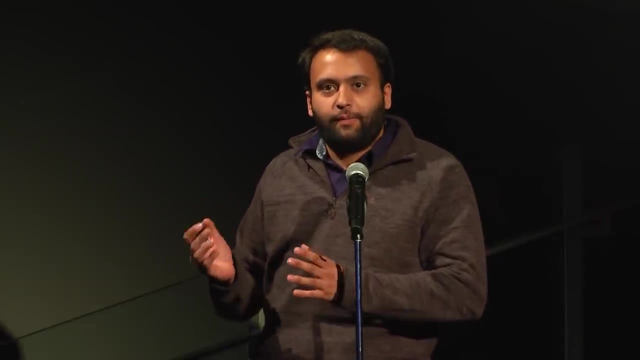 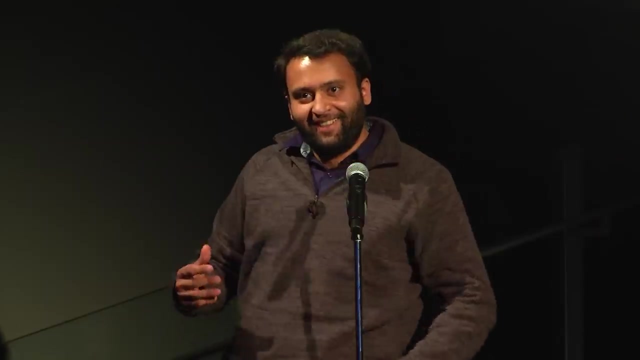 time. So I'm not a physicist, so I'm just curious which one would be faster, Because technically, light goes through space-time, but gravity is space-time. So This is a fantastic question. So it sort of has a two-part answer, in terms of which 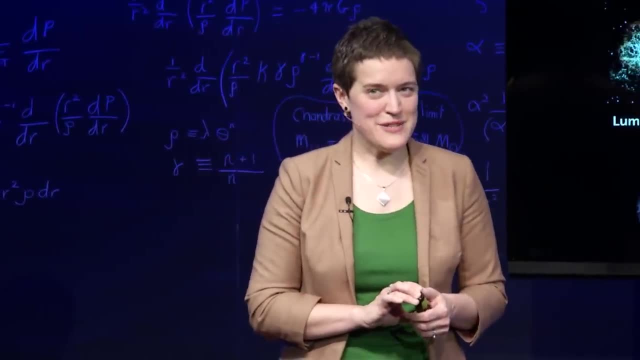 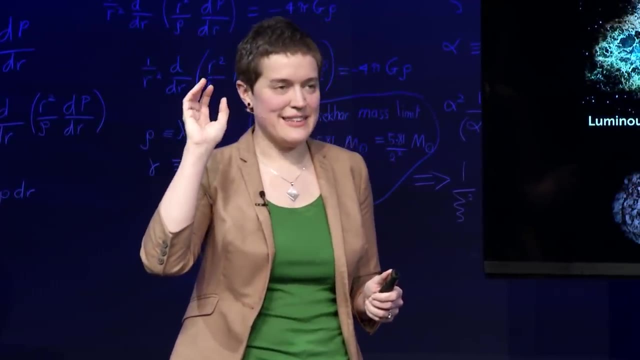 is faster. They're both traveling at the speed of light And for something like this, it sort of helps to. I have a couple colleagues who are experts in this, but the way that I like to think of it is that the speed of light is almost. a property of space-time. It's built in. It's not an extra speed limit that things have. It's actually part of our model of how space-time works. So both light and gravitational waves will travel at the speed of light. Now we'll detect the gravitational waves. 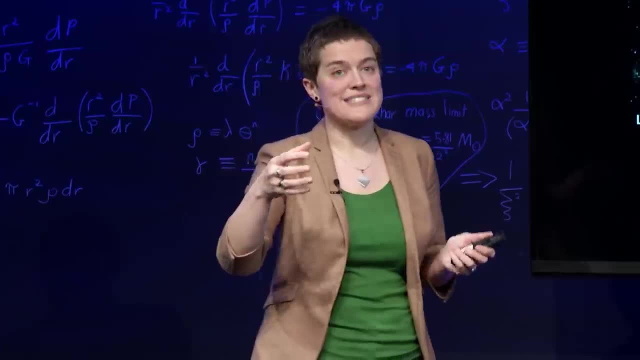 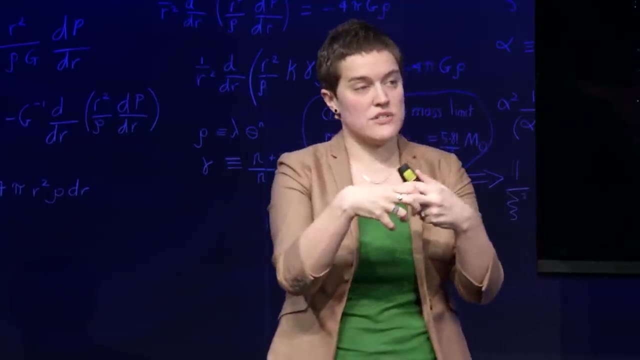 first, with the light following it, Not because they're moving faster, but because that's the order in which the signals are produced. That gravitational wave signal happens first as part of the gravitational disruption of the two neutron stars colliding, And then the flashes that happen after the gamma. 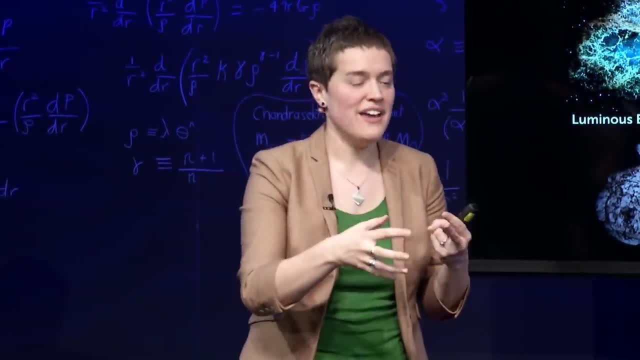 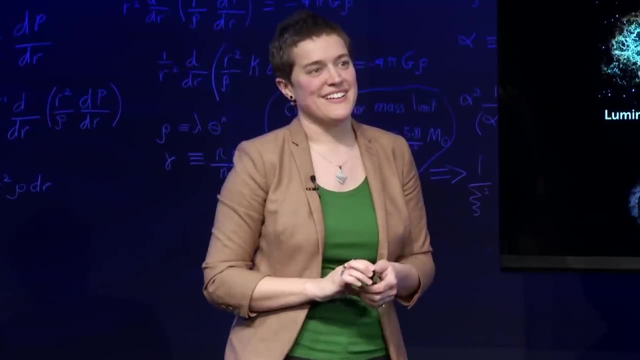 rays and other light that comes later- something called a kilonova- and emission of other light will happen a little later, because it's literally happening later in the event, not because it was just too slow, Fair enough. So warp drives are possible then, right? 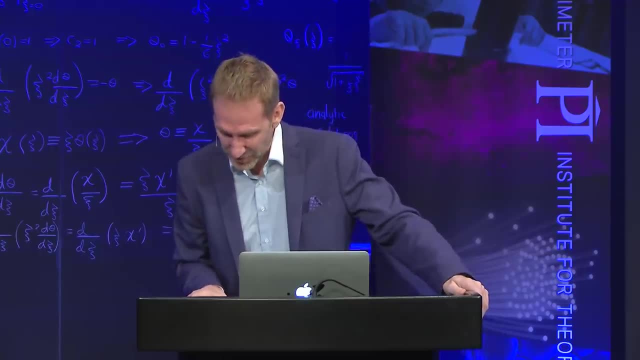 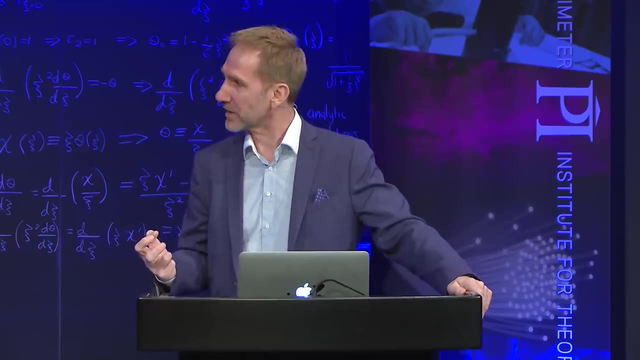 Very good. Let's take an online question. In the Thorin-Zittkow objects: what happens to the original core of the giant when it's replaced by a neutron star? This is a fantastic question and it's a question we, first of all, don't have a. 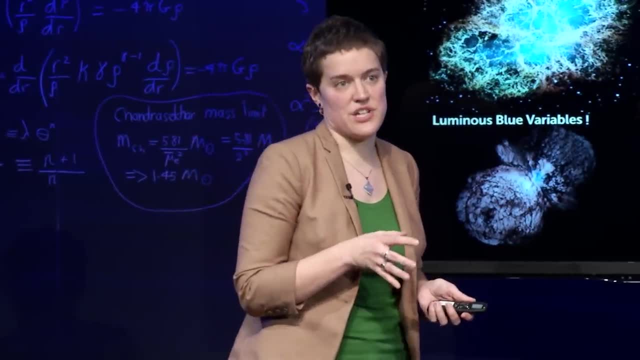 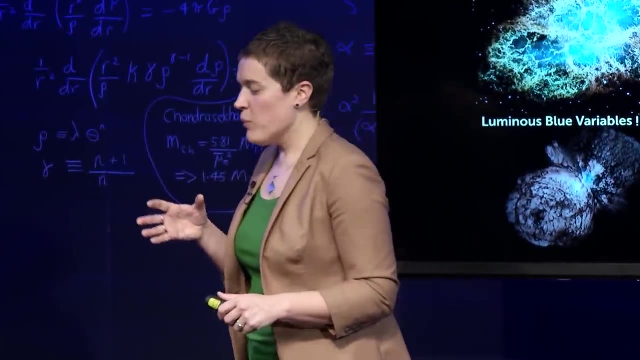 definitive answer to. We're just starting to study Thorin-Zittkow objects. There was a resurgence of interest after we thought we had found one, so we're still working on trying to model them and how they behave. But what we think happens is that that neutron star will settle into the core of the original star, which is starting out by fusing helium in the core. By disrupting the core itself, we go from fusing helium in the very heart of the star to fusing helium in sort of a shell around. the new core, The actual fusion itself will also be disrupted by being very near the neutron star and by other weird physics that's happening in the core, So that old core, we think, will sort of run out of fuel and peter out. but this is just one of several explanations for 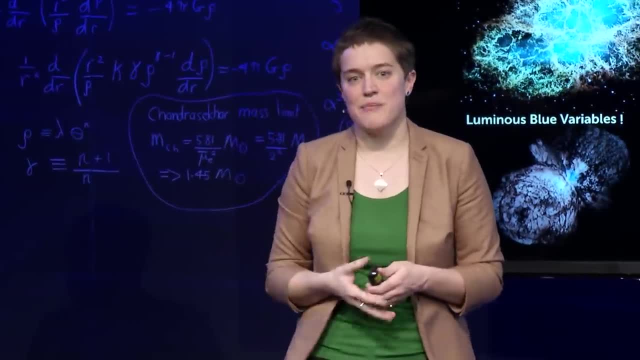 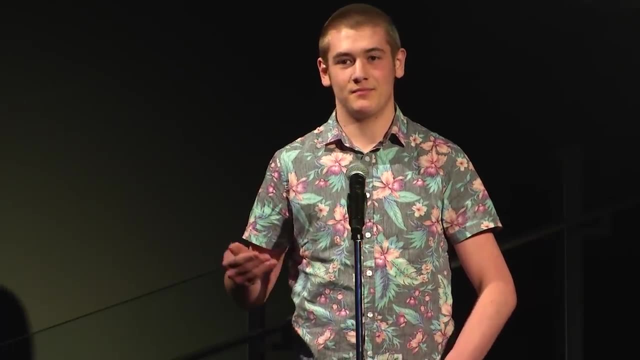 what we think might happen to it, and we're still trying to suss that out from models Excellent In the theater. The one star you talked about, Eta Carina, is a star system. I should say that I have heard of before. 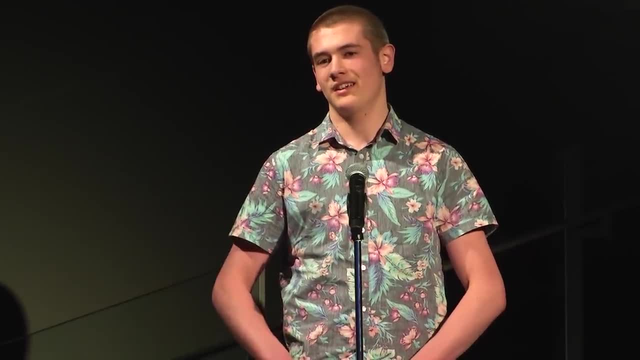 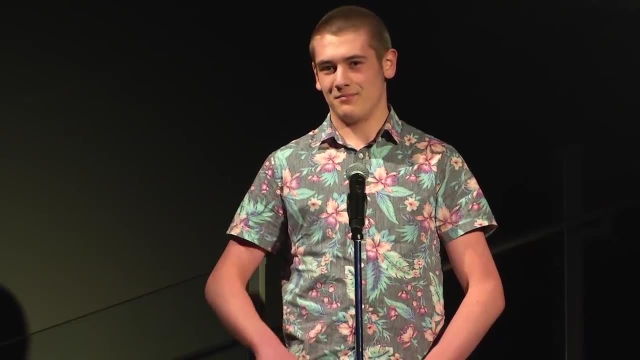 from my online Earth and Space Science class that I'm taking this semester. What I've heard about that star is that when it goes supernova- and it will- its brightness will rival that of the Moon. Is that true, And if so, how long will that last? I think that could absolutely be true. The supernova that happened in 1054 was outshone everything except the Sun and the Moon, so I could certainly see something like Eta Carina behaving that way. You also mentioned an interesting thing that I want to make sure everybody else. 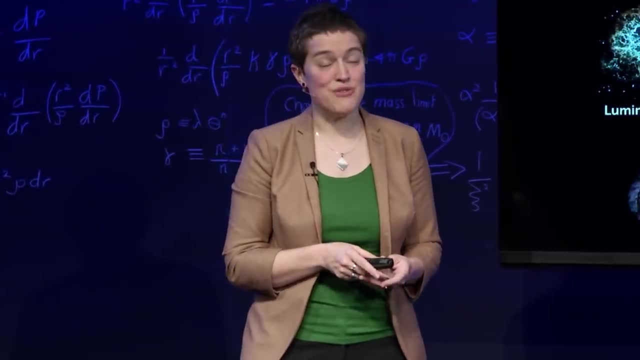 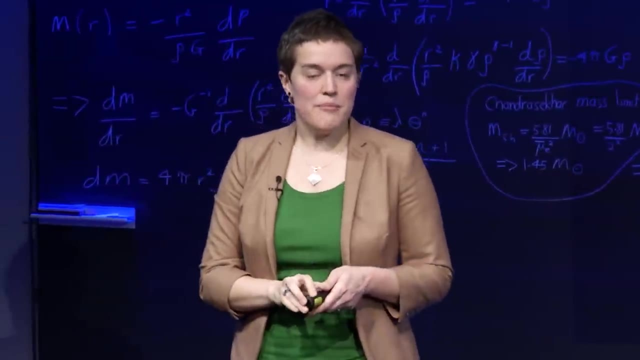 understands, because you were very careful in calling it a star system, And you're right. there are actually two stars buried in there, buried in that picture of the ejected material that we see. Both of those stars are tens of times the mass of our own Sun, and we do think. that a supernova from something like that should be very dramatic and very bright If it gets as bright as the Moon. it's hard to say exactly how long that would last, but it would be on the order of maybe a week or two weeks. 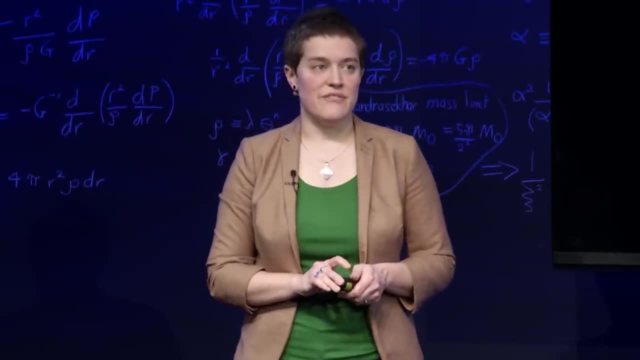 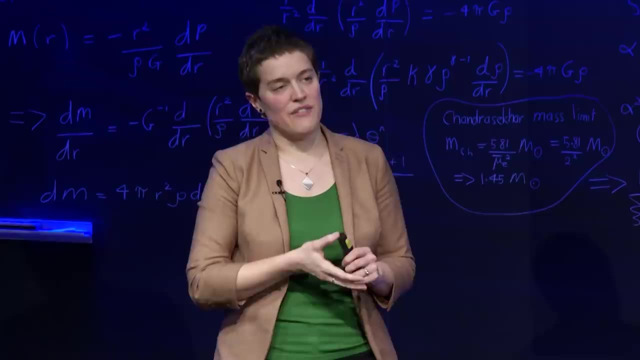 Supernovae will get bright very quickly and then start to fade very quickly, And there's actually a lot we can learn about the star and the chemistry of it by following how the supernova actually fades away. But that really bright period will last a couple weeks. 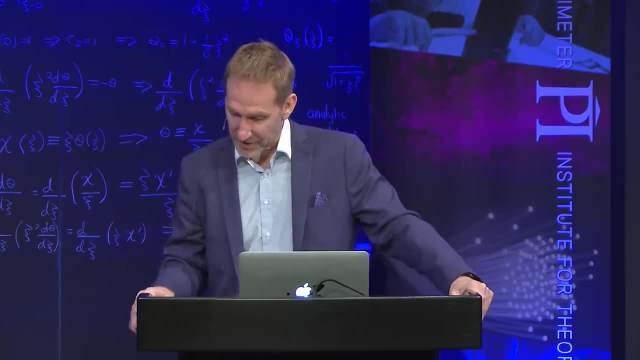 Thank you Good. Here's another online question: Polaris. Polaris is a rare star that won't last that long. Do we know how much longer it might last? It sounds wild that the near, relatively speaking future, the North Star might not be there. 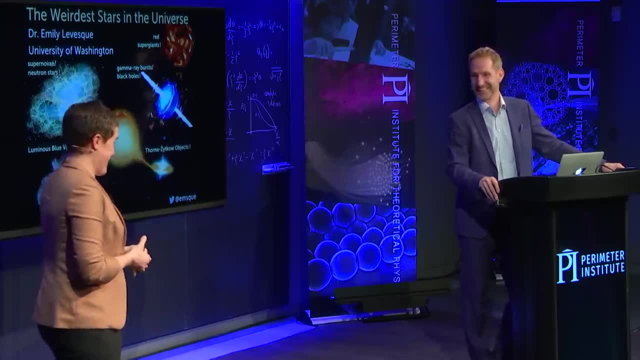 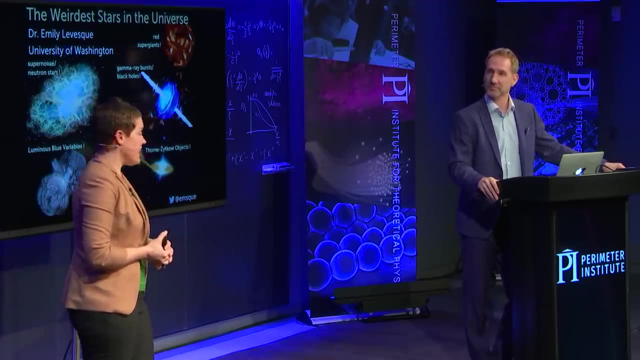 So the good news is that the star will be there for a while. It's just changing evolutionary state And it's hard to actually say where the star is in its evolution Because yellow supergiants are so rare and because it's so. 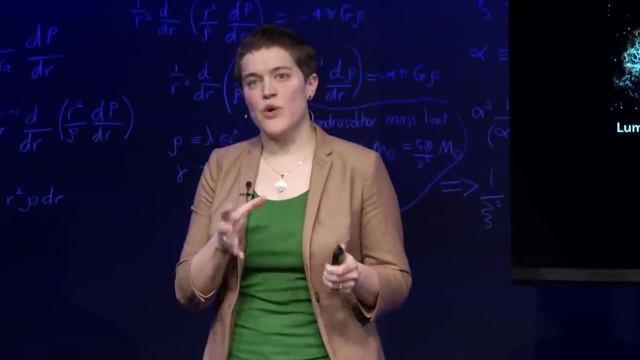 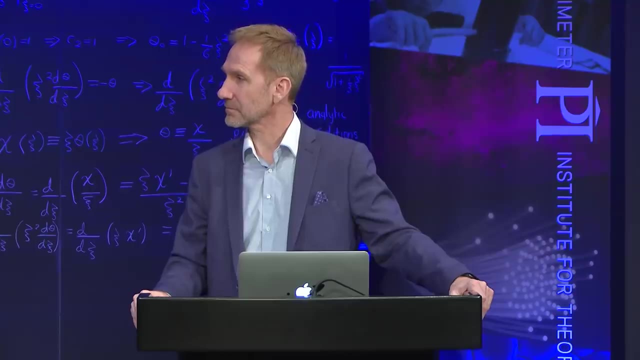 difficult to study them. as a result, we don't have a great formula in place for saying: oh, Polaris is going to last this much longer before it turns into a red supergiant, or it's exactly at this point in its evolution. It would be. 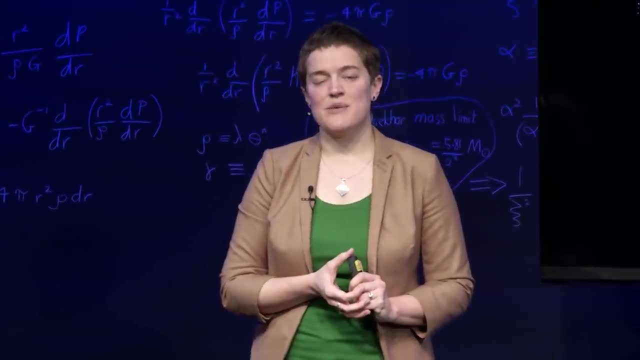 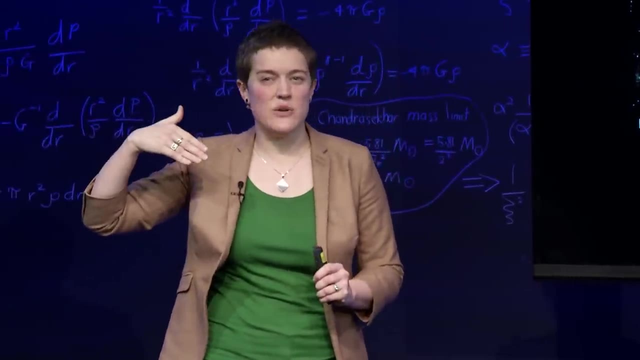 really interesting to find more of these stars. but what's hard is that without knowing the exact distance to a star, it's very easy to confuse something bright and far away, like a yellow supergiant across our galaxy, with something dim but nearby. 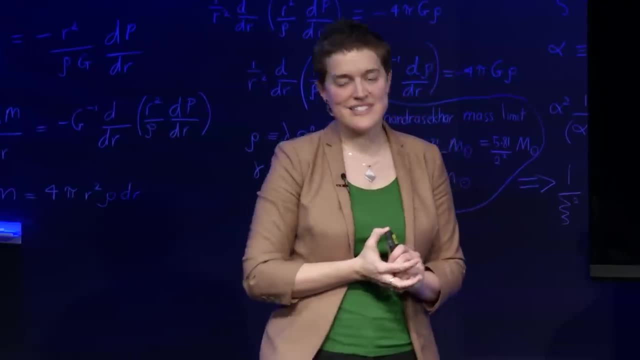 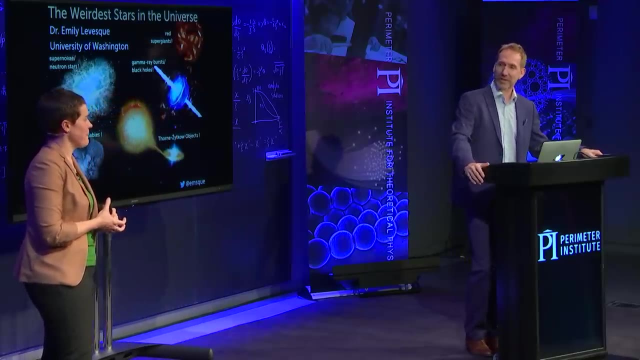 like a star, like our sun, a yellow dwarf. So we're trying to study more of these and we'd love to be able to eventually answer that question, but we don't know yet. Let's finish with one last question: Your excitement, passion. 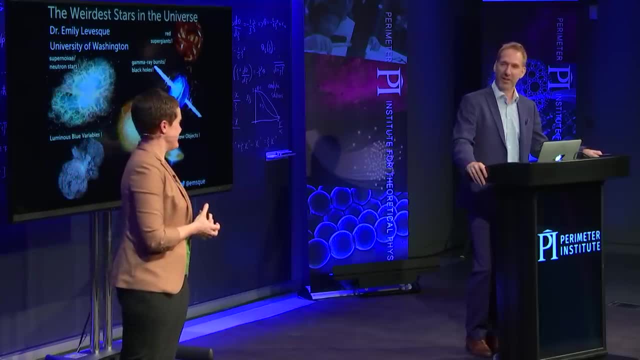 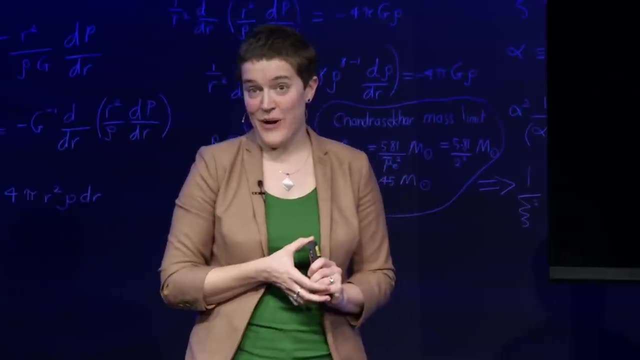 for astronomy is infectious. When did you know that you wanted to study the stars? I think I knew I wanted to be an astronomer when I was about two And I remember why. I have a reason. So I was two years old. in 1986, which was the last time that Halley's Comet made a close pass of Earth. I have an older brother, Ben, who was 12 when I was two, and he had a school assignment to observe Halley's Comet. 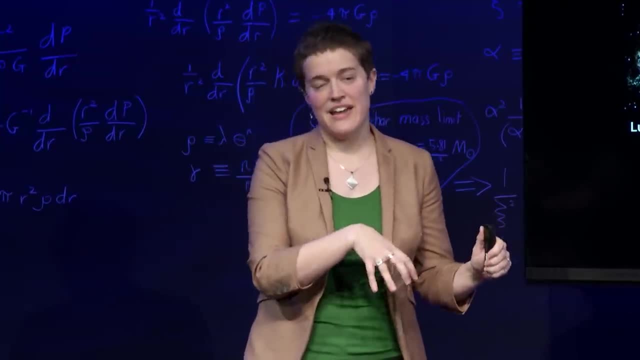 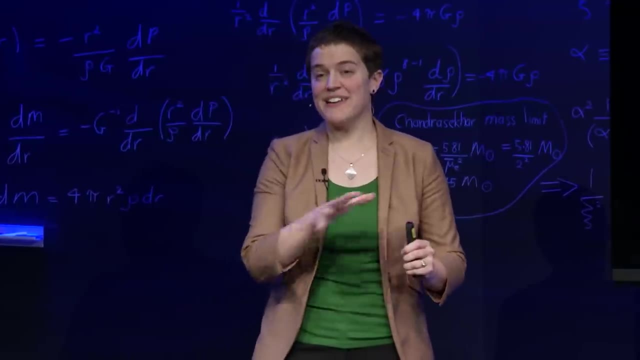 So me and him and my parents all went tromping out into the backyard and I'm sure I was a slightly fussy two-year-old who was a bit bothered by the dark until they sort of pointed me up And apparently I was fascinated and from. 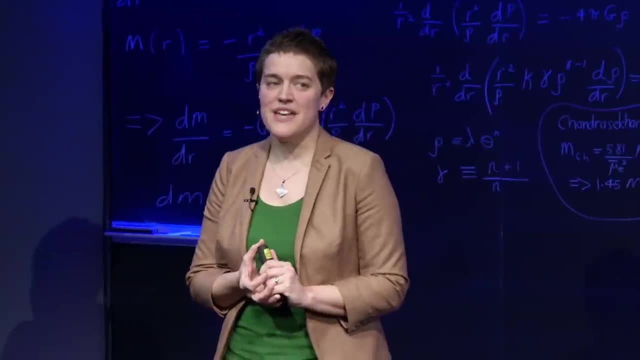 then on. people would ask me what I wanted to be when I grew up, and the answer was always: well, I want to be a ballerina or an astronomer, Or I want to be a firefighter or an astronomer And later on, a marine biologist. 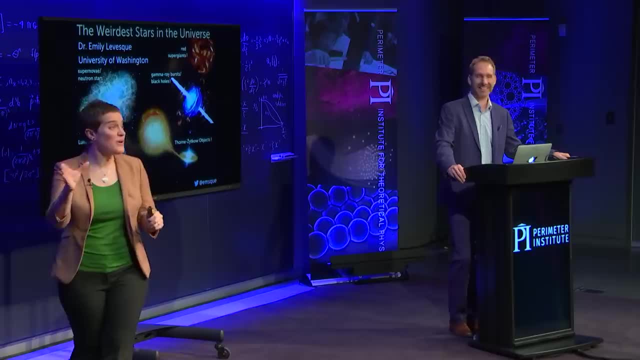 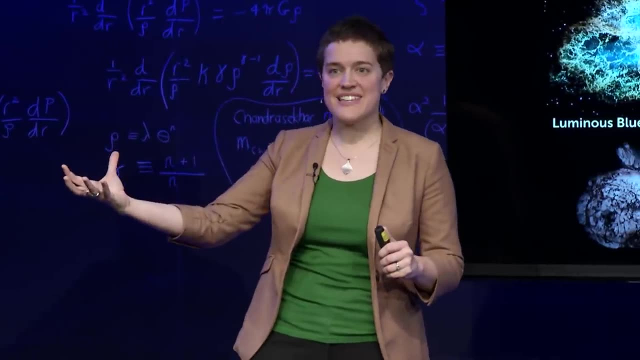 or a paleontologist or an astronomer, But astronomer was always there And astronomer stuck. I read A Wrinkle in Time when I was about eight years old and it just absolutely fascinated me. I was so amazed that we had this protagonist. 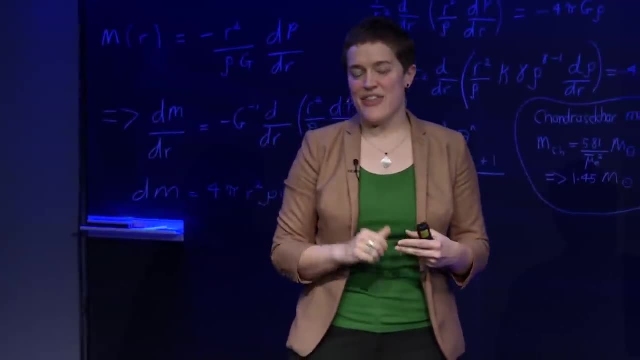 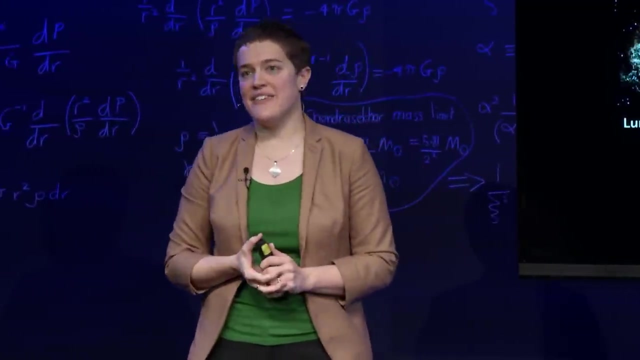 of a little girl who was into physics and into astronomy and that and other books like that and things like science activities in school really helped encourage this in me, And then when I went to college I majored in physics, knowing that that was the